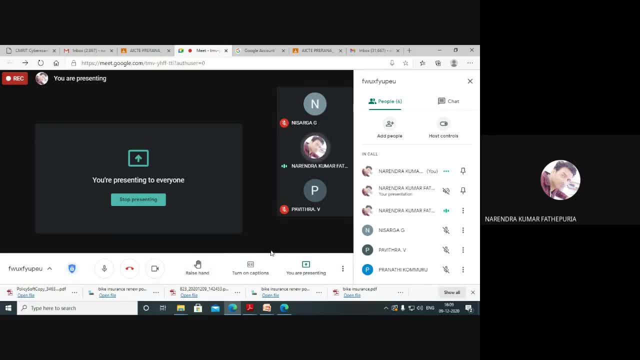 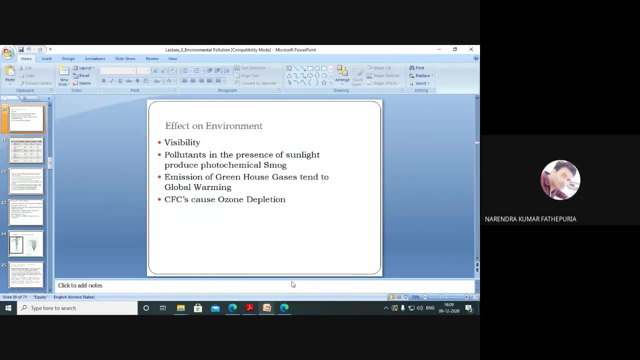 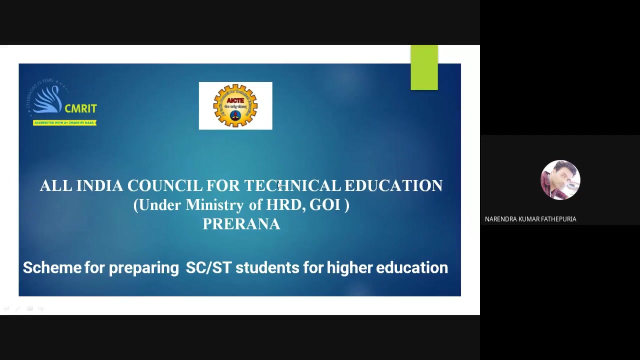 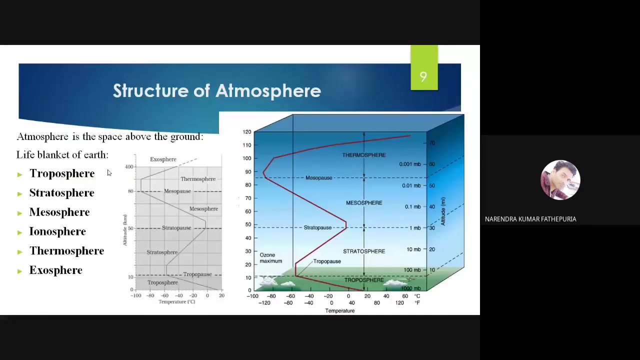 portion for the 8th syllabus. as concerned, Do not leave the class in between. finish at 5.9, which is right now 4.9.. Okay, Yeah, So we were here last time. We were discussing about the air pollution, various pollutants, various impact on human. 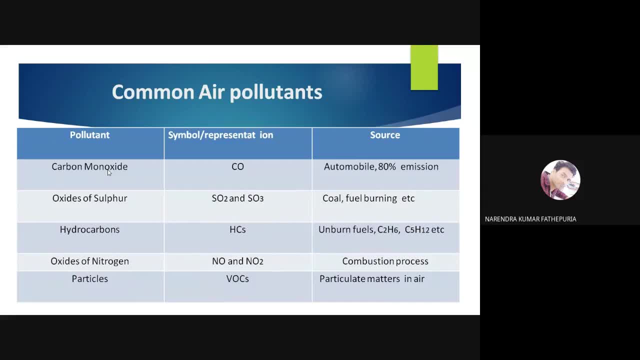 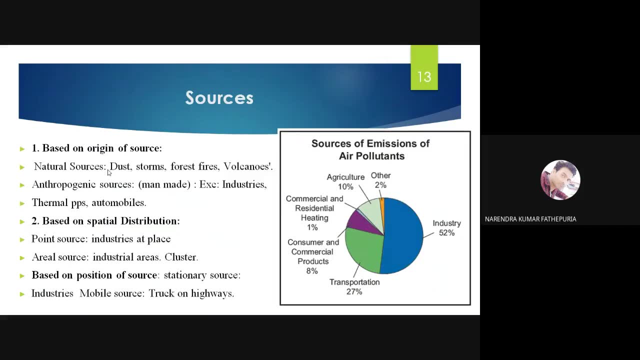 being, as well as the planet, environment and on animals, wild animals and aquatic life. The sources we have. we were discussing last time the various sources of air pollution, The contribution from the various sectors, industries, transportation, transportation studies. we were talking When we were talking about the classification of the air pollutant. 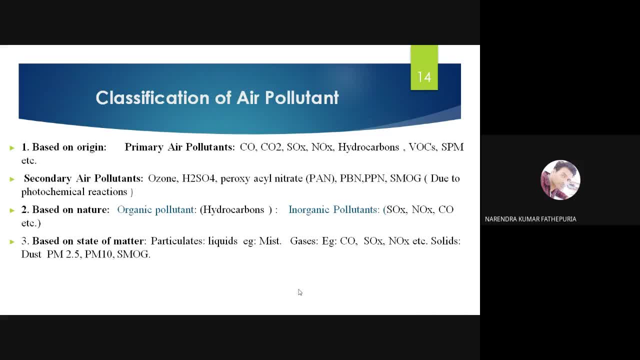 we have primarily or defined in primary air pollutant, as well as the secondary air pollutant Based on the nature. also, we have defined organic pollutant and organic pollutant Based on the state of matter. also, we have defined Particularly matters in liquid forms, solid. 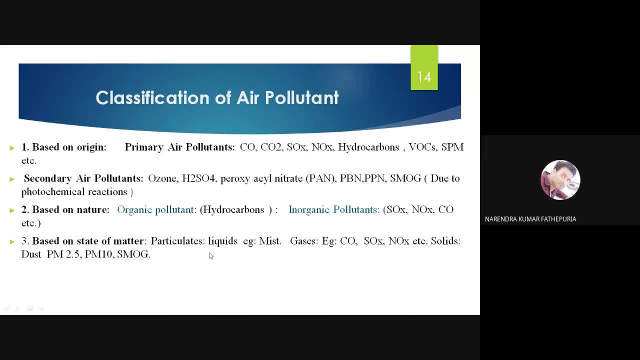 forms and gases forms. Based on this, we have, like in the liquid forms we called as gases forms, the various gases and solids in form of dust, PM2.5, PM10 and smoke is also coming in this state of matter, form. These are the criteria. 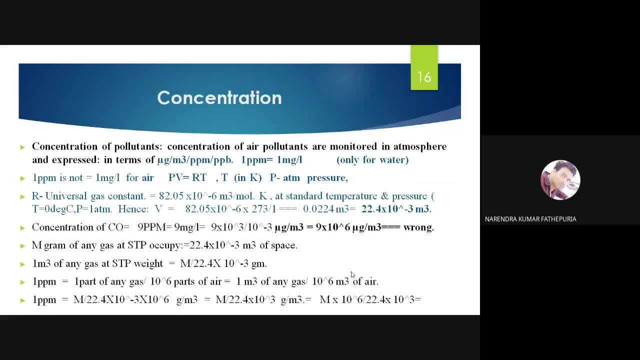 of the pollutant that we have discussed yesterday. Now we were talking about the concentration part last time. All the gases laws will be applicable here, because liquid is different and gas is different. So, like you generally consider, 1 ppm air, 1 mc per liter, will be. 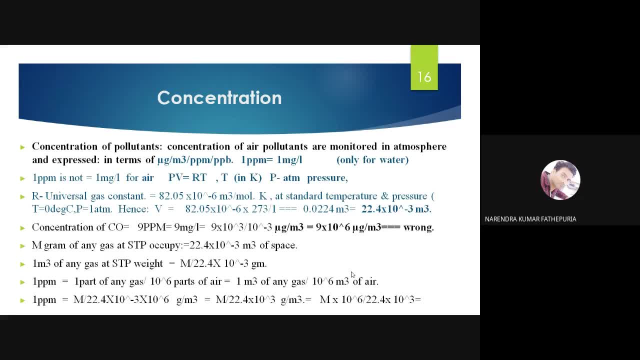 the same meaning, but here it is not like this. not equal to 1 mg per liter for the year. so gases law is valid for it. pv is equal to rt and then if you want to determine the value of concentration, carbon monoxide present in a water. 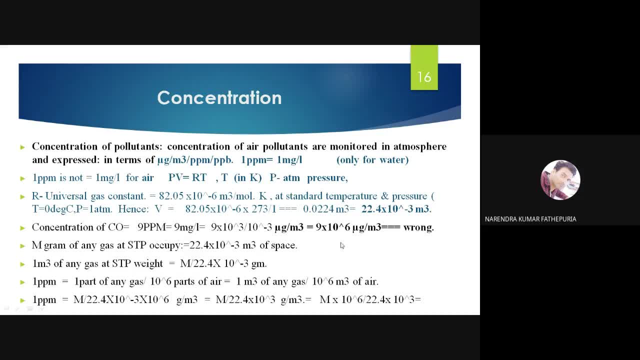 suppose in a one question, given 9 ppm, so 9 mg per liter, if you write it, if you did the wrong calculation, so for that we have to do some conversions so that we have yesterday class. i've explained this thing. and finally, 1 ppm is equal to one part of any gas divided by 10 to. 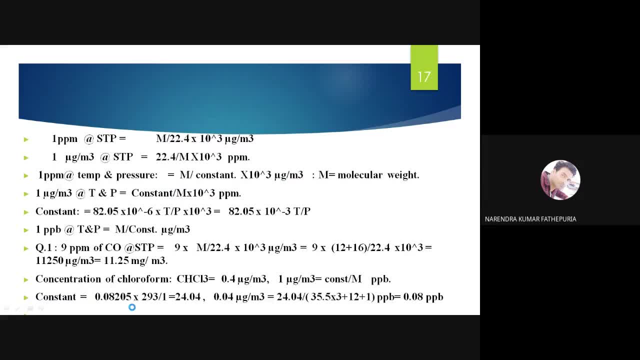 the sixth part of here. and then finally we have uh, yeah, this one. so 1 ppm at the standard temperature and pressure will be equal to uh m divided by 22.4, the molecular weight of the substance divided by 22.4 into 10 to the 3 microgram per cubic meter. so concentration. 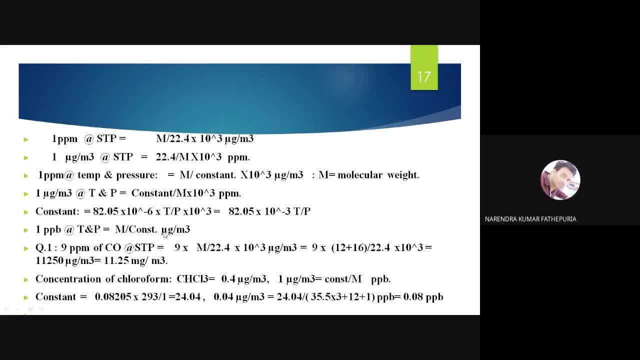 generally of the gases. we are going to measure the microgram per cubic meter only, so we have done this numerical last time, okay, so 9 ppm of carbon monoxide at stp, so there's a 9 ppm means 9 into m, divided by 22.4 into 10 to the 3 microgram per cubic meter. 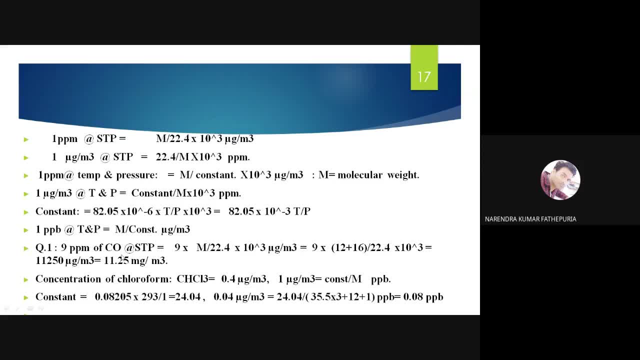 so m will be the molecular weight, so that is 12.6, 12 plus 16, and then if you do the calculation, you will getting it now 11, 250 microgram per cubic meter, so it will be around roughly 11.25 mg per. 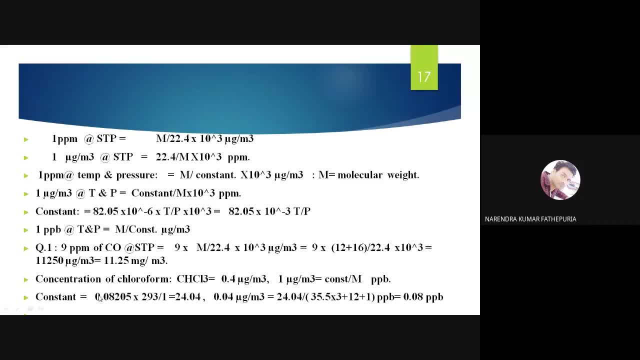 cubic meter. so like this is the same thing you can do the concentration of chlorine, phclp. so this is given in the reverse manner. also you can do in that way. so if the concentration is given in one, in the microgram per cubic meter, then you will get in ppm also by using this relation. so here: 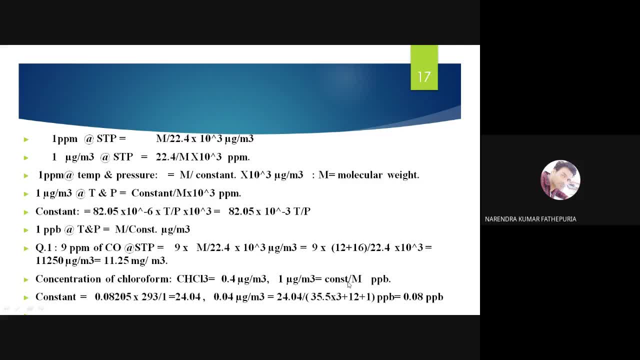 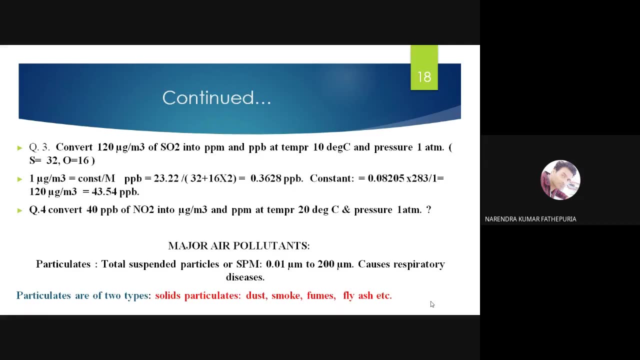 it is a reverse. so one microgram per cubic meter is equal to constant divided by m into ppv, a ppm that's called. this can do the final solution that like 120 microgram per cubic meter of s2p into ppm and ppb at temperature. 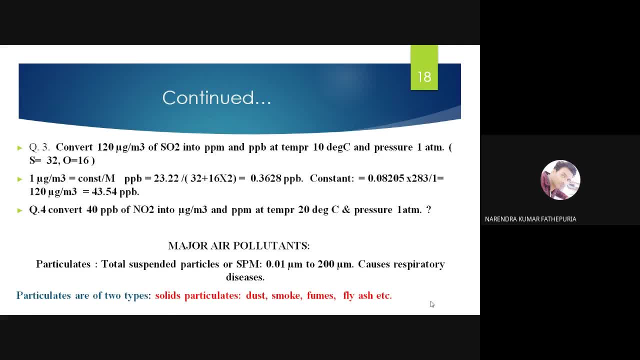 10 degrees celsius. the pressure is one atmosphere. we have to convert it. so this is the formula that we have just now discussed: one microgram for a cubic meter is still constant divided by m. so like this you can do the respective conversion. small, small questions they may ask in a question. 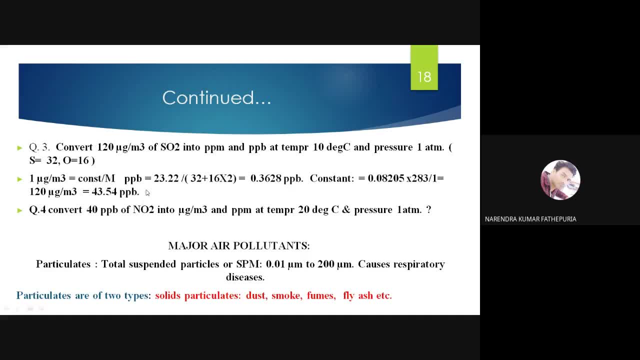 from the gate point of view. so these things, one or two marks or one mark station, so same, like the, convert particle pv of tornadoes and dioxide into microgram per cubic meter and ppm at temperature, 20 degrees celsius and pressure, one atmosphere. these are the things that you can do it. so the major air pollutants like these, are particulate. 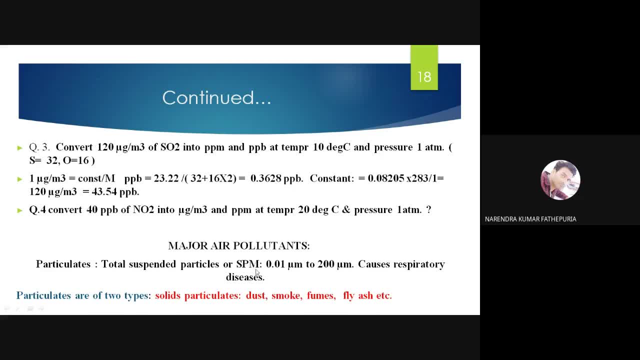 matters which claim control the total suspended particles um. the size of suspended particulate matter is 0.01 micrometer to 200 micrometer. it causes the respiratory diseases. so there are the particulate matter called as respiratory or suspended particulate matter, rspn, so it's 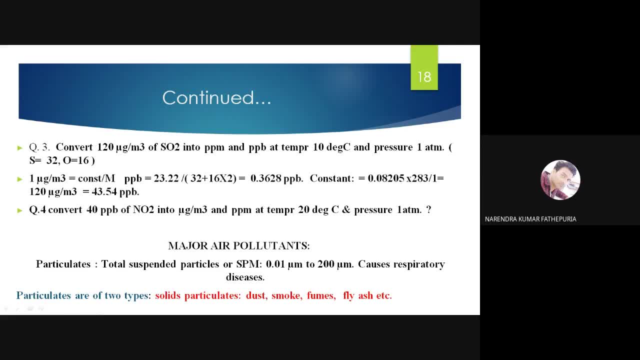 like. it's not visible, very less, and micron is very less size. you cannot see from human eyes, but it can easily disperse into into the air. it can while you are breathing it. these particles can- particular matters can- easily or inhale and then it creates a lot of problems for the lungs as well as for the 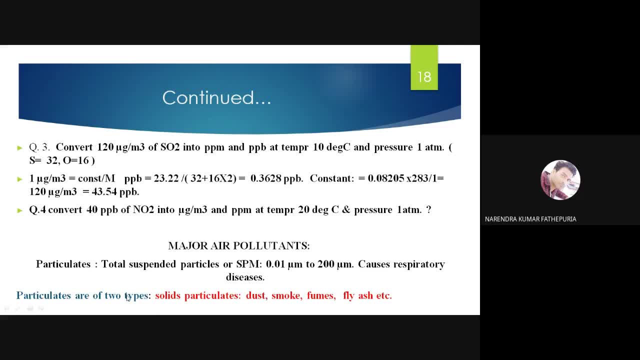 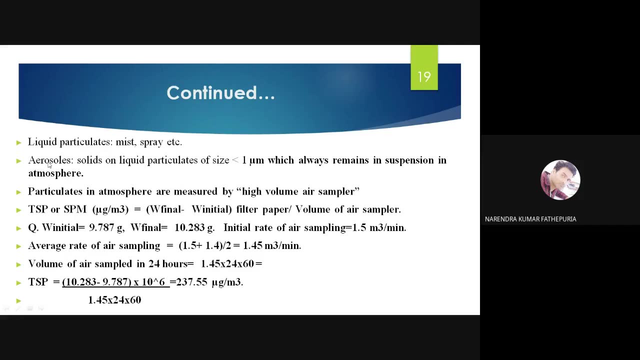 respiratory tract damage. so particulates are the are of mainly two types. there's a solid particulates like dust, smoke, fumes, flyers will be coming in the solid particulates. there's a liquid particulates which will be having mixed in spray. there are some aerosols, also solids on liquid particulates for particulates of size less than one micrometer. 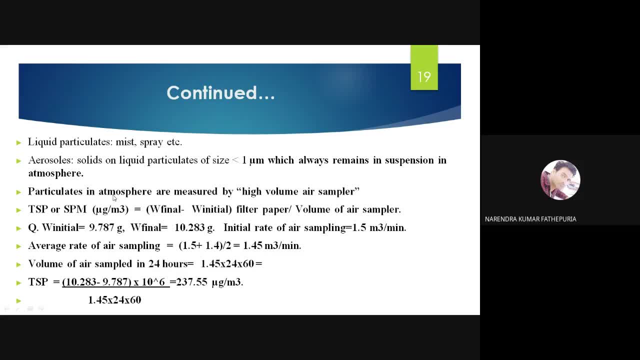 which always remain in suspension in the atmosphere. the particulates in atmosphere are measured by high volume samplers, so high volume air samplers are required for measuring concentrations. so while they are going for the measurement of the pollution, there are the various devices that you have to use it for it. there's a total suspended solid source in the particulate. 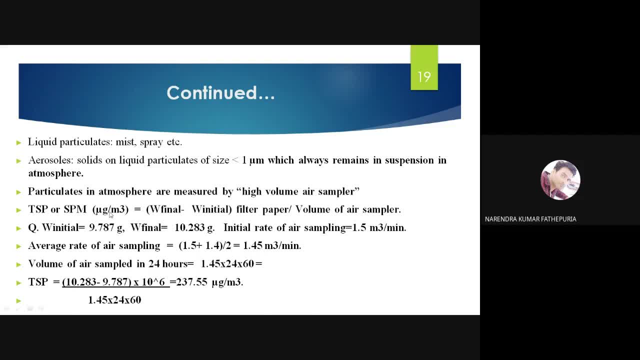 matters, yeah, in the particulate matter, that you generally measure in microgram per cubic meter. so if you have a, if you have a high volume air sensor, so initial volume, you have to note it down for the filter paper, and then final volume after the accumulation, yeah, after the 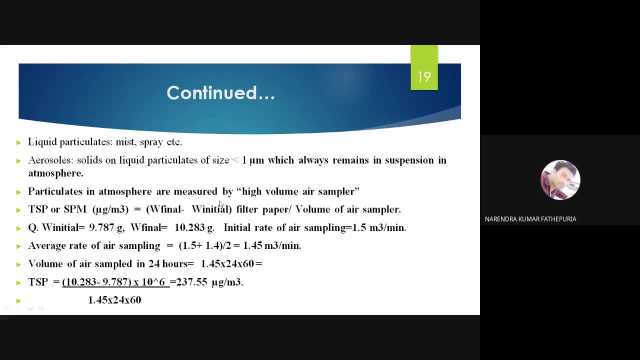 clogging of the suspended particulate matter on the filter paper, weight difference will be there. so final weight minus initial weight of the filter paper divided by the volume of the air sampler, so you will get that the complete- uh like- volume of suspended particulate matter in microgram per. 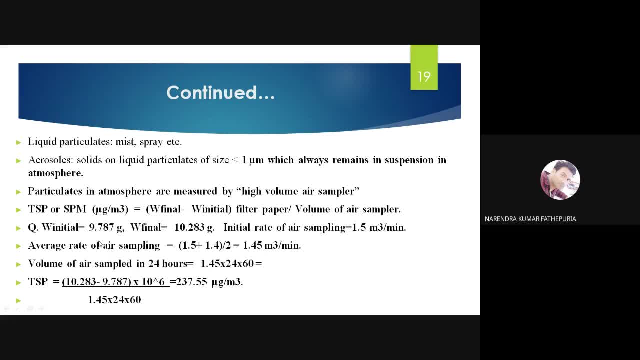 cubic meter. so like this: suppose the initial weight of filter paper is nine to seven, eight, uh seven gram is given. the final weight is after putting a volume sampler for for a certain time, and ten point two, eight or three gram vinyl. so initial rate of air sampling is given as 1.5 meter cube per minute. 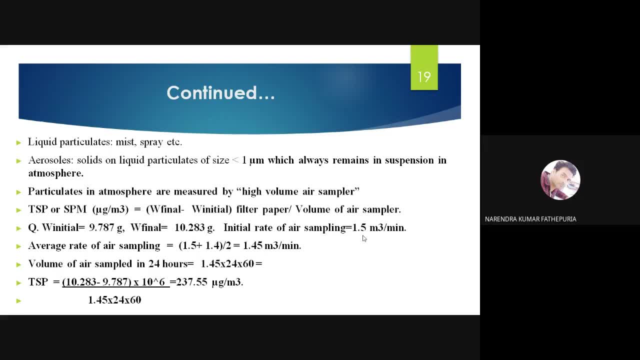 initial rate of air sampling, which is 1.5 cubic meter per minute. every minute that air sampler is taking a 1.5 cubic meter of air average rate of air sampling you can determine through this: there's a 1.5 plus 1.5. 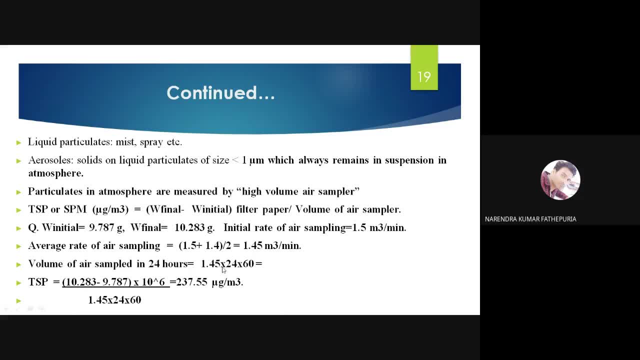 4 divided by 2, 1.45 meter cube per minute as the initial rate, and final rate is given as 1.4 cubic meter per minute. so the average, you can take it. and volume of air sampled in 24 hours: 1.45 into 24, into 60. you will get it in a minute: 1.44. total volume of the air sample. you can get it. 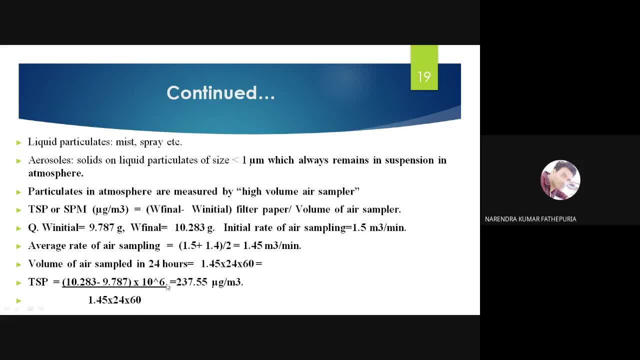 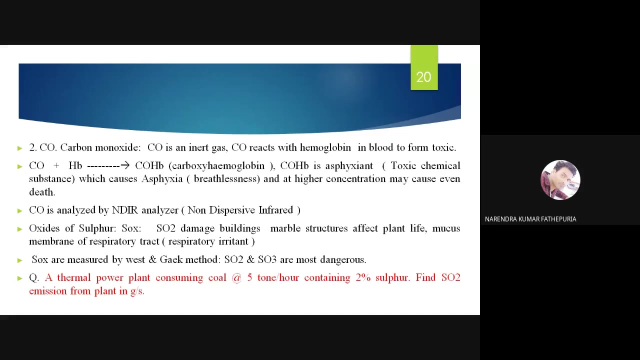 now tsp, you will get it here. so this final minus here you are able to dzi. if you multiply by the paper here, the volume of the air sample will be getting a 237.55 microgram per cubic meter. and that way you are going to calculate. 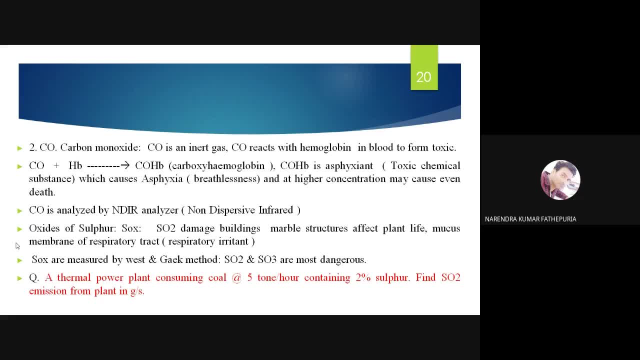 the suspended particulates volume and your rate of suspension. microgram per cubic meters, like this you have to estimated. carbon monoxide reads with the hemoglobin in blood to form toxics. so carbon or dioxide, carbon monoxide plus hemoglobin. it forms the carbo, or hemoglobin, carboxyhemoglobin. 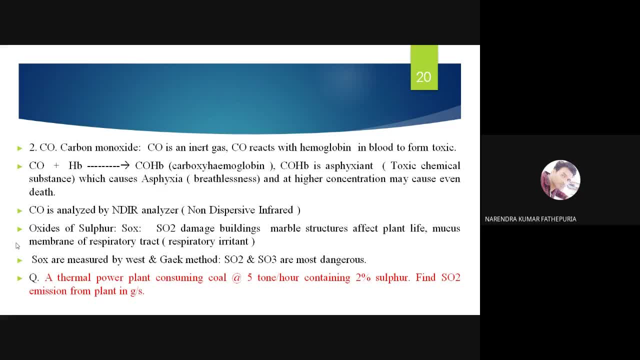 which is um espousian- yeah, we call it toxic chemical. the measurement is important. one by one. we are talking about the measurement impact. we have already discussed in the last class various impacts on the human being, animals and water, animals and the climate, and environmental, and we have studied and various types of pollutants also. 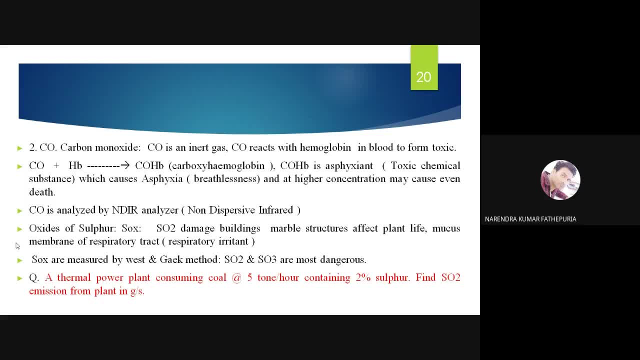 we have discussed in every polluting process. we have discussed in the last class, we have discussed in the last class, we have discussed in the last class and how it is adversely impacting the environment, how it is adversely impacting the environment, how it is that was impacting the human body. that also we have discussed, so i'm not repeating that. okay then, 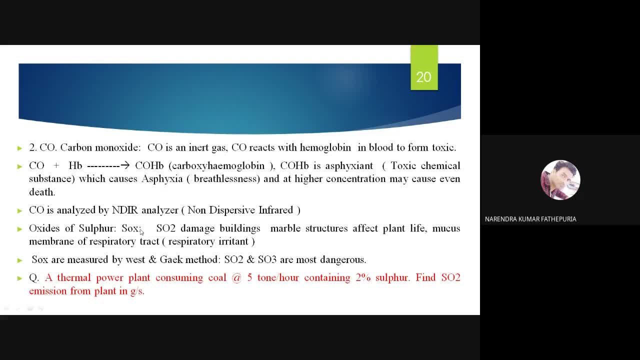 there are oxides of sulfur that are to the same way you can um like the major. the volume and microgram per cubic meter cover 41He. fares for damage. buildings, marble structures affect plant life. nucleus membrane of derasperated tread respectated irritations stress muutų members. meta sharpens uğSTHAB aomanpart over the caller in this example. 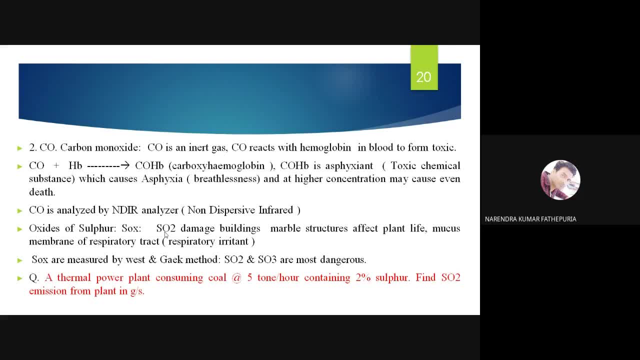 SX are measured by West or the GECK method, SO2 and SO3 are most dangerous. So suppose the equation is: given a thermal power plant containing a coal of five tons per hour containing 2% of sulfur, Find the sulfur dioxide emissions from the plant's gases form. There's a coal thermal power plant, 5 tons coal is. 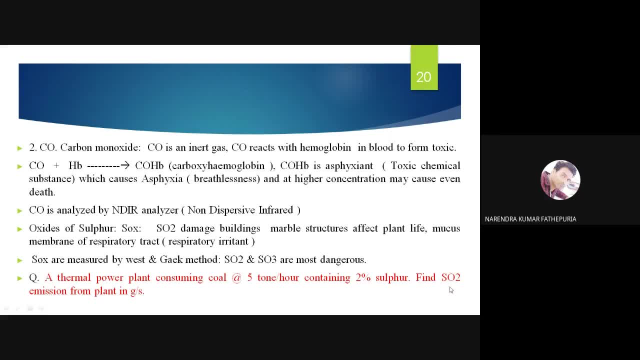 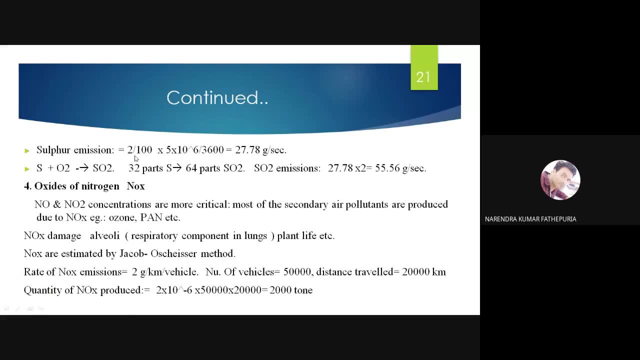 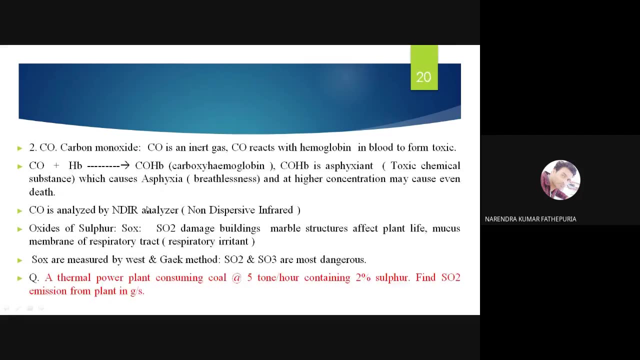 required per hour. It contains 2% sulfur, The sulfur dioxide emissions. you have to measure it, So sulfuric there's a sulfur emissions. you can measure like this: 2% means 2 by 100. Where we have came? Yeah, 2% means 2 by 100 multiplied with. 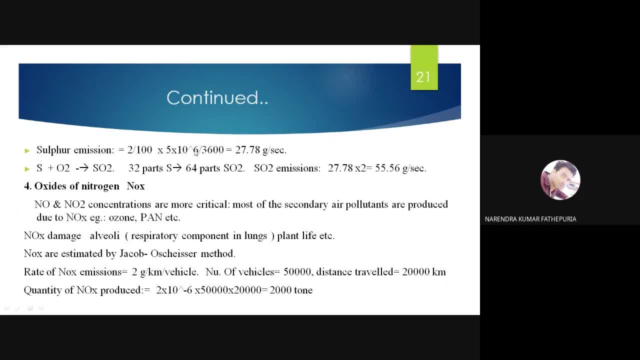 5 tons per hour. it is given So 5 tons, 5 into 10 to the power, 6 divided by 3600.. So you will get it here at 27.78 gram per second. Sulfur emission: total So S plus O2 will be the SO2 and the molecular weight. you. 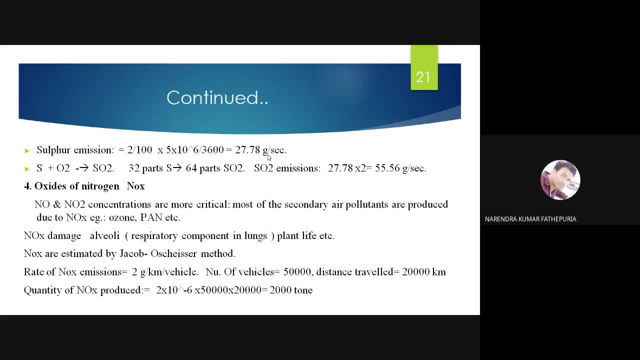 can calculate, There's a 32 parts S, 62 parts SO2.. So SO2 emissions will be 27.78 multiplied with 2. So you will be getting a 55.36 gram per second. This is the emissions which will be released from the thermal power plant. 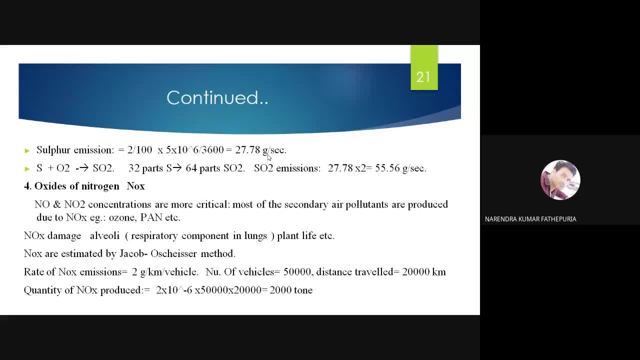 So like this you can measure it. There's the volume sampler. We are going to collect these gases in micrograms per cubic meter. Then NOx: NOx measurement is also necessary. NOx sampler and SX samplers are there. We do have in our laboratory also Volume samplers And analyzers also. NO2 analyzer is also there. 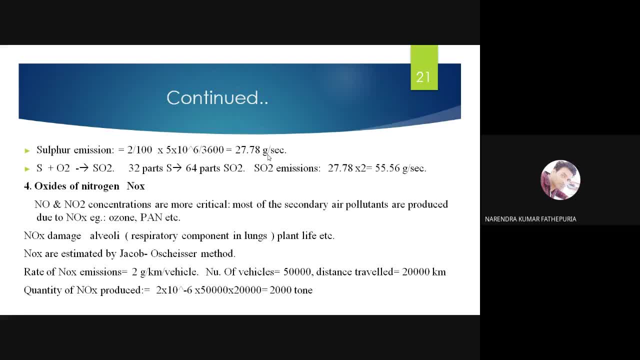 So NOx damage respiratory component in lung plant labs etc. NOx are essential, So NOx is essential. So NOx damage respiratory component in lung plant labs etc. NOx is essential, So NOx is intended. by Jacob Ostiazer method, The rate: 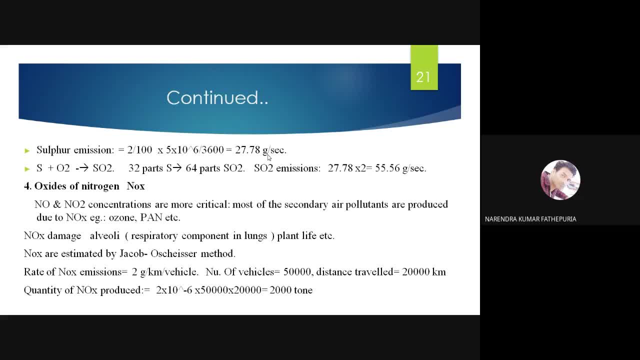 of NOx emissions will be equal to 2 gram子 per kilometer per vehicle. It's a moving vehicle. I have told about the sources of the pollutant: moving sources: fat point sources, Non point sources. The classification of source of pollutants we have discussed in last class. 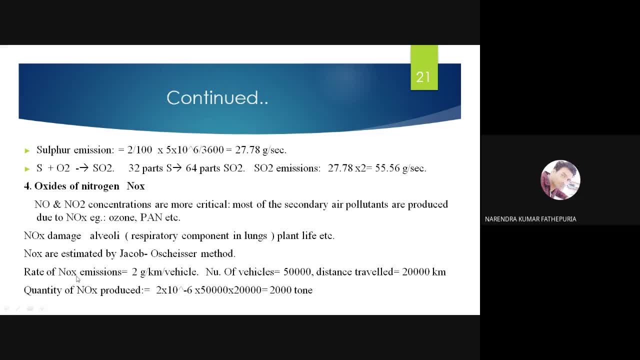 So is done. This is moving. source of dust. NOx emissions are coming two gram per kilometer per vehicle. Number of vehicles around, suppose, 50,000.. Europa And no one knows me. But instead of because of the heavy antigens And for example, 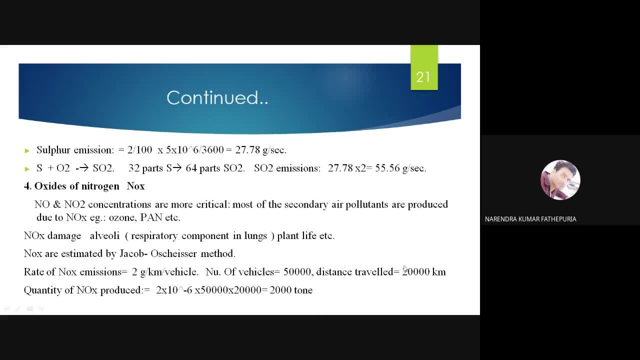 thousand. if you consider in a particular city, distance travel will be equivalent to twenty thousand kilometers. so quantity of nox produced, you can measure it two into ten, to the minus six, into fifty thousand, into twenty thousand, you will be getting a two thousand ton of nox gas. 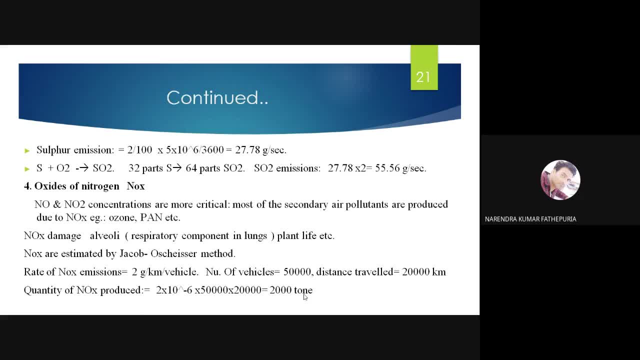 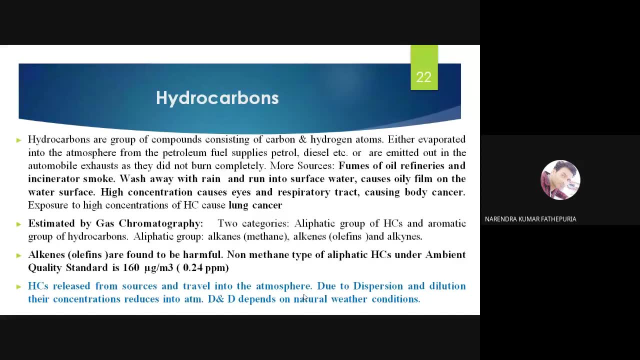 from the city. okay, so like this you can estimate it now. hydrocarbons- hydrocarbons- these are the unburned fuel, actually, while the fossil fuel based emissions liquid, but petroleum, gasoline, petrol diesel, kerosene and various uh complex chains of hydrocarbons and the coal also. it's a group of compound consisting of carbon and hydrogen atoms. 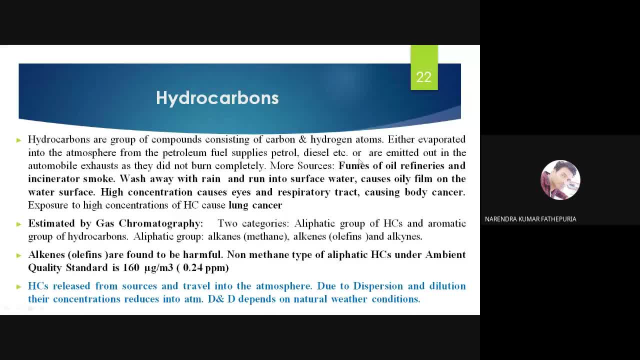 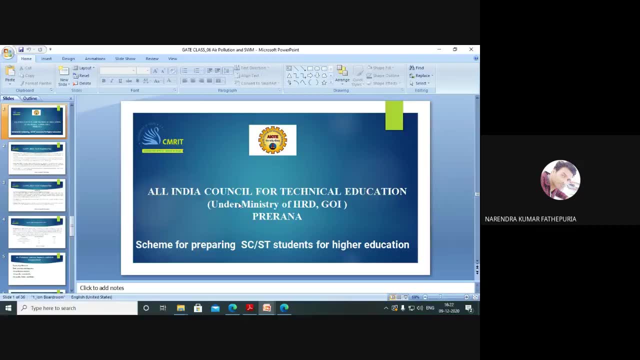 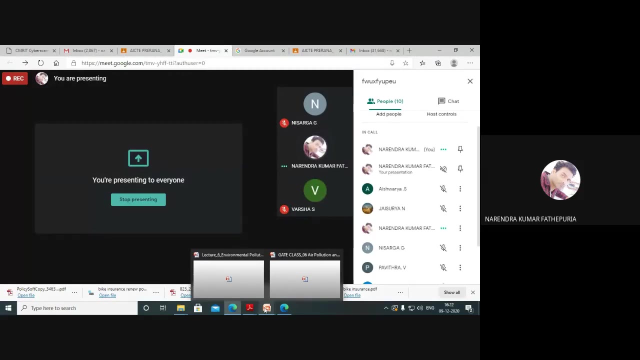 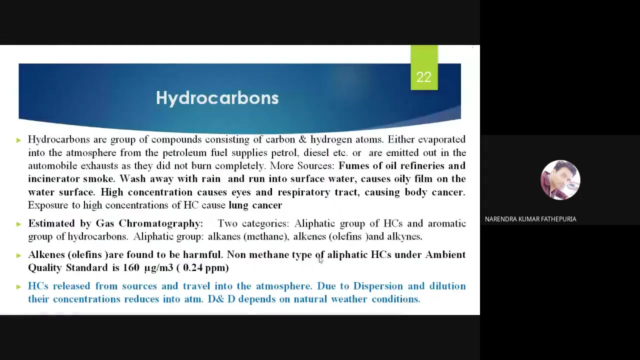 either evaporated in the atmosphere from the petroleum fuel supplies, petrol, diesel, etc. or are l emitted out in the automobile exhaust, as they did not burn completely. next a second. yeah, did not surface the fumes of oil refineries. these are the main sources of hydrocarbons. 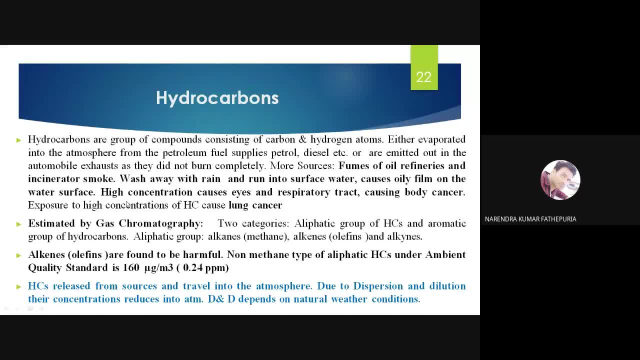 except petrol, lasers and kerosene and all that, the fumes of oil refineries and incinerator is smoke. so most of the cases you are using incendiator in most of the industries, like uh uh, various automobile industries, various thermal power plants, as well as an incinerator based waste. 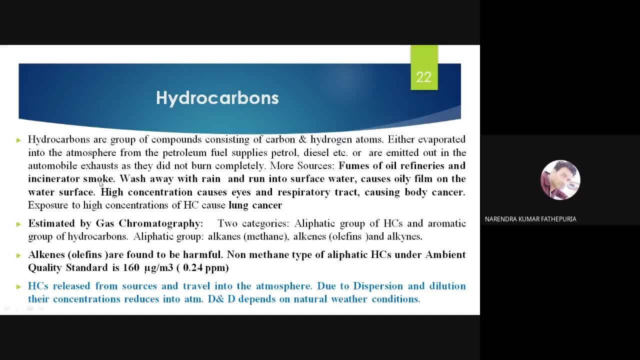 to energy plant. you are using incinerator smoke so that the smoke is also having unburned fuel and wash away with these all polythene hydrocarbons. once the rainfall occur in a particular area, these all polythene hydrocarbons will wash away with the rain and run into the surface water. 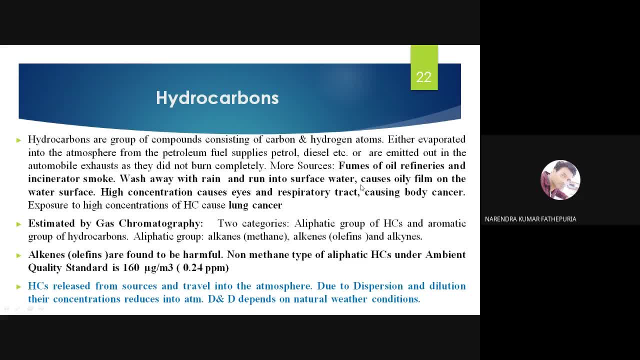 causes oily film on the water surface. high concentration causes eye and respiratory tract problems, causing body cancer also. low concentration- that much of significance is not there. exposure of high concentration of hydrocarbons causes lung cancer also. these are again the adverse impact on the planet as well as on the human being life. 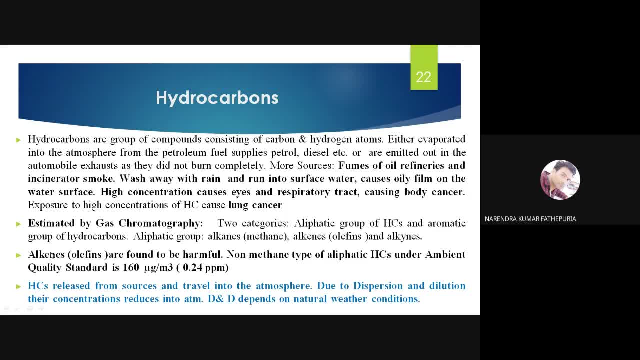 various body cancers and lung cancers will be the reason because of the hydrocarbons. so hydrocarbons are measured by the gas chromatography. there is a gas chromatography analyzing mechanism. this is the laboratory analyzing mechanism of various gases. there is a liquid gas chromatography. gas co-chromatography. 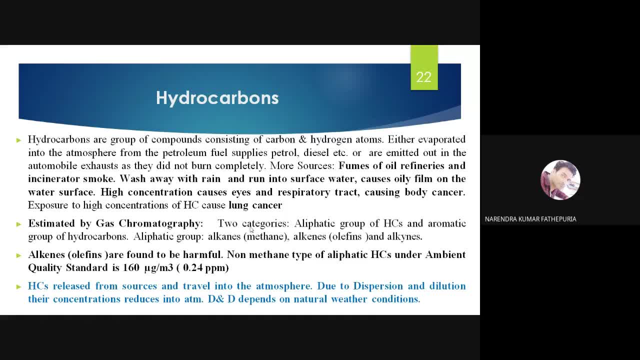 there is various type of gas chromatography. it is experimental analysis method. so while you are analyzing the gas chromatography, you are analyzing the gases, because analyzing the gases is more difficult than liquid and storing the gases is also very difficult. there are various properties. some of the gases are highly active in the atmosphere. 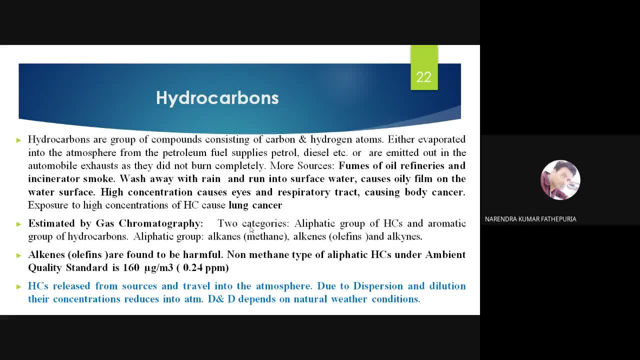 highly chemically reactive. some of the gases are very ignitable in the nature. so we have to understand the various properties of the gases. hydrocarbons estimation can be done by the gas chromatography method. there are two categories. one is the aliphatic group of hydrocarbons. 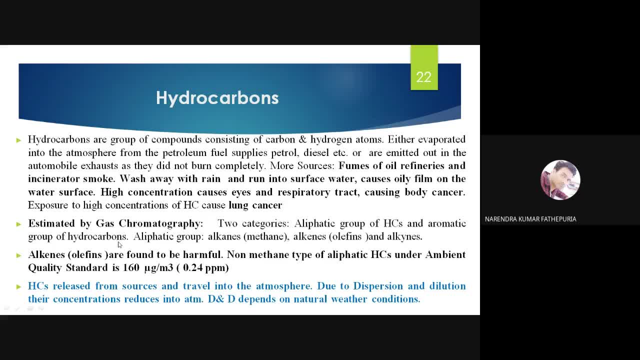 and second one is the aromatic group of hydrocarbons. we have studied about the organic chemistry. then you can understand the aliphatic group of hydrocarbons and aromatic group of hydrocarbons. so aliphatic groups of hydrocarbons like alkenes, methane, alkenes, olefins and alkynes. 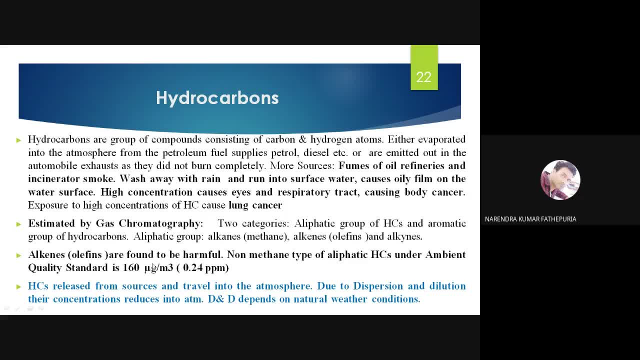 olefins are more dangerous, so alkenes olefins are found to be harmful. non-methane type of aliphatic hydrocarbons- the most common aliphatic hydrocarbons- under ambient quality standard condition is 160 micrograms per cubic meter. 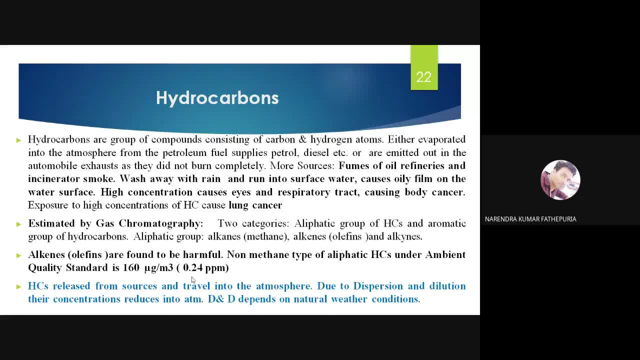 I will come for the national ambient air quality standards later on. there is the air quality monitoring index, there is air quality index, there is the national ambient air quality index that you have to maintain. these are the standard emission standards. like we have water effluent standard, drinking water effluent standard. 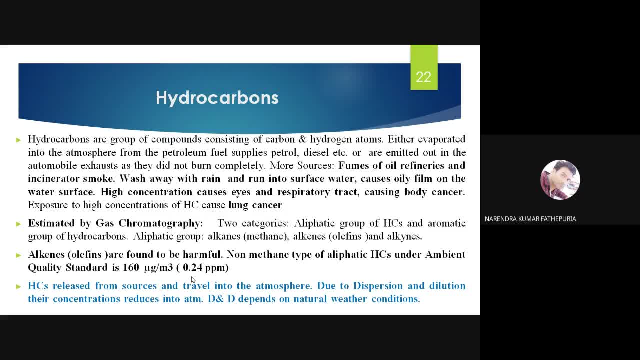 industrial water, wastewater effluent standard. in the same way we have air quality standards also. so the various pollutant is ranging from the various industries. so what should be the standard limit? someone has to there to control right and regulate. so the central pollution control board and all that. 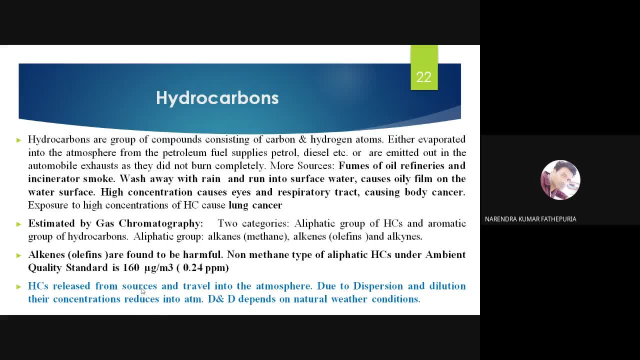 they have, and then environmental protection agency EP has decided the standard. so how much CO2 can be accepted, how much hydrocarbons can be accepted in the particular atmosphere and how you will decide the green zone, red zone and yellow zones and severe zones and sensitive zones. 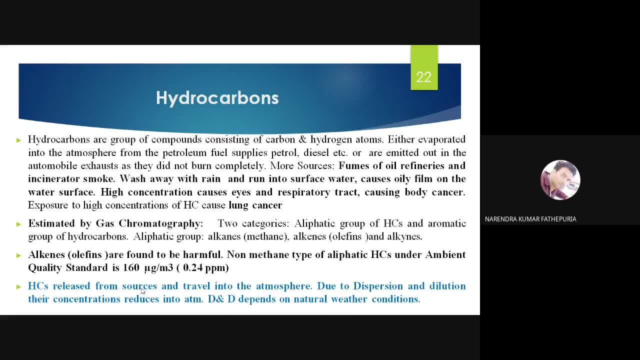 right based on the air pollution. the percentage of air pollution that we are getting in a particular area, suppose the particulate matter. the assessment of particulate matter is getting very high. more than 300 to 400 micrograms per cubic meter means this area is called as very sensitive. 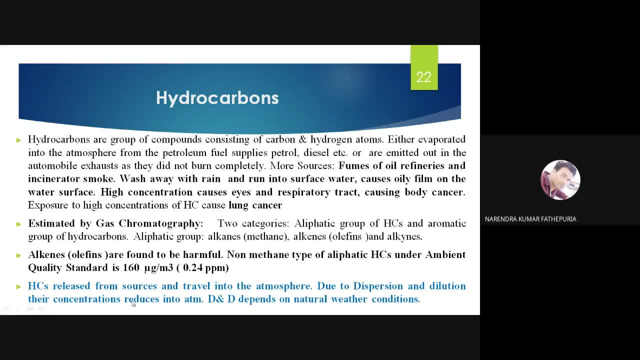 so I will be talking later about the joints in all that. air quality monitoring standards. right. so hydrocarbons released from the sources and travel into the atmosphere due to the dispersion and dilution. these are dispersion and dilution. these are the both techniques and natural methods. 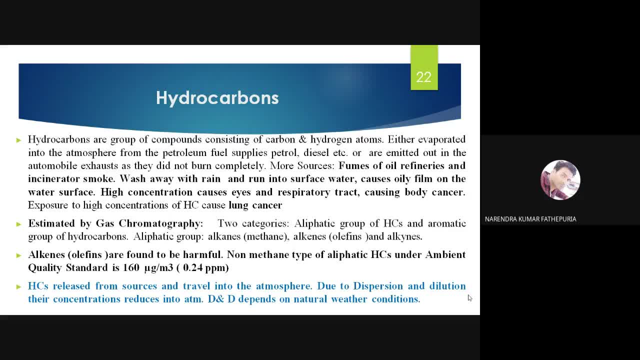 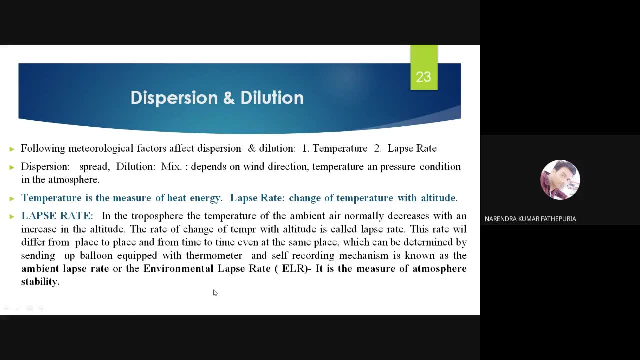 for reducing the air pollution and pollutant into the atmosphere. I will be talking later about the dispersion and dilution details. their concentration reduces into the atmosphere, so dilution and dispersion both depend on the natural weather conditions. because natural purification process. I will be coming for the dispersion and dilution. 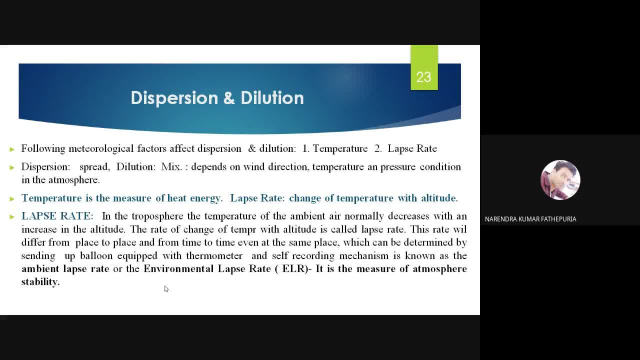 both are the natural processes. generally, if you see, a dispersion means the spread actually. so once the air pollutant is accumulated somewhere in that area, once it is released from the source, it has to spread in the air right. some of the time it depends on the various climatic conditions. 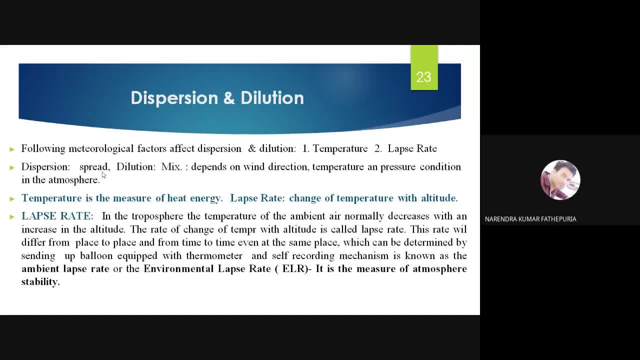 what is the temperature, what is the wind speed and what is the pressure? right? so all the factors, climatic factors, play an important role while the dispersion is happening. more dispersion is happening means the pollution that is in the air. more dispersion and dilution following metal with other temperature. 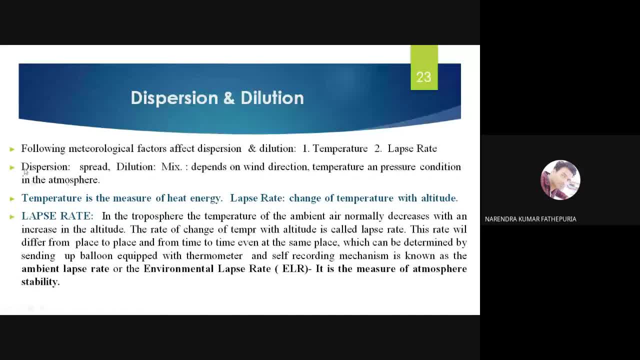 second is the lapse rate. I will be talking about the temperature, lapse rate and pressure one by one. then, simple term: dispersion means집 spread, dilution means mixing, depends on the wind direction, temperatures and then and then pressure conditions in the atmosphere. we have already classified the various spheres. 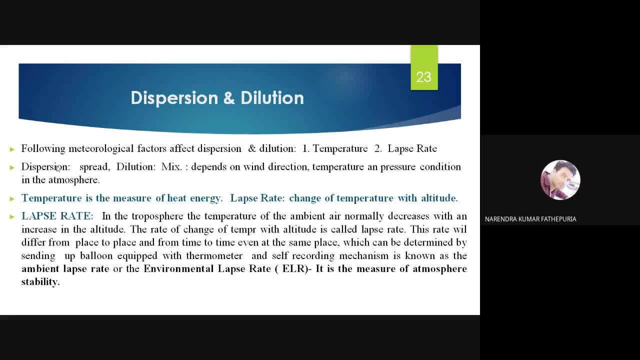 mesosphere, ionosphere, stratosphere, troposphere, all that. there's a temperature range and the flow meter in height. so with respect to altitude, with respect to height into the atmosphere, these various layers will depend. so temperature is the measure of heat energy number one. left street is the change of temperature with altitude. so there's a change of temperature on y-axis and 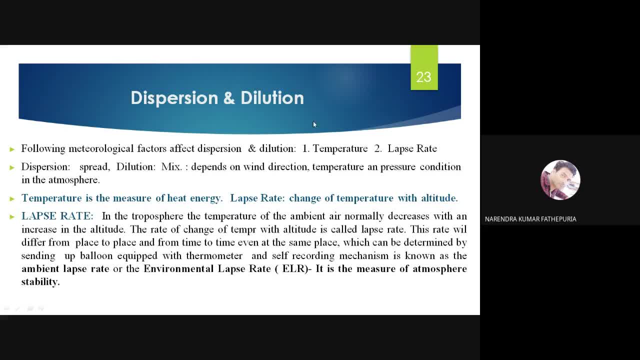 altitude. no, there's, the altitude will be on a y-axis in height and then temperature will be on x-axis. then once you plot this graph, once you slope this, I will be going for the graph in all that slope it. so, change of temperature with altitude will call it as the left rate. this. 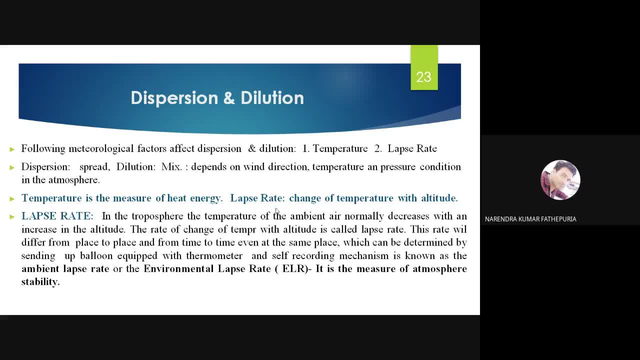 is very important while you are deciding the condition of the weather, condition of for of the pollution label into the, into the atmosphere. so let's really play a very important role for the metallurgical point of view. so I will talk about the one by one. this is a left rate. 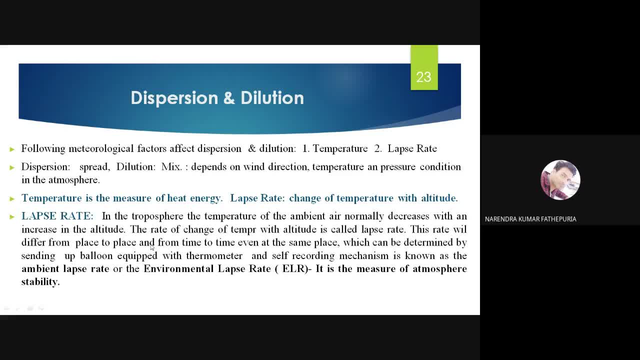 and in the proposed sphere, the temperature of the ambient air normally decreases with an increase in the altitude. this is the common theory right in the atmosphere region. the pressure of the ambient air normally decreases with an increase in the altitude. the rate of change in temperature with altitude is called as left rate. 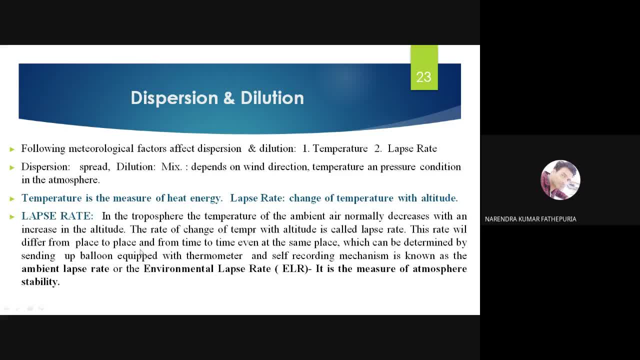 and this rate will differ from place to place. these are the terminologies and technical terms that we are going to use it while you are analyzing and measuring the pollution. once you analyze, once you measure the quantity of pollution, then you can find out the solution. so the controlling measurement part- control part of the pollution will be different. so 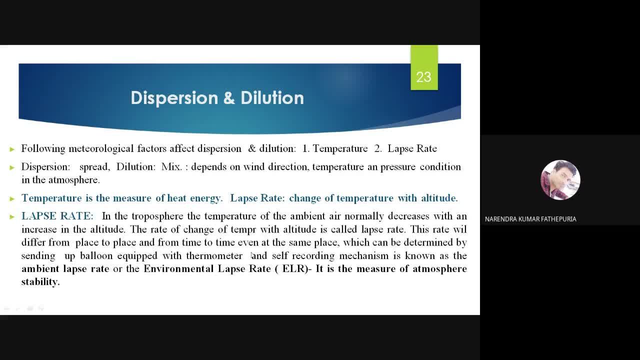 we are talking later, right? so this rate will differ from place to place, and from time to time even at the same place, which can be determined by sending up balloons equipped with the thermometer recording mechanism, is known as the ambient lapse rate, or sometimes we call it as the environmental. 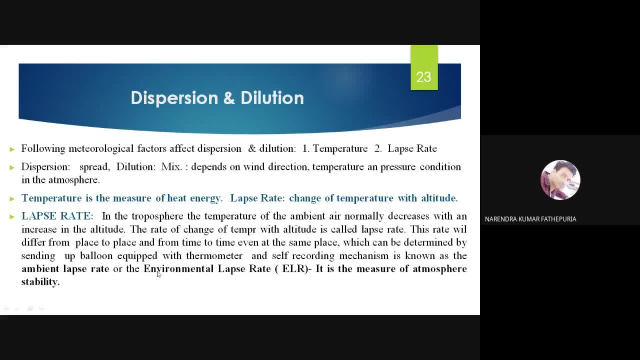 lapse rate. from now onward we will be calling as the ELR. yeah, environmental lapse rate. so what is environmental lapse rate? how to determine it? there is a balloon you have which we are sending up this value. it could be the thermometer. so, with respect to height balloon will go in a on a vertical height. 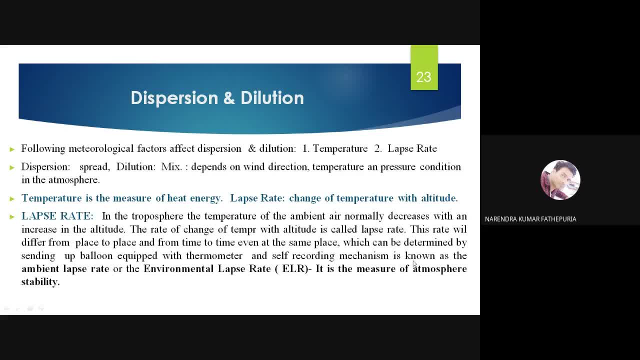 into the atmosphere based on the temperature range. it will be recording. there's the self recording mechanism there for the temperature and height- and then automatically the graph will be plotted with between the temperature range as well as the height and then every time you will get the environmental lapse rate. so this phenomena is 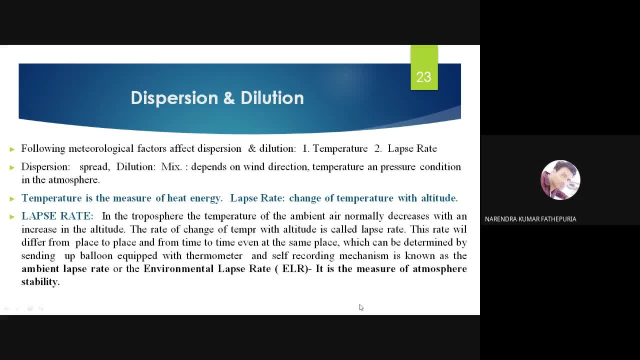 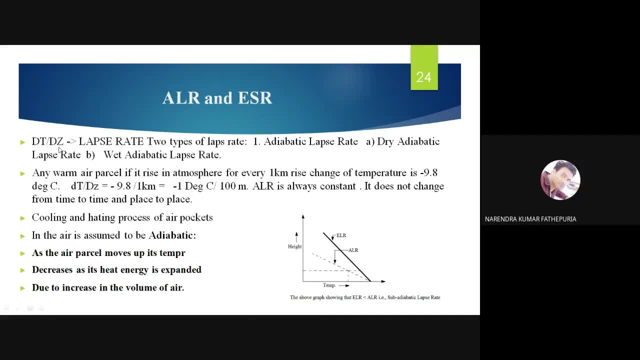 called as the ambient lapse rate. yeah, environmental lapse rate. that is the measure of the atmosphere stability, actually how the stability is that atmosphere. so we can generally denote as the dt by dz here. this is the lapse rate- environmental lapse rate. two types of lapse rates are there. 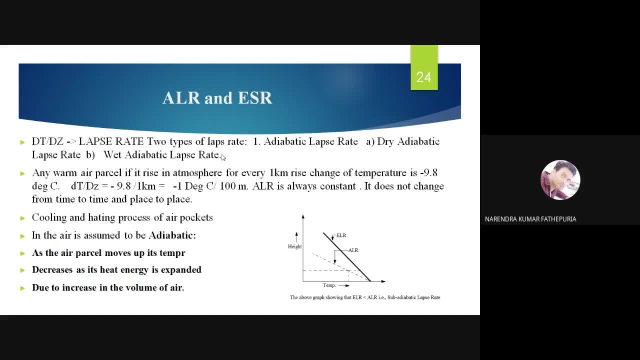 the second is an adiabatic lapse rate. are having the two types again: dry adiabatic lapse rate and wet adiabatic lapse rate. okay. so number first is adiabatic lapse rate. there are the two types again: dry adiabatic lapse rate. I will be calling as d a l r and this is wet adiabatic lapse rate: w a l r. okay. 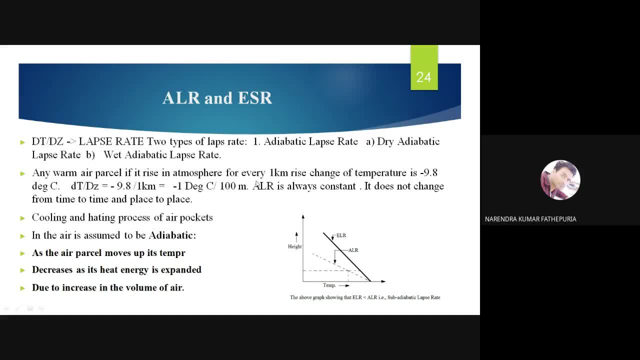 so any warm air parcel, if it is, rises into the atmosphere. for every one kilometer rise changes of the temperature is minus 9.8 degrees Celsius. so dty dz, you can get it minus 9.18. this is a change of temperature DLT divided by one kilometer, so you will be getting a minus 9.8. 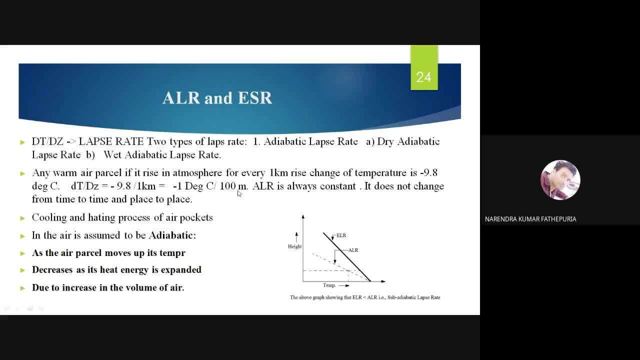 and you can write it: minus one degree Celsius divided by 100 meters. so alr is always constant. the adiabatic lapse rate will be, will remain always constant. so there's adiabatic love for gases that I will talk later. okay, it does not change from time to time and place to place cooling and heating process of air pockets. 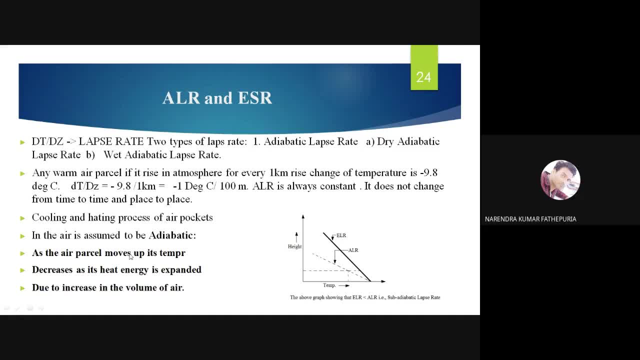 uh, I will explain this map, this mechanism- this is a natural process actually- how the cooling of waves, cooling of air will be taking place and how it will be, uh, heating of, like, how the heat exchange and because the conduction and convection process will be taking place for the 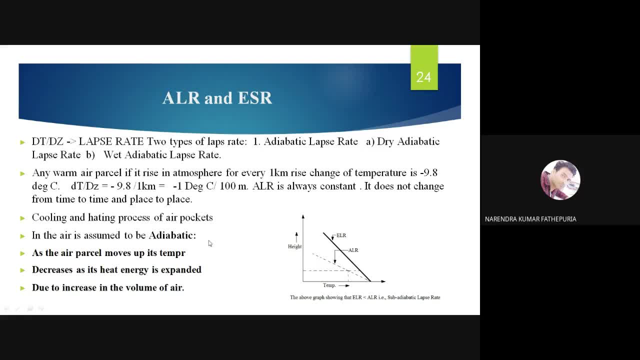 uh, for the air wind, the hot air as well as the cool air. right, so there are the various air pockets. okay, we will deal with just a reasonable cause here. of course there are adiabatic processes, naught Prin. a addition of the flux will injure an advance mass. so, uh, the anesthesia bin will chase even. 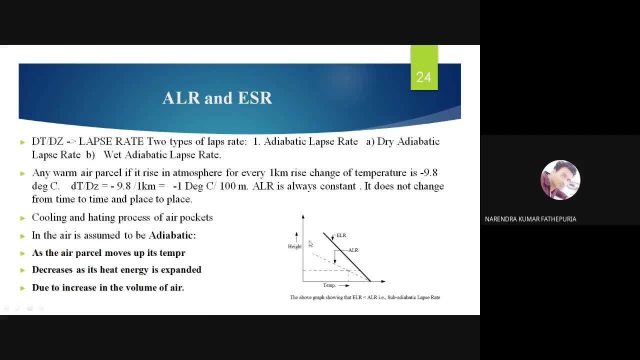 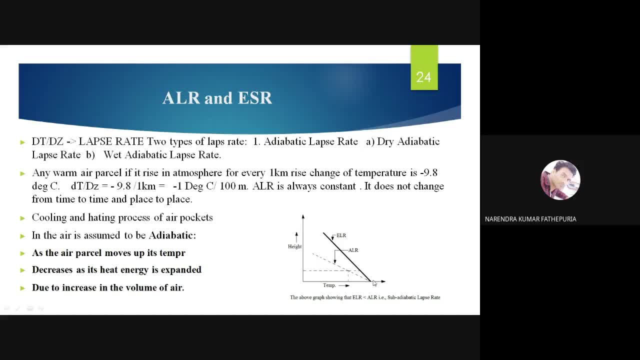 So you see there, this is the height on the y-axis and temperature on x-axis and this is the environmental lapse rate. darker one is the environmental lapse rate and this dotted one is the adiabatic lapse rate. So adiabatic is the ideal conditions, but we assume that the whole atmosphere, the lapse 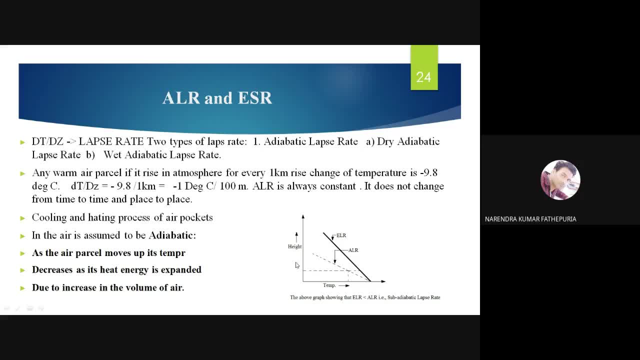 rate will be considered as adiabatic one. So everywhere you can put a slope and x-axis and y-axis and you can get the ratio. So suppose here you can put a slope and then you can get a environmental lapse rate. 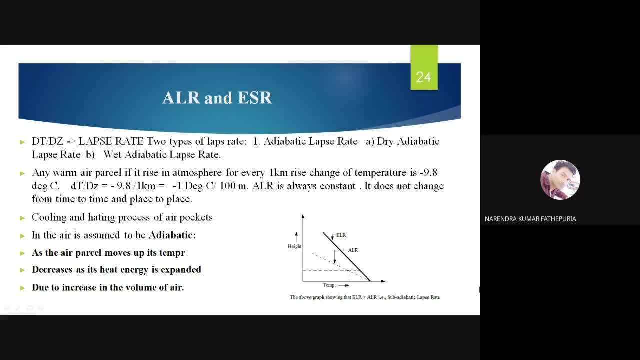 This is a common phenomena. so if the air pocket your air parcel moves up with the temperatures, its temperature start decreasing and it is like releasing the heat energy, and heat energy will be used for the cooling air. there is a cool air and warm air, so heat. 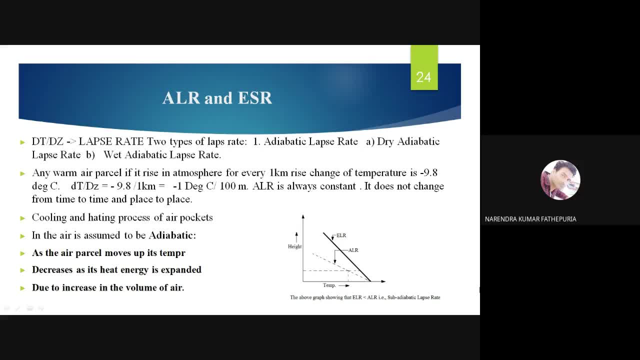 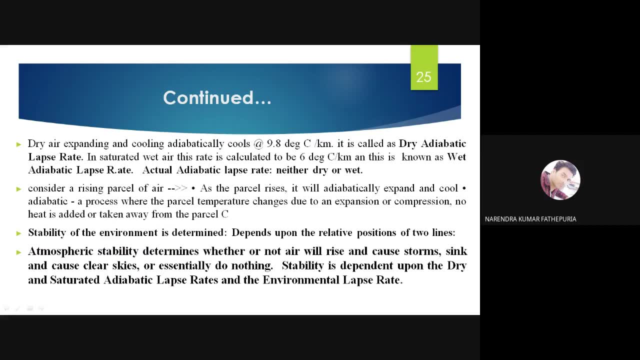 energy will be supplied from the hot air to the cold air, From the higher temperature to lower temperature. so there is a convection process will be taking place. So what is happening here, in the whole process and mechanism, in the stratosphere mechanism? 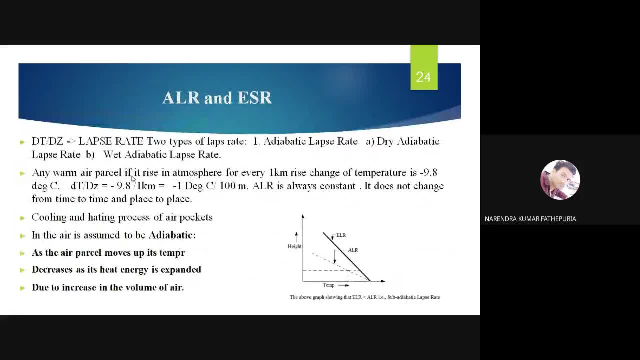 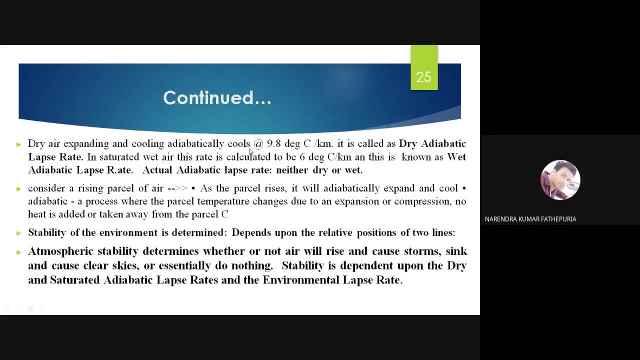 once this air pocket moves up, the temperature goes down and heat energy is expended due to increase in the volume of the air. Dry air expanding and cooling adiabatically cools at a 9.8 degree Celsius temperature per kilometer. 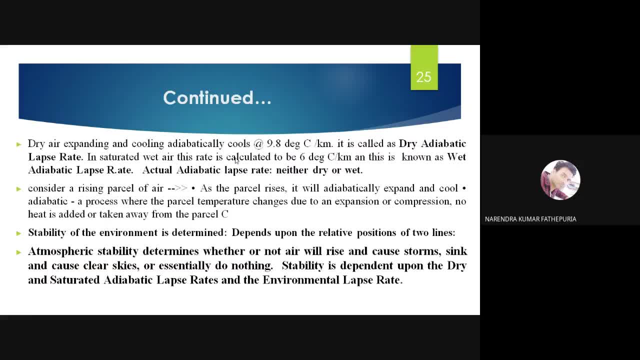 Suppose in this example they have taken an example. they have taken that example, So it is called as a dry adiabatic lapse rate and saturation: a saturated wet air. this rate is calculated to be a 6 degree Celsius per kilometer and this is known as a wet adiabatic. 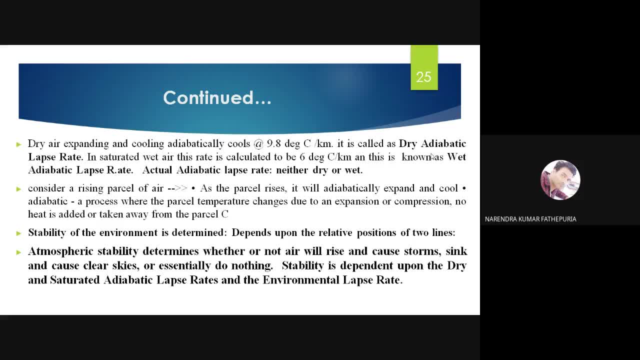 lapse rate. So these are two adiabatic rates here: dry adiabatic lapse rate as well as the wet adiabatic lapse rate. So actual adiabatic lapse rates, neither dry nor wet. So in between it works. 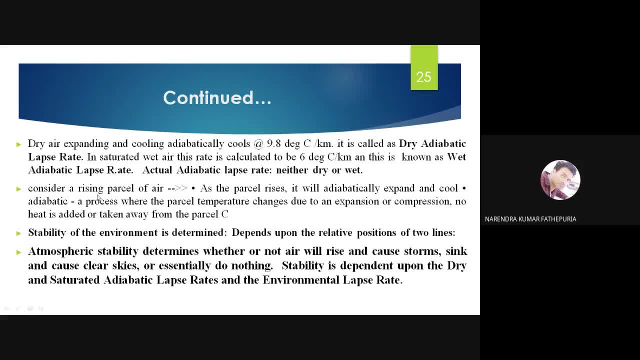 So let us see So. consider a rising parcel of air. as the parcel rises, it will adiabatically expand and cool. Adiabatic is a process where the parcel temperature changes due to an expansion or compression process. No heat is added or taken away from the parcel. 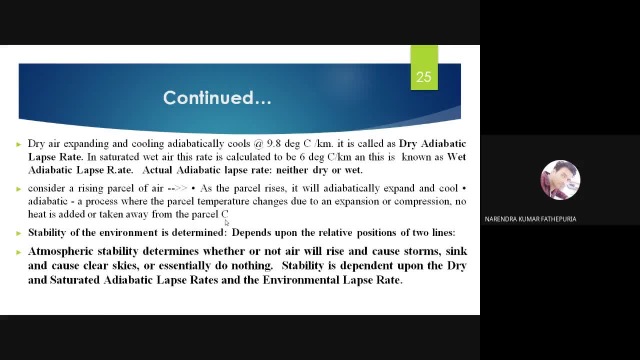 Okay, So that is the constant rate, or adiabatic lapse rate is the constant rate. There is no heat exchange. Okay, Okay, So there is no heat exchange taking place, no addition, no taking away and the partial temperature changes due to the expansion and compression. 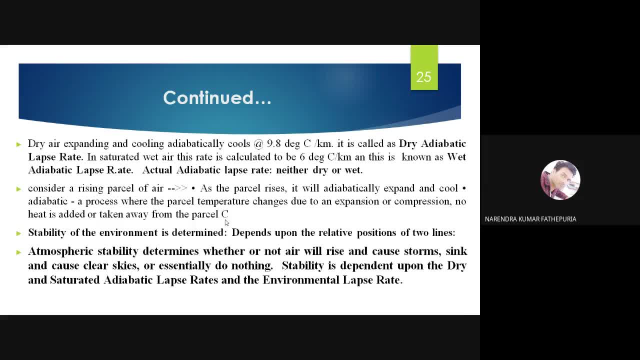 So simultaneously, expansion will be happening. On the other side, compression will be happening. So there is no. So it will balance reaction. actually, Stability of the environment is determined. as I told you, it depends on the adiabatic. 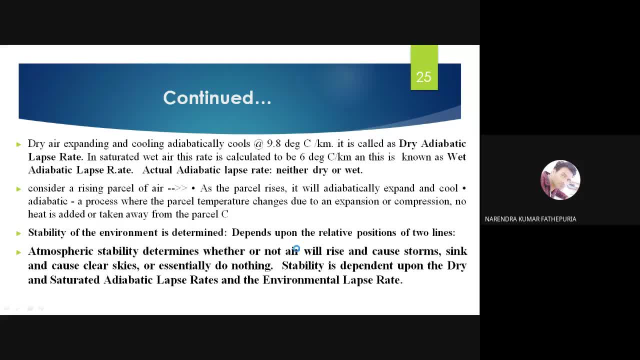 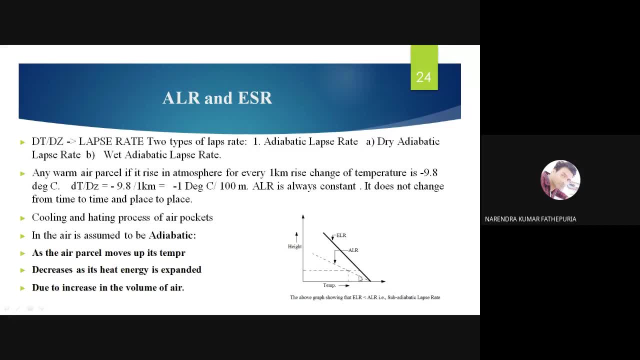 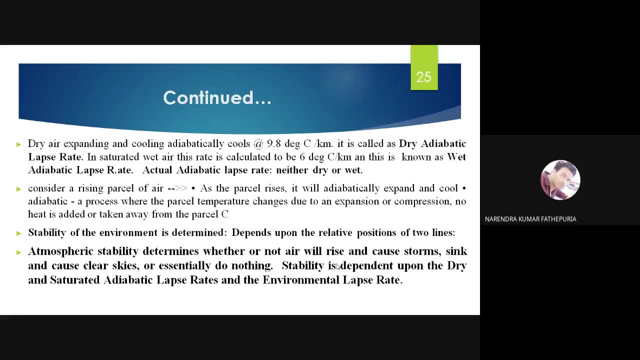 lapse rate and environmental lapse rate depends upon the relative position of two lines. These are the two lines. Okay, are the two lines? elr environmental lapse rate and this is the adiabatic lapse rate with respect to height and temperature. so, uh, these, these both lines, will keep changing based on this stability. 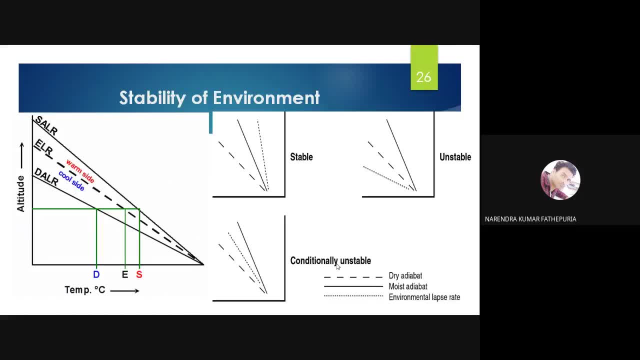 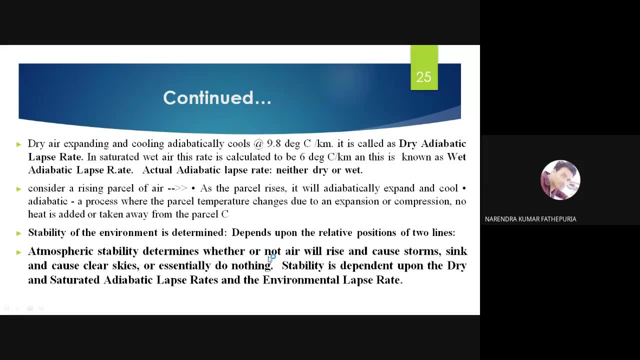 will measure. so every talking about the stability part, there are one by one, i will come. this is atmospheric stability. uh, atmospheric stability determines whether, whether or not air will rise and cause storms, sink and cause clear skies or essentially do nothing. the stability is dependent upon the dry and saturated adiabatic lapse rate and the environmental lapse rate. so, whether you 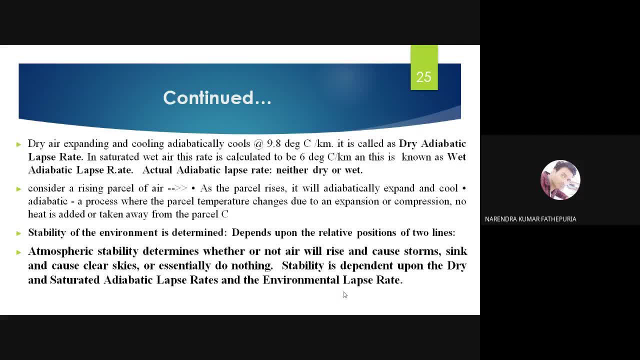 are going to determine what will be the condition into the atmosphere: whether atmosphere is stable, whether atmosphere is suitable for the pollution dispersion or not. more dispersion will be happening. more dilution will be happening means the there is, the more chances. then quickly the pollutant will disperse easily. the sky will be clear. okay if there is a dispersion. slow if there. 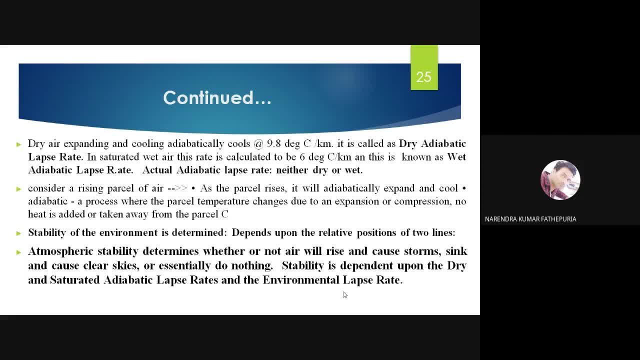 is less dilution means the more time will take to or take away the pollutant. so it is very important to understand the stability and it depends on weather condition, temperature, as i told, wind speeds or pressure, everything above that. so this is the stability of the environment. 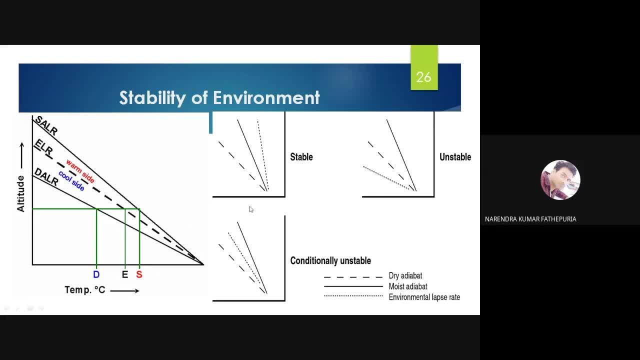 this is the height and this is the. these are the various graphs. height versus temperature. the environmental left street: this is the adiabatic left street and this is the isothermal condition. so both are keeping away. this is a stable condition right now. environment: this is the dry adiabatic left skin: this is the wet adiabatic. 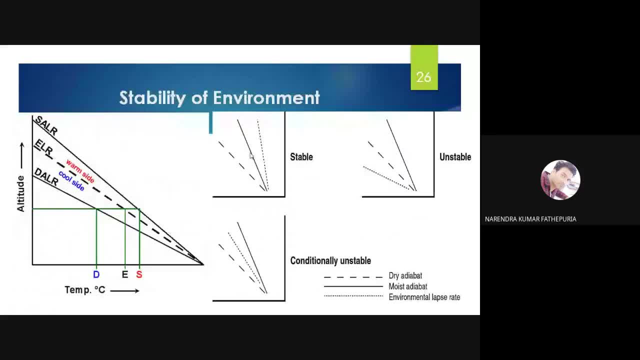 yeah, so the sea land will decide the stability criteria. this is the stable condition, and this is then a stable condition where the environmental episodes is far away from the adiabatic left straight and this one is down. okay, i'll be talking later about all this. i will come. 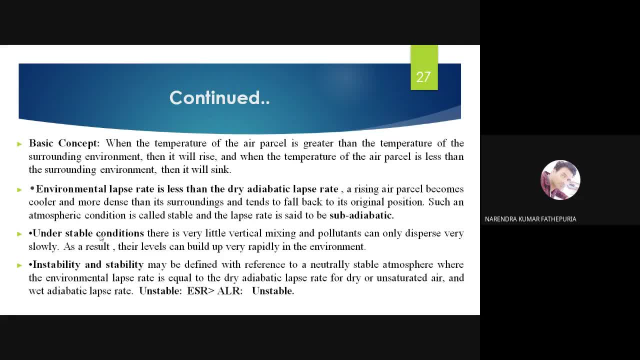 back up for this graph again. so what is the basic concept here? when the temperature of the air parcel is getting higher or's going down? we will see later on that we will come back up for this graph. so what is the basic concept here? when the temperature of the air parcell is getting? 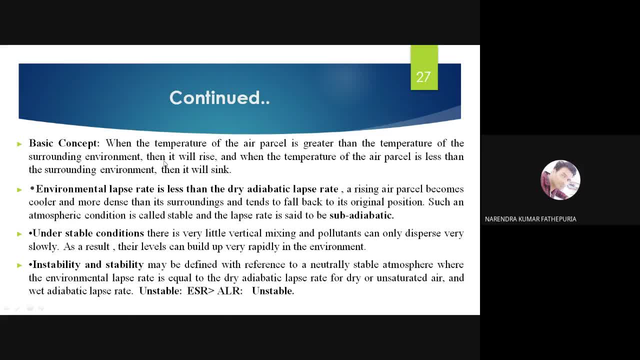 air parcel is greater than the temperature of the surrounding environment, then it will rise, And when the temperature of air parcel is less than the surrounding environment, then it will sink. There are two conditions: sink and flood. So both conditions will depend on the temperature. If the temperature of the air parcel is greater than the temperature, 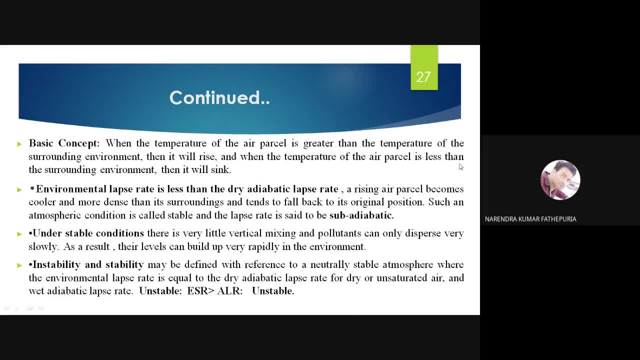 of the surrounding, then it will rise, And when the temperature of the air parcel is less than the surrounding, then it will sink. So, environmental lapse rate: there are the three conditions. we will be talking here about the three conditions, These three conditions. 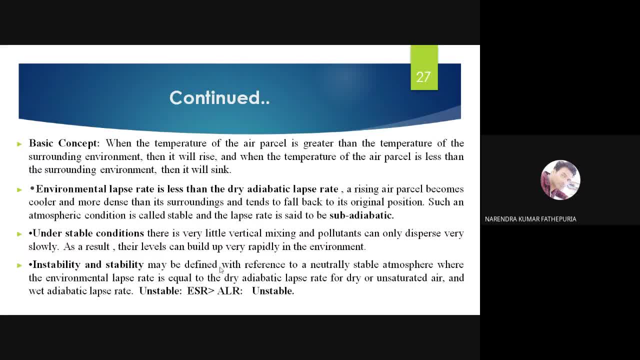 we will be talking here stable, unstable, neutral conditions. So one condition. there is the first condition, the environmental lapse rate, which is less than the dry adiabatic lapse rate. Some of the terms are new for you, I think, so don't get scared here. So 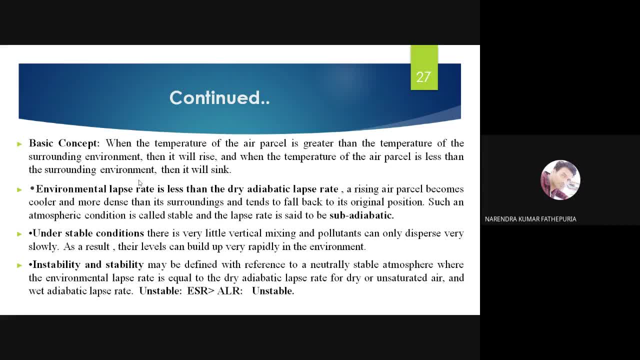 you have to understand the environment. If you have studied as elective your air pollution control, then you can do that. There is the environmental lapse rate, which is less than the dry adiabatic lapse rate. This is one condition. Here. ELR is less than the dry adiabatic condition. What is going? 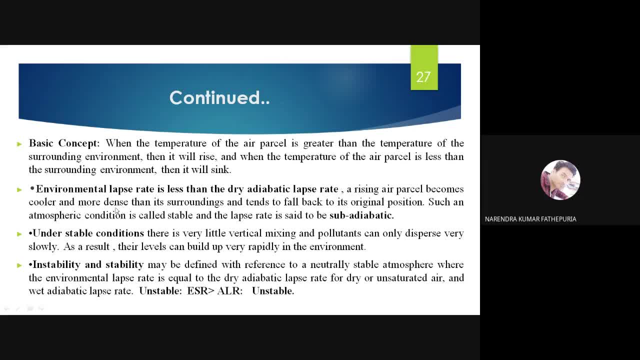 to happen in this. A rising air parcel becomes cooler and more denser than its surrounding and tends to fall back to its original position. Such an atmospheric condition is not going to happen. So the atmospheric condition is called a stable and the lapse rate is said. 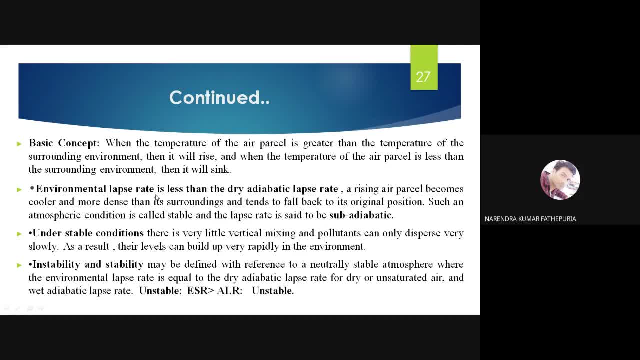 to be a sub adiabatic. So in the environment, if the ELR is less than dry adiabatic lapse rate, then sub adiabatic conditions will be taking place. Number second is the. under stable conditions This is very little vertical mixing and pollutants can only disperse very slowly. As a result, their levels can build up very rapidly. So the level of adiabatic lapse rate which is less than the dry adiabatic lapse rate is less than the dry adiabatic lapse rate. So in the environment if the ELR is less than dry adiabatic lapse rate, then sub adiabatic. 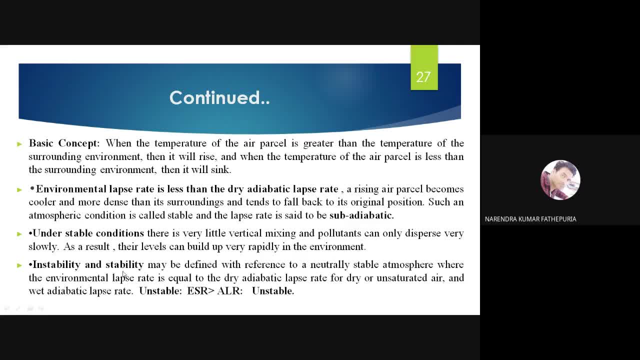 system can build up very rapidly. The third one is the instability condition. Stimulate one meter. So I said first of all the admissibility condition of sub adiabatic lapse rate which is less than the dry adiabatic lapse rate which is less than the dry adiabatic lapse. 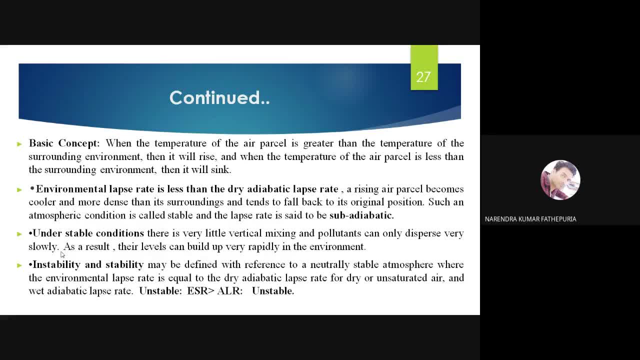 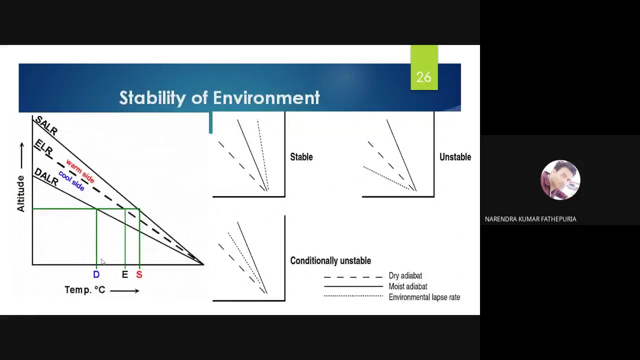 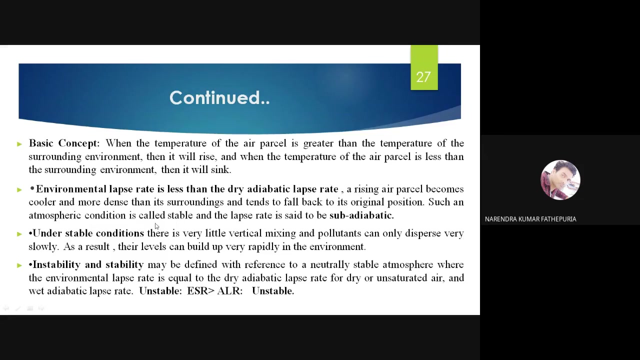 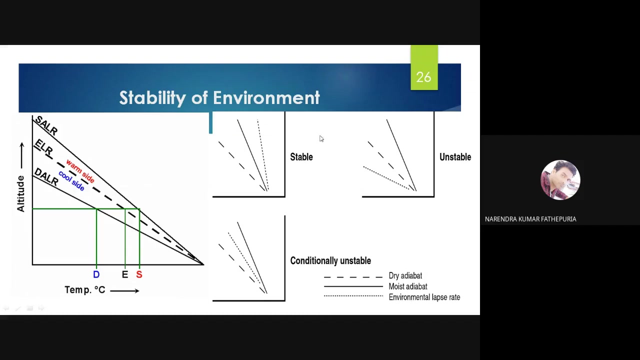 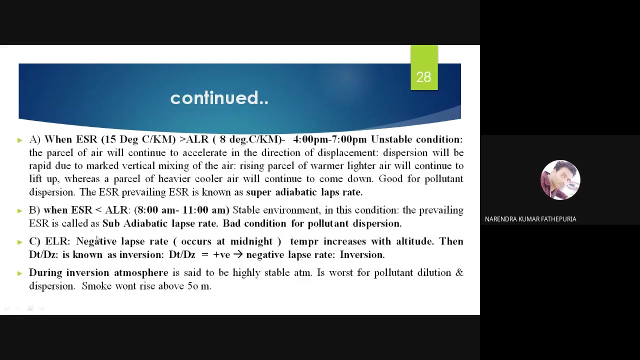 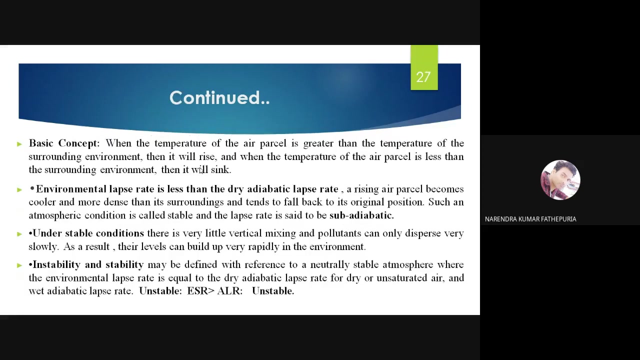 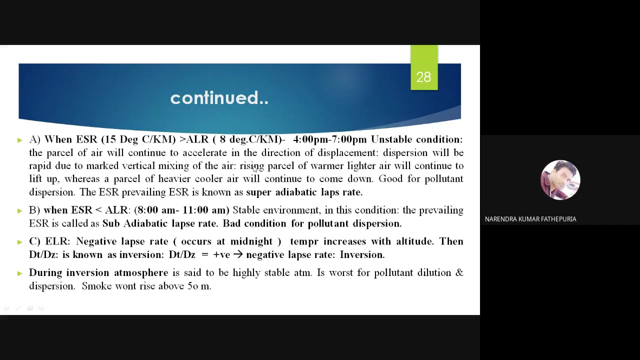 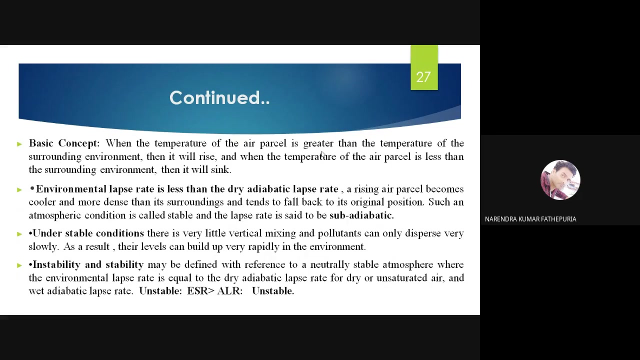 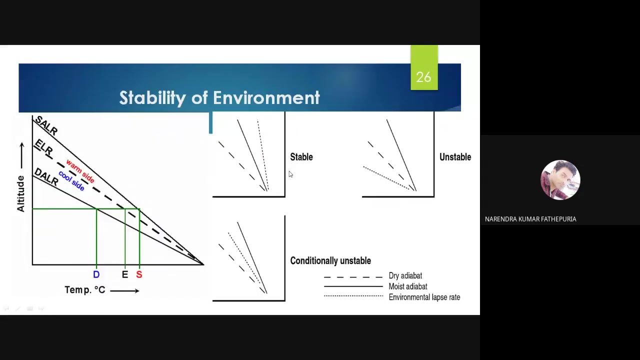 rate. So here we were talking about the environmental stability rate. okay, And there are the conditions for it. temperature: This condition is called as stable condition, where ELR rate will be less than 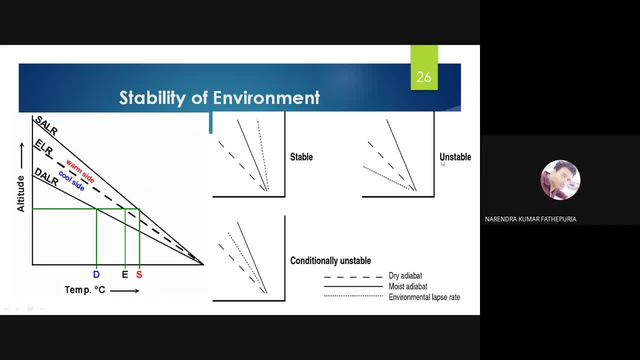 to what we called as ELR rate And unstable condition. highly unstable condition means when the ELR rate is greater than to the ALR rate, adiabatic lapse rate. This is unstable condition And there is one condition: where ELR rate is equal to ELR rate, which will be: 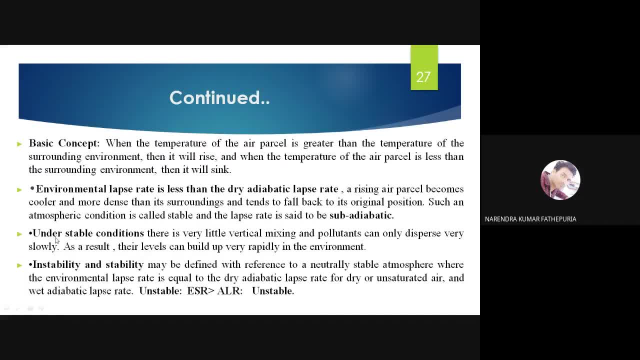 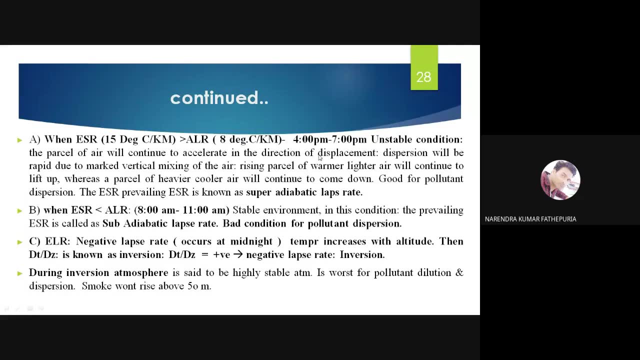 called as here, which will be the neutral condition. So stability and instability of the environment will be decided based on this rate only. So first condition: we will be talking here. It generally occurs at 4 pm to 7 pm in this timing And it is a highly unstable. 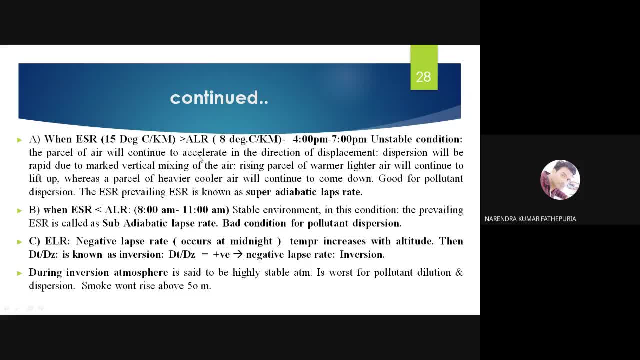 condition. What will happen in this case? The partial of air will continue to accelerate in the direction of displacement. Dispersion will be rapid due to the marked vertical mixing of air Rising. partial of warmer, lighter air will continue to lift up, Whereas partial 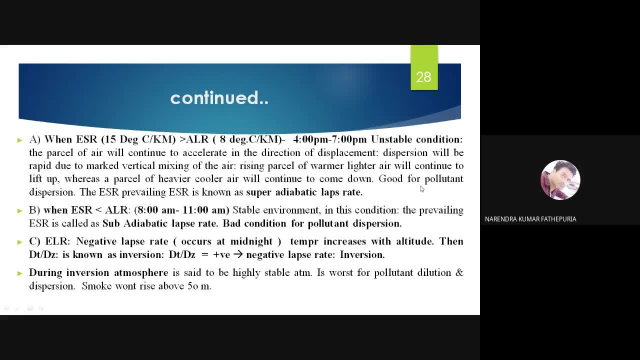 of heavier, cooler air will continue to come down. Good for the pollutant dispersion. This condition is good for the pollution dispersion. The ESR- prevailing ESR is known as the super adiabatic lapse rate, So sometimes we call it as a super adiabatic lapse rate, And this condition is good for the environment. It's. 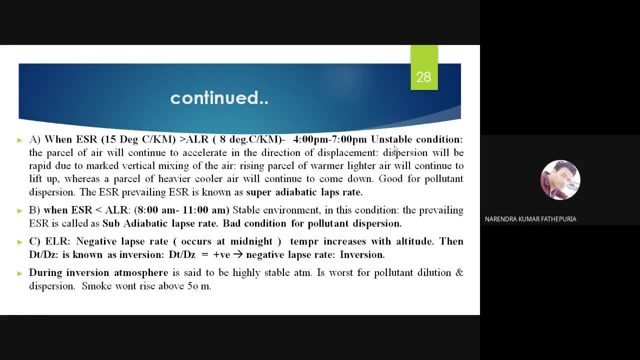 unstable condition because highly unstable environment will be good for the pollution dispersion. This is a simple concept for it. So the environment is highly unstable when it will be, when the ESR is greater than ALR. In that condition it is good for the pollution. 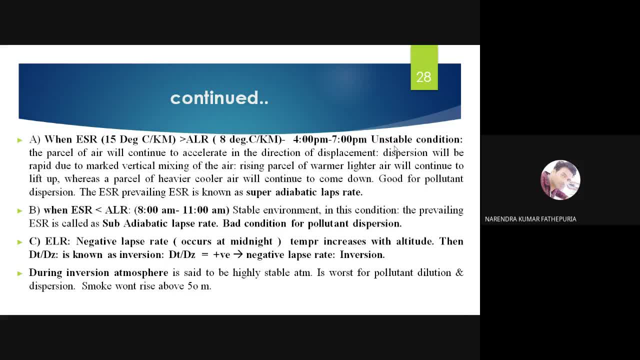 dispersion or easily the sky will be clear from the pollution. The second is when the ESR is less than ALR. It will be occurring in the morning hours, 8 am to 11 am. Stable environment. it is, as I told you, In this condition the prevailing ESR is called as: 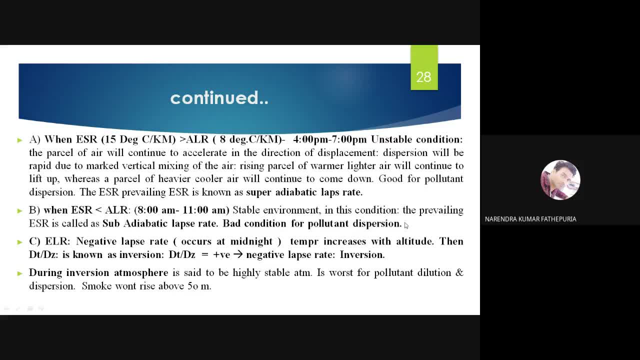 a sub adiabatic lapse rate. Bad condition for the pollutant dispersion in the morning, So generally in the winter season. the fog and all that. I will talk later about the fog, how the inversion will be taking place and all that. 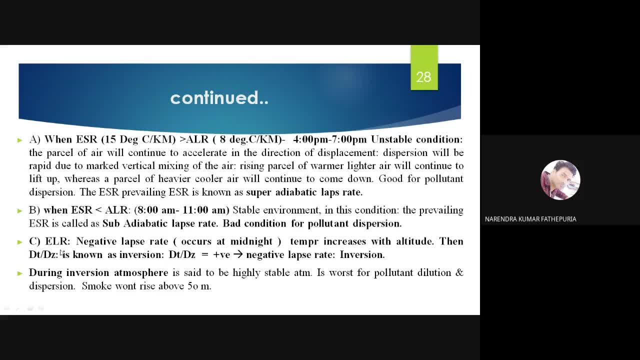 So this is the bad condition for the pollution dispersion. Third one is the ELR. This is called as negative lapse rate. Occurs at midnight, generally at midnight. So this is the negative lapse rate. Temperature increases with altitude. Then DT by DZ is known to be: is known as: 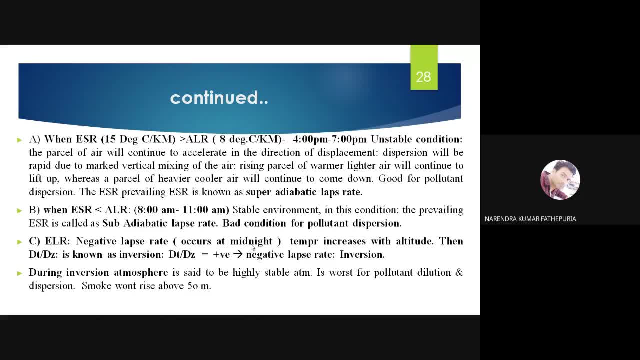 an inversion. So DT by DZ will be equal to positive And then it will be the negative lapse rate which is called as an inversion. Now, during inversion atmosphere, it is set to be highly stable atmosphere and it is worst for the pollution dilution as well as. 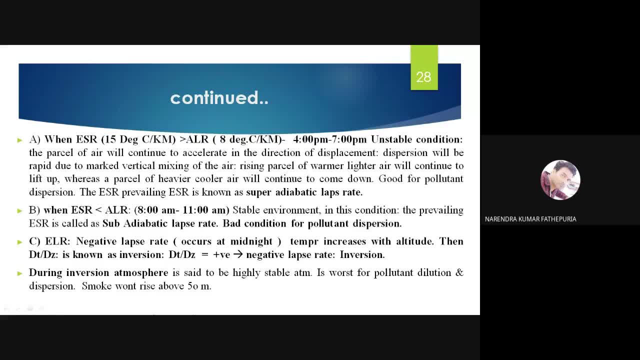 dispersion: Smoke born dries above 5 meters, above 50 meters in that condition. So inversion is the highly we can say stable environment which is very harmful for the nature because pollution will not happen, Pollution will not disperse Dilution as well as dispersion. 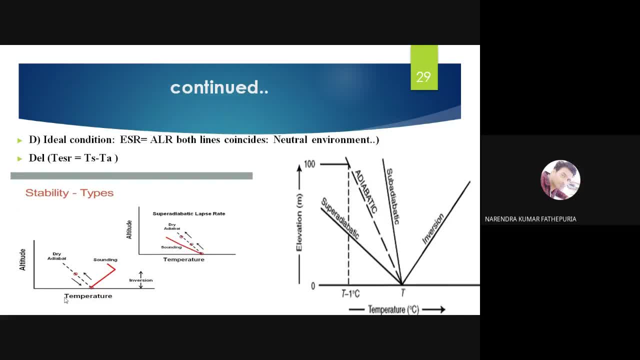 will not happen in this case. I will be talking later about the inversion. These are the ideal conditions. So here is the inversion where the ESR equal to ELR- Both lines- coincides each other and this is the neutral environment. This is neutral environment. You see here, this is the temperature. 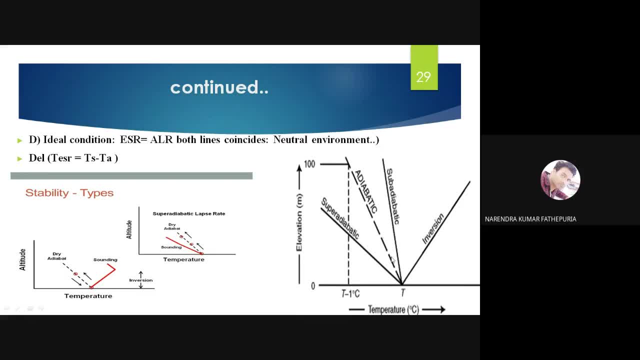 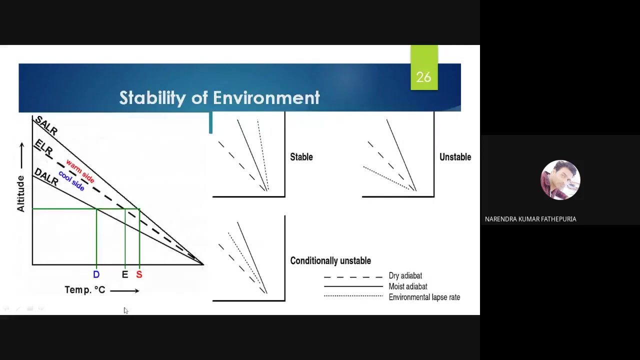 as well as this is the altitude, and this is the adiabatic, which is hard, is the adiabatic. 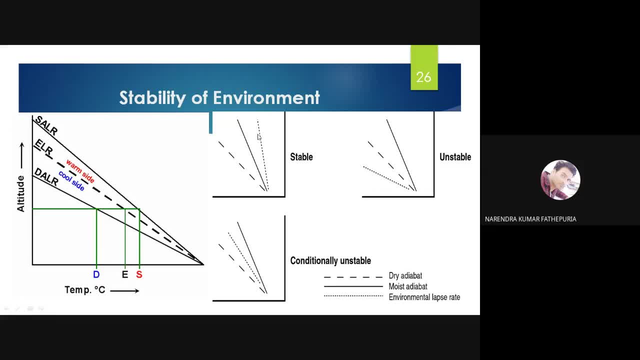 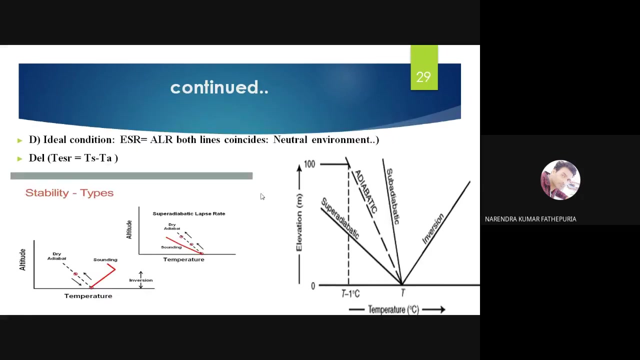 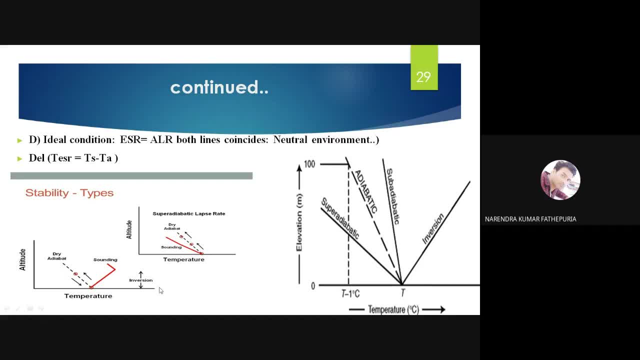 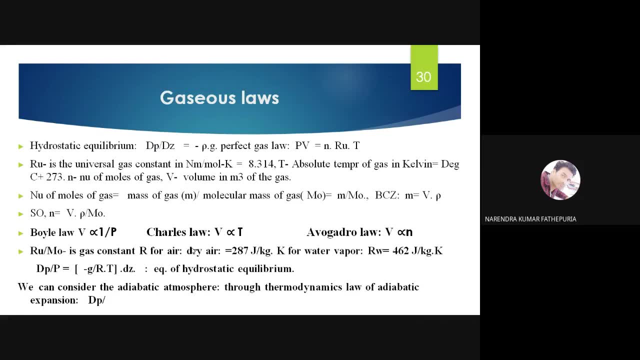 temperature versus altitude. This is dry adiabatic layer state and all that, how the temperature and all things will be happening. right For adiabatic layer state. Yeah, So there's a gaseous law that you have to understand for the dispersion and dilution techniques before. 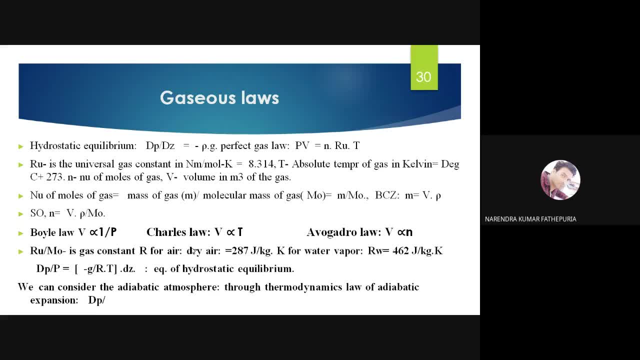 studying the dispersion and dilution. I will be taking two minutes for it, for explaining these gaseous laws. Then I will be coming for the main topic that I want to discuss today. So this is a hydrostatic eucalyptium. dv by dz is equal to minus rho into z. Perfect. 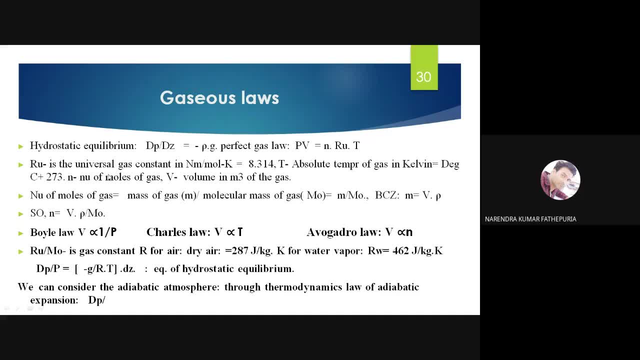 gas law you have studied in thermodynamics. part T is equal to n into r into 3.. r is the universal gas constant in neutron to meter per mole into Kelvin. In your 11th class also you have studied this In your engineering, first year engineering also you have studied. 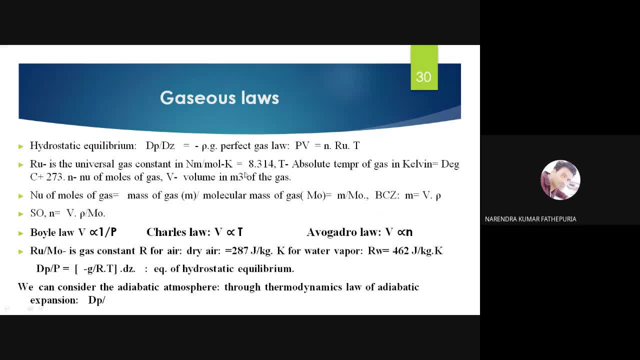 these things by gas law. Generally, in physics also they keep talking about it. 8.314, T is the absolute temperature of gases in Kelvin. Therefore this theory- I am not going for the details, Only main point- I am covering from the gate point of it And temperature. 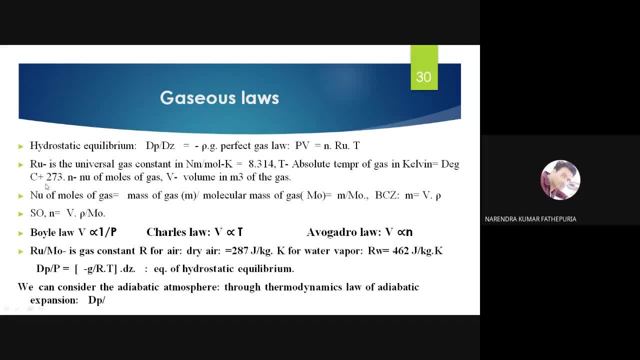 will be plus 273.. We have to take 273.16,. we have to add in the standard degrees of the temperature. N will be the number of moles of gases, V is the volume and magnitude of the gases, And number of moles of gases is equal to mass of gas: m per molecular mass of the gases. 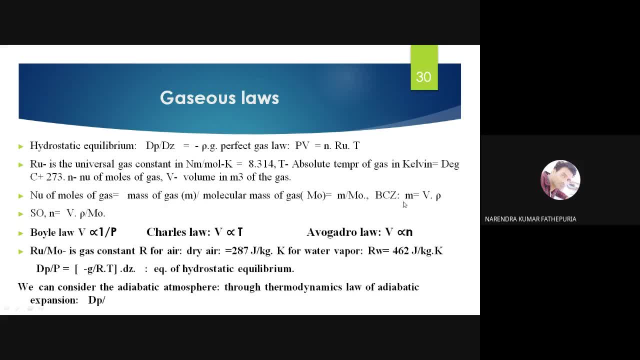 So small m divided by capital M. Small m divided by capital M, So generally small m will be the V into rho And you can write it in the final form And number of moles of gases will be. you are getting in. These are the three laws that we speak, that we talk in the gases forms. One is the Boyle's. 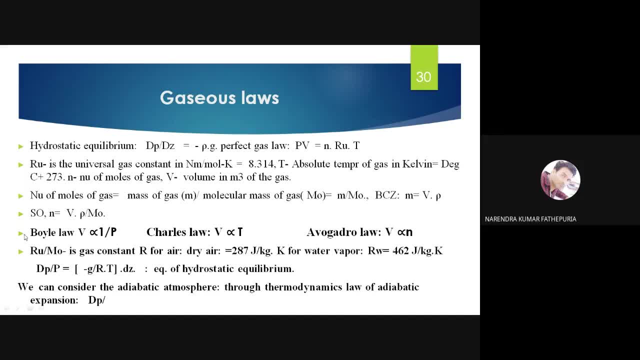 law, Charles' law and Avogadro's law- And the Boyle's law says that all laws are talking in terms of volume, in terms of pressure. So the Boyle's law always says about the pressure and volume. And then Charles' law says volume versus temperature. And Avogadro's law says: 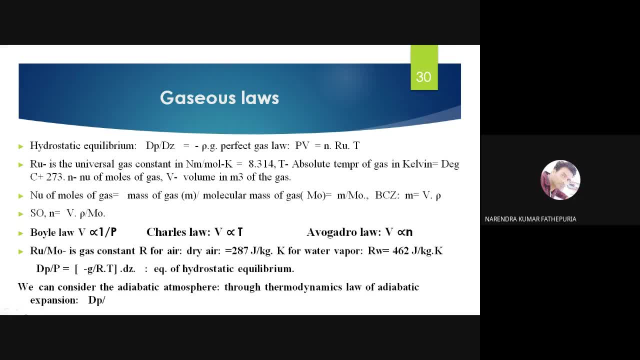 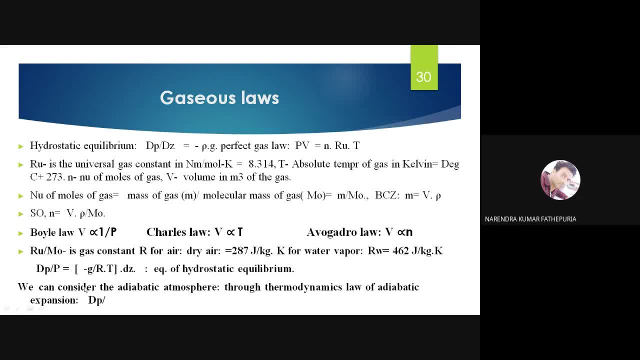 So I'm going to try and find out where the gas constant is. this is the temperature level Now, if I look at the pressure taking up, so it's probably at the 3.5 G Joule per Kg in Kelvin. for the water vapor, Rw will be 462 Joule per Ks in Kelvin, So this 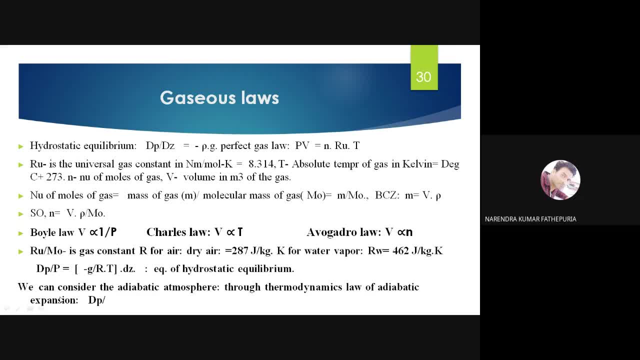 is the standard equation. If you go for the, PV is equal to RT. we use it. If you put all the, then we'll be getting this form. This is called kind of static equation: Tp by P is equal to minus, minus rt into dz, So we can consider the adiabatic. 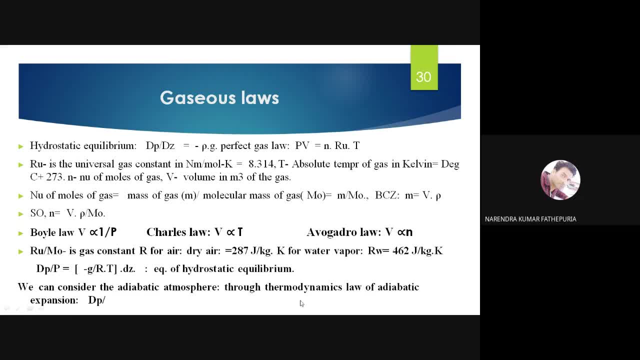 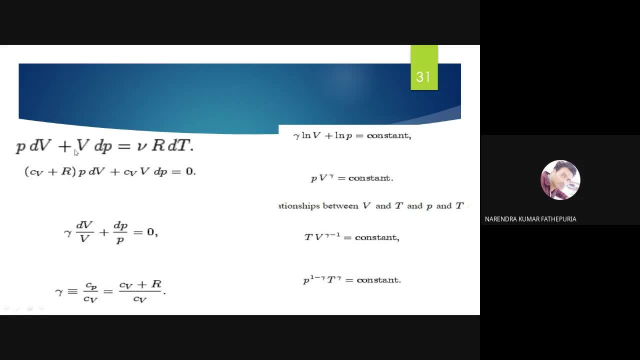 So adiabatic lapse rate, we will take it through the thermodynamic law of adiabatic expenses Coming here. So this is the general calculation. PV is equal to RT and then derivative with respect to dv and volume. right pressure p into dv plus v into dt is equal to v into 1 into dt. 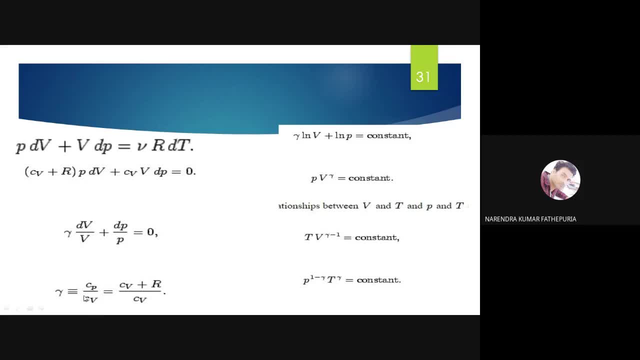 if you go for it, How do they solve it? This is the specific heat at constant pressure and specific heat at constant volume, Cv by Cv. So dv plus R divided by Cvd is the normal, we can say the derivation that you have multiple. 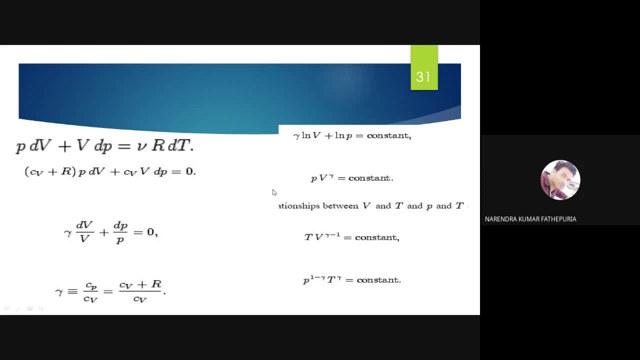 times done it and then you know the standard values for gases loss. So if I am talking about the adiabatic conditions, so there is adiabatic conditions are locked in. different PV to the over. gamma is equal to constant generally for the adiabatic conditions. 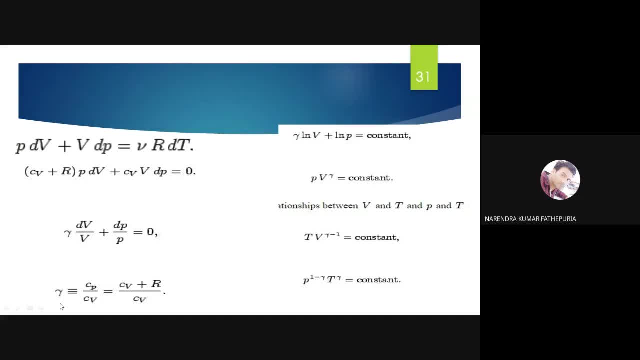 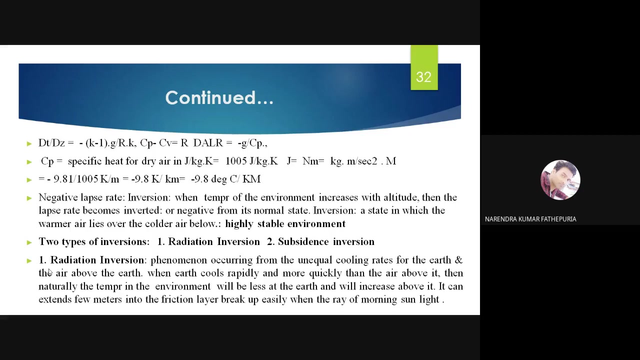 So gamma is the gases constant. There is a p relation- 1,, 2,, 3, as well as this one. So it is important and that is also important. So Also to that question: Okay, Okay, some. 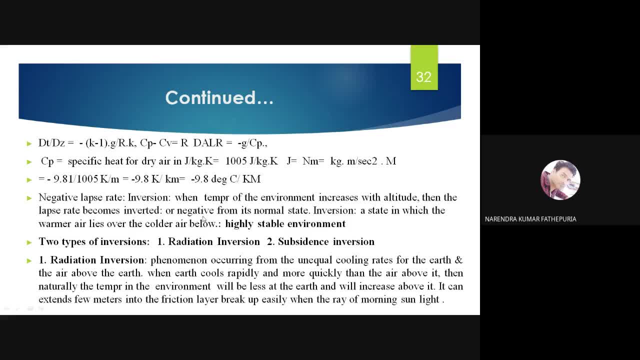 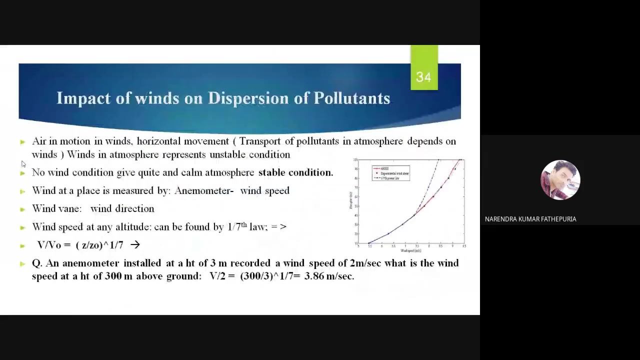 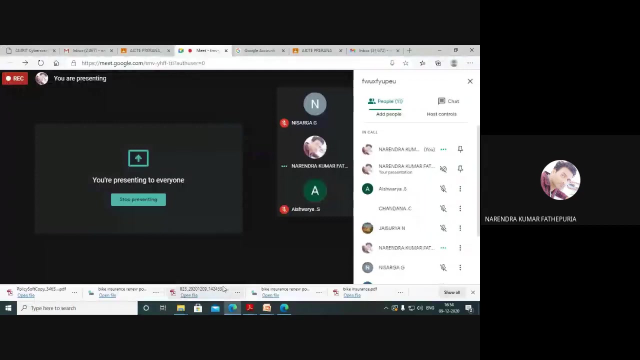 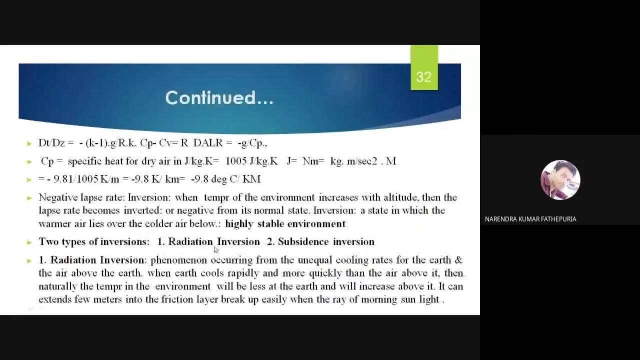 you, you, yeah, let's go disconnected. so here, yeah. so here these equations. you can do it. I have already calculated notes for this. we just try to solve the questions and go for the series, also gate series. we have hardly one month for gate exams now, but basic. 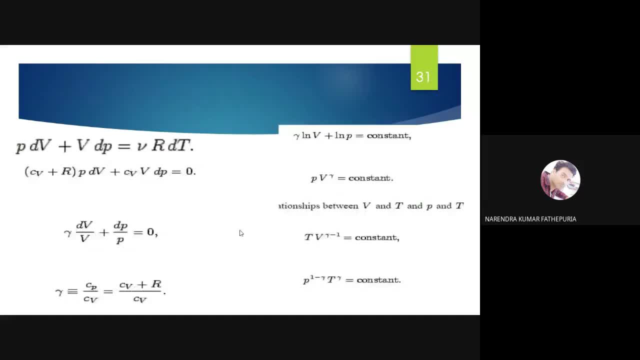 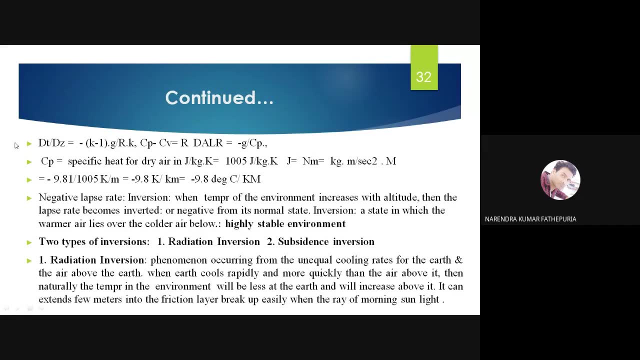 query part and basic equations, derivations. I have explained everything and standard equations that is used. we just go through these numericals and then try to solve it. so once you go through these slides and air pollution slides, you will be getting enough confidence for attempting the question. 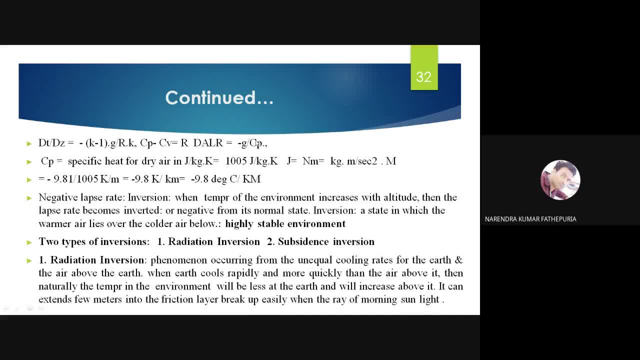 okay, related to gases. okay, so this is the formula for d minus g into c m g by c p and then you can do it, which will be: if you want to convert into k g s and k g into meter per second square meter and conversion you can. 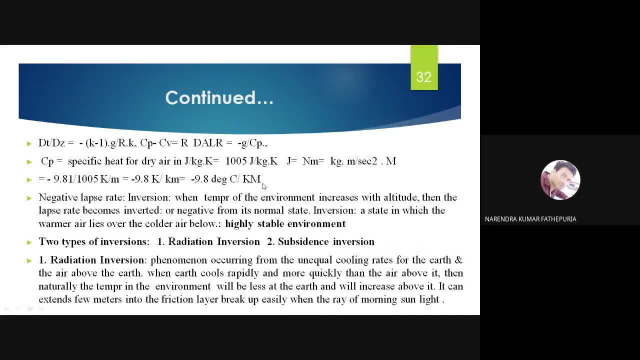 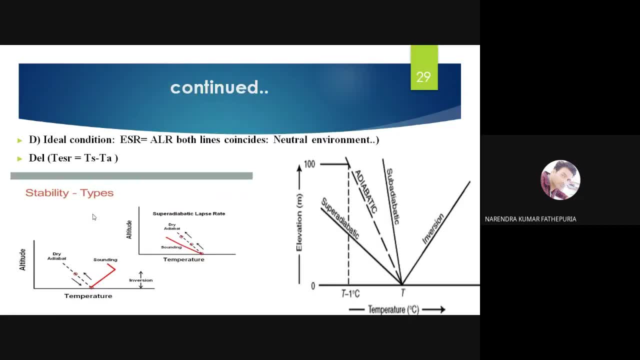 do it and finally you will get minus 9.8 degrees per kilometer. now you are talking about the negative lapse rate. yeah, inversion, that is very important. so there's a fourth type, as I told you. okay, the another thing is del t s? r sometimes, 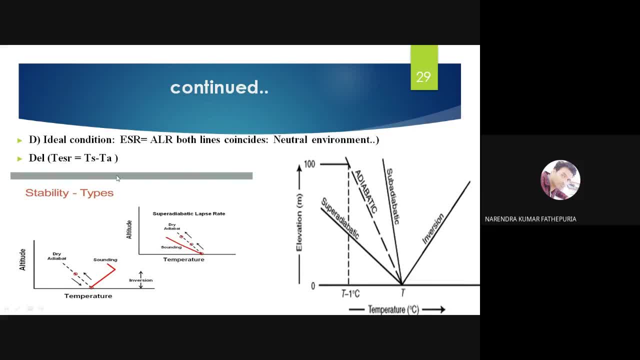 there is two temperature given in the question. temperature for t s and t a will be given, so higher minus lower. if you can do it, you will get. the temperature for the e s r e l? r environmental lapse rate will be equal to the ratio temperature graph. 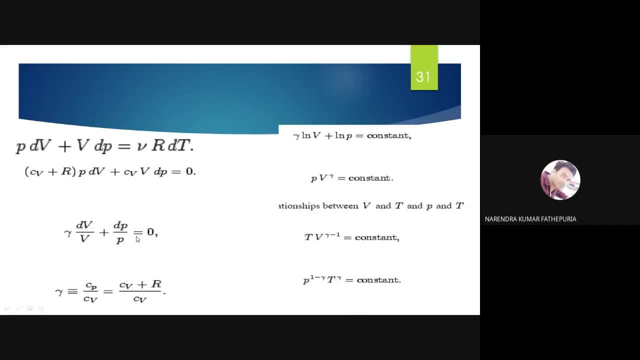 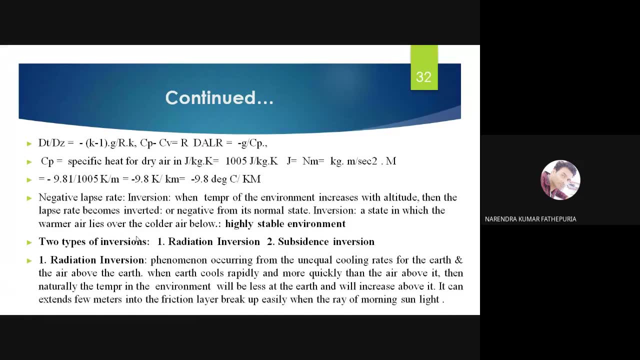 so this, you can get this okay. so there is basic equations you can solve. so inversion: what is inversion? when the temperature of environment increases with altitude, then the lapse rate becomes inverted or the negative from its normal state. inversion: it's a state in which the warmer air 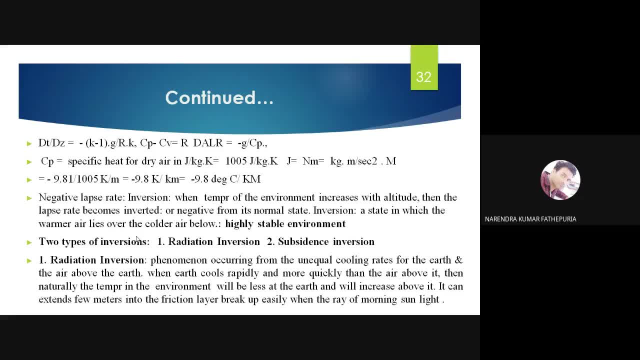 lies over the colder air flow and higher stable environment, highly stable environment- and it is very bad for the pollution dispersion. there are two types of inversions. one is the radiation inversion number. second is subsidence inversion. there are two types, mainly so. first we will talk about 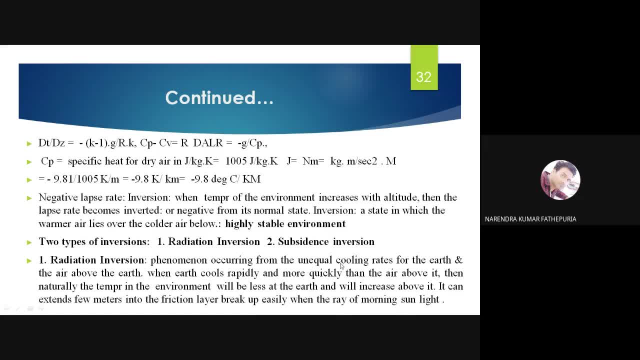 the radiation inversion, this phenomenon occurring from the unequal cooling rates for the earth and the air above the earth. when the earth cools rapidly, the more quickly than the air above it, then naturally, the temperature in the environment will be less at the earth and will increase above. 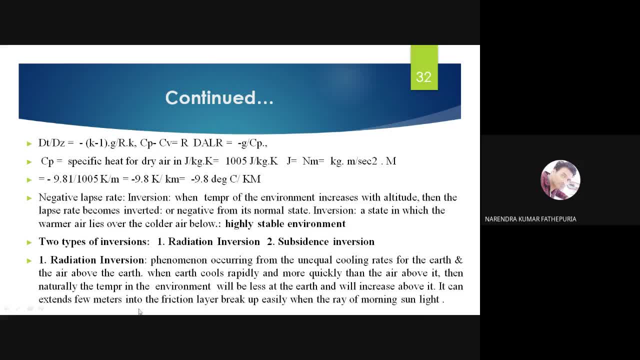 it. it can extend few meters into the friction layer, break up easily when the ray of morning sunlight comes. so this phenomena is having a certain temperature ranges and generally on the surface temperature rises and this phenomena occurs early in the morning. this radiation inversion occurs in the morning. 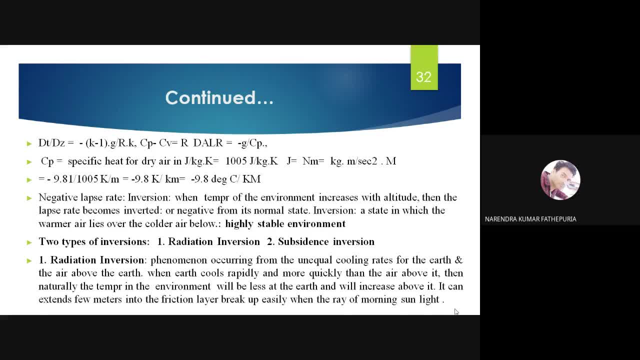 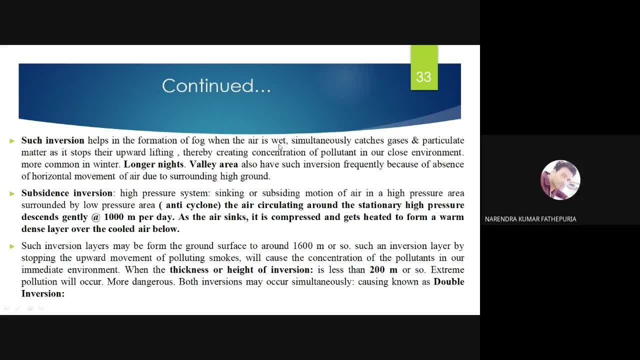 and morning, it can easily break this layer. so, yeah, such inversions. such inversions help in the formation of fog. when the air is wet, simultaneously catches gases in particulate matters, as it stops their upward lifting, therefore creating a concentration of pollutant in our close environment. 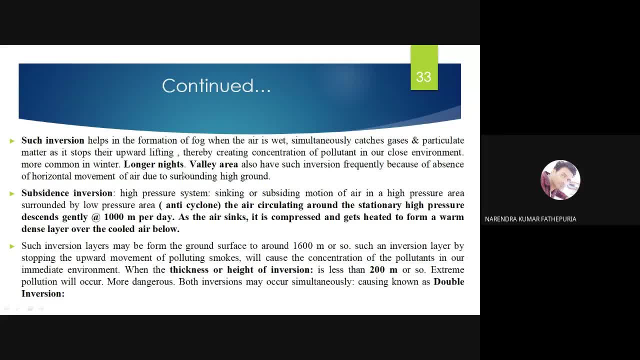 more common in the winter: longer nights because of the longer nights in the winter. in the valley areas also, this practice is very common. radiation inversion is very common in valley areas. what will happen? also have such inversion, frequently because of the absence of horizontal movement of air due. 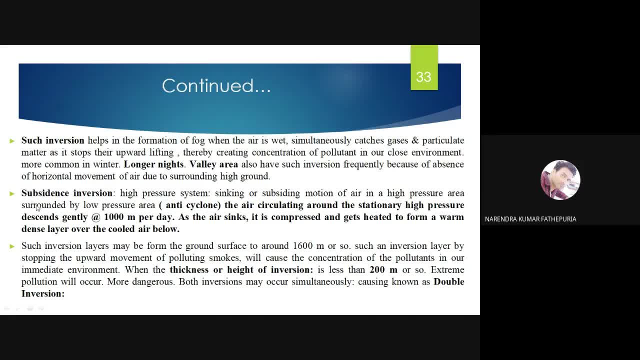 to surrounding high ground. okay, so that is the technique. then this is the process inversion and then second is the subsidence inversion. it happens at high altitude, high pressure system sinking or subsiding motion of air. in a high pressure area surrounded by the low pressure area, there is 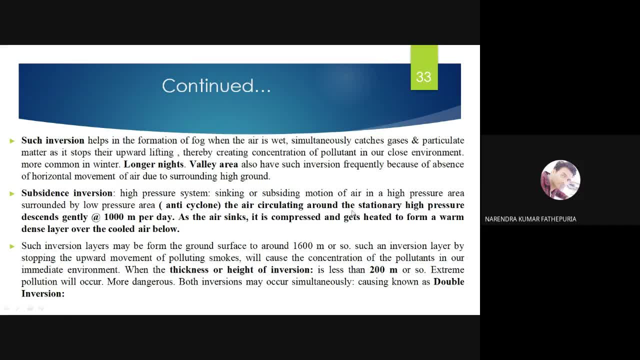 an anticyclone which the air circulates around. the stationary high pressure descends gently at 100 meter per day. as the air sinks, it is compressed and get heated to form a warm, dense layer over the cold air flow. so there is a cold air and 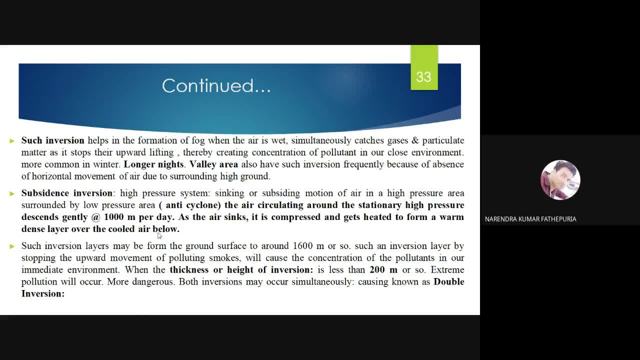 warm air and because of the wind speed, because of the temperature and pressure profile is different for the particular area and these conditions okay. so generally anticyclone conditions, such in politics, will cause. the height of the inversion is less than 200 meter or so the extreme. 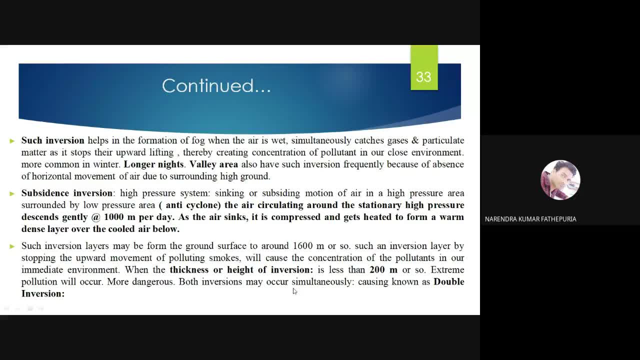 pollution will occur more dangerous. both inversions may always occur simultaneously. sometimes so well in the world. but for a first step in work, please the person to take place together simultaneously, and this condition is called as double inverse. all conditions are adverse for the environment. it is not. 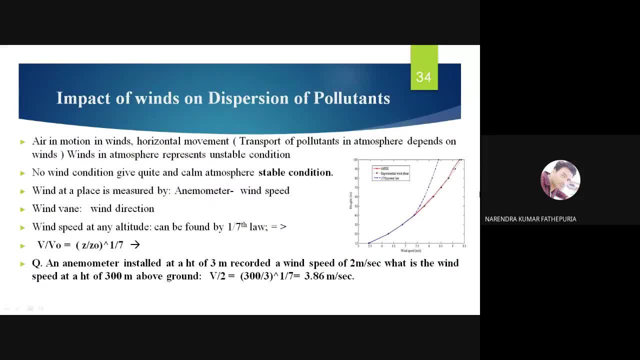 good for the pollution, of pollution we want, the quickly the pollution and particulate matter does and all the pollutions, so this person, so I should be clear now. second is the impact of wind or dispersion pollutants, this environmental, let's see it in everything we are studying. 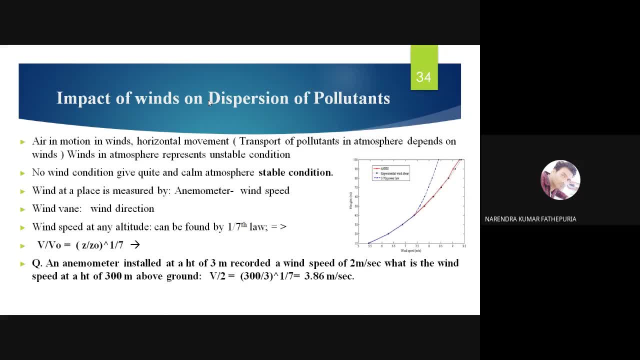 second impact we have for the direction. wind defeat play a very important role in that there is a wind rose diagram for this analysis, for the wind rose diagram. through this, the meteorological department, the weather and wind, this wind defeat and all that right. so the of the 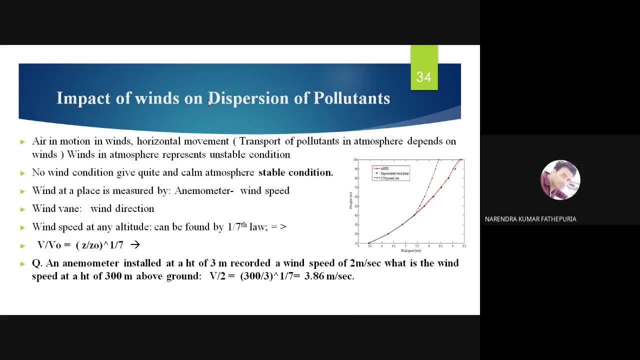 atmosphere, as well as the pollutant dispersion right, how the pollutant is released from the particular industry. so I will be talking about the various types of plume. okay, generally the air and wind, horizontal movement, transport of the pollutant and atmosphere depend on the wind. if 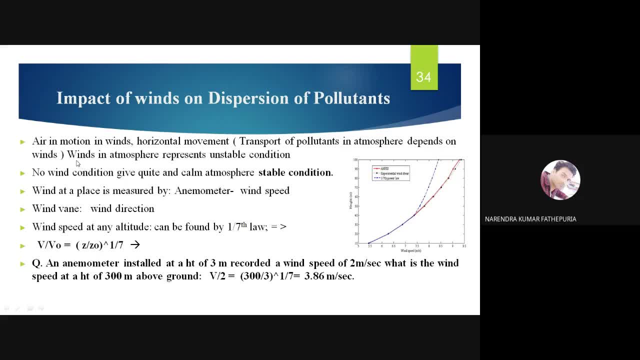 there is no wind, then pollutant will not disperse, so it helps in dispersion of pollutant and wind in atmosphere represents unstable conditions. no wind conditions give quiet and calm, stable, very harmful for the atmosphere, for the pollution, pollutant dispersion. wind at a place is measured. 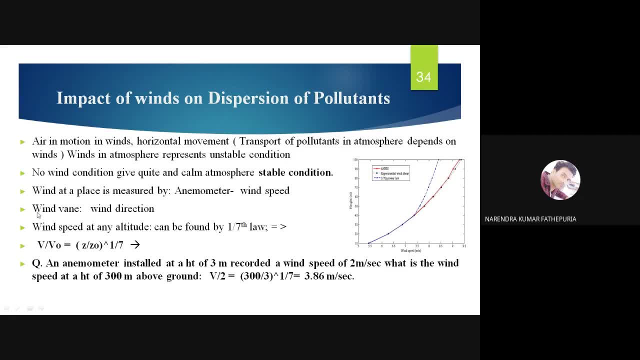 by anemometer. there is a device called anemometer which will measure the wind speed. there is a wind vane also wind direction. on which direction wind is going? that? also through the wind vane, you can measure it and there is a wind speed at. 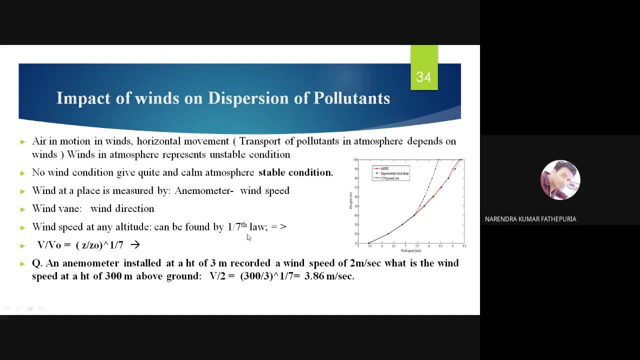 any high altitude can be measured by the 1 by 7 law. there is a 1 by 7 law in wind speed measurement, which is will be equal to b by b, not is equal to z by z, not to the 1 by 7. 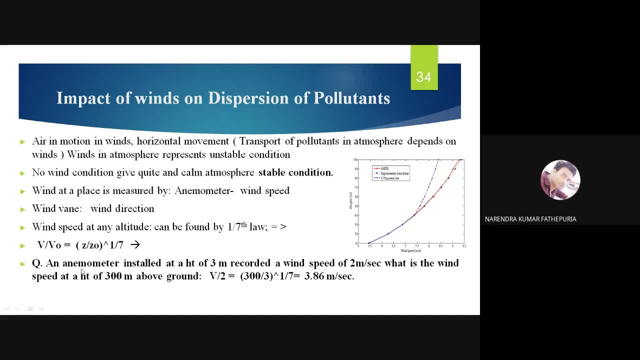 this law is called as 1 by 7 law. sometimes they ask great questions. suppose you have given 2, 3 equations here. so this is the 1 by 7 law for measuring the wind speed with respect to altitude. so suppose in an anemometer. 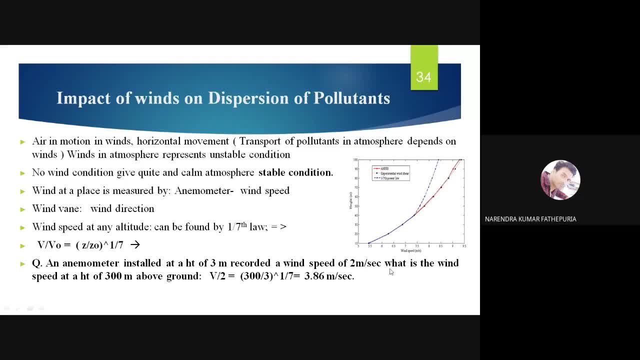 installed at a height of 3 meter, recorded a wind speed of 2 meter per second. what is the wind speed at a height of 300 meter above the ground? so just use this equation and get that so v by 2. 2 velocities are given. 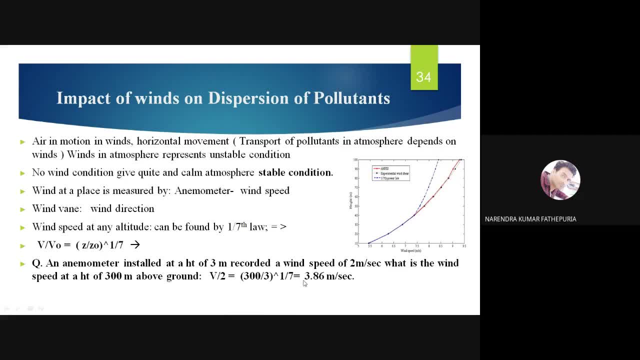 divided by height, altitude is v. you are getting it so recorded at a 3 meter height recorded wind speed. is there? what will be the recorded wind speed at a 300 meter height, so that you have to use this relation and you get the height at anywhere? 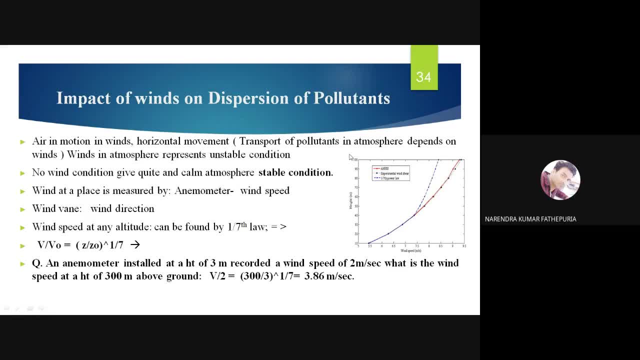 along with this altitude. so this is the wind speed we have taken on x axis, and height we have taken on y axis. so this is the graph. you are going to plot it right. so this is the 1 by 7 forward law through this blue lines. 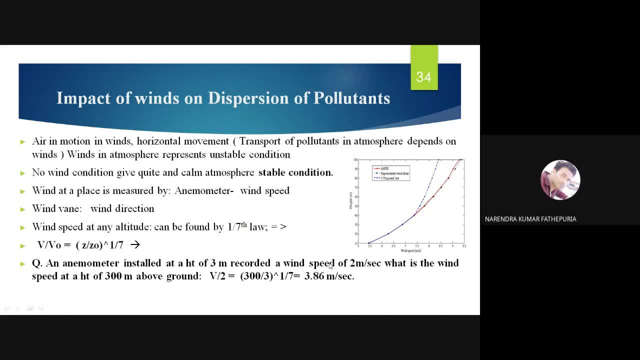 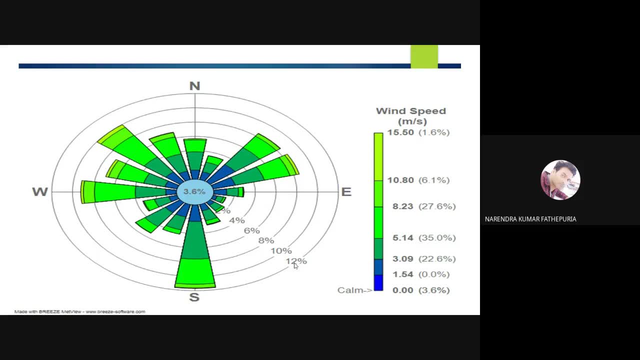 anywhere you can get it. the wind speed: you can measure it by using this equation. now we will be coming for the wind rose diagram, which is very important. this is the wind rose diagram, wind speeds generally, the forecasting, where the forecasting and these metallurgical department used to. 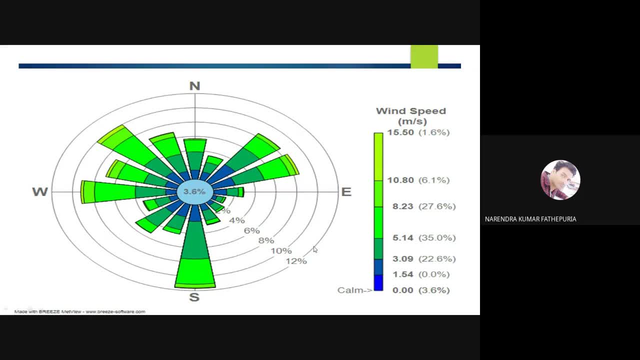 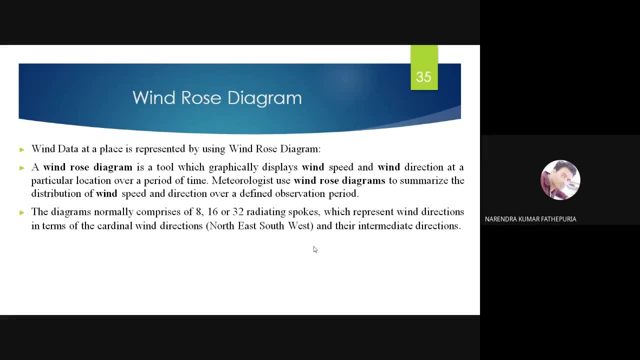 go for it okay. so the wind direction, speeds and everything we noted down through this wind rose diagram. so wind data at a place is represented by using the wind diagram. wind diagram is wind and wind direction at particular location over a period of time. meteorologist used wind. 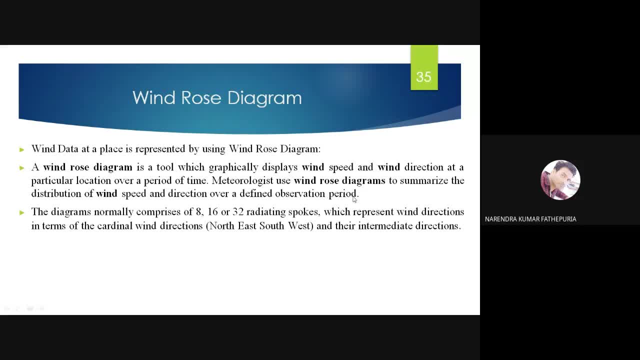 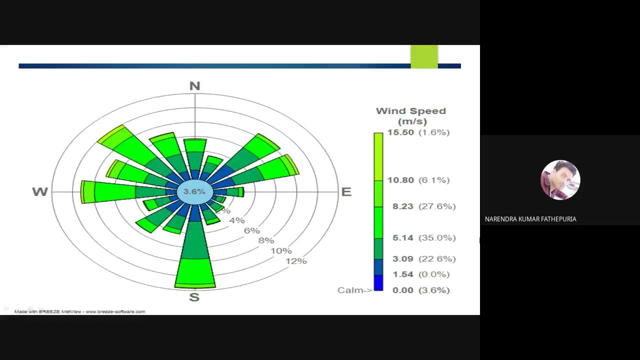 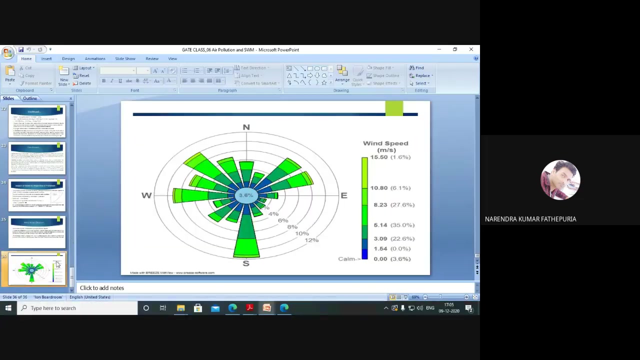 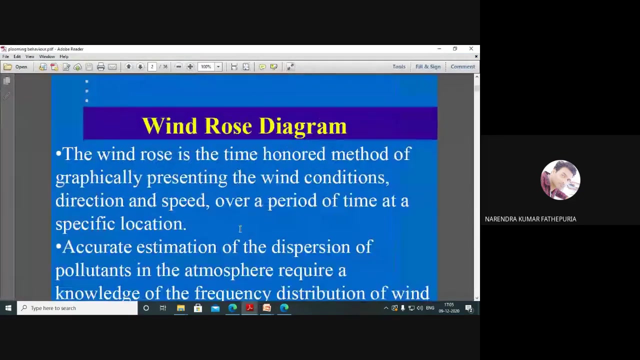 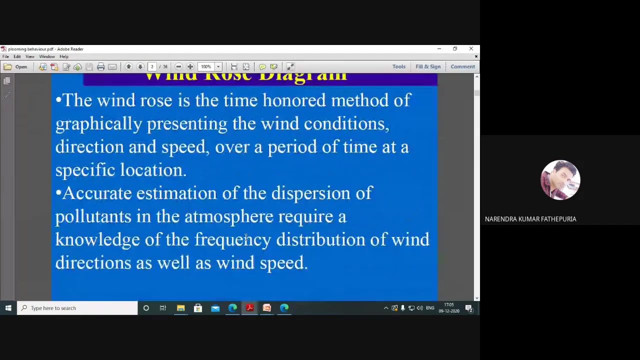 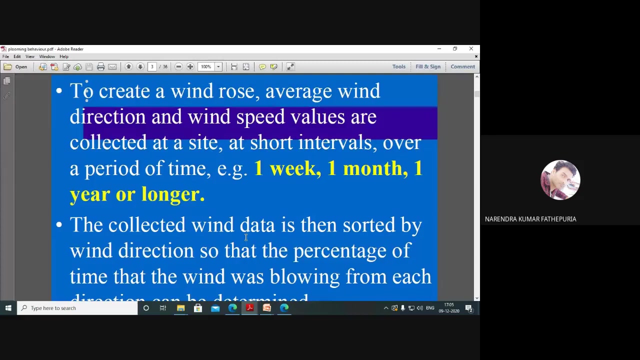 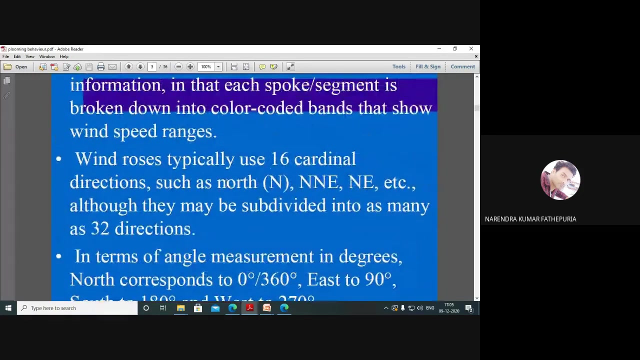 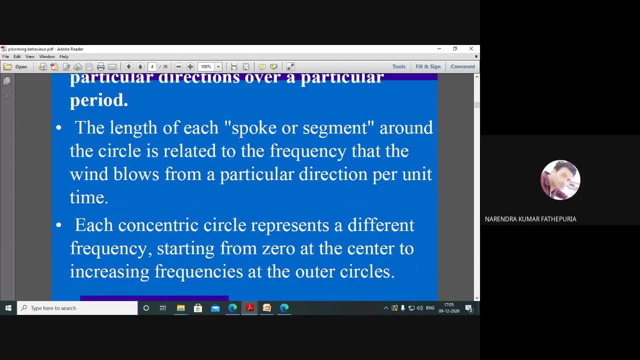 diagram to summarize the distribution of wind speed and direction over a different direction. to find observed observation period, the diagram normally comprises of eight, sixteen or thirty two radiating spokes, which represents wind directions in terms of cardinal wind directions, like north, the direction for you for segment each. 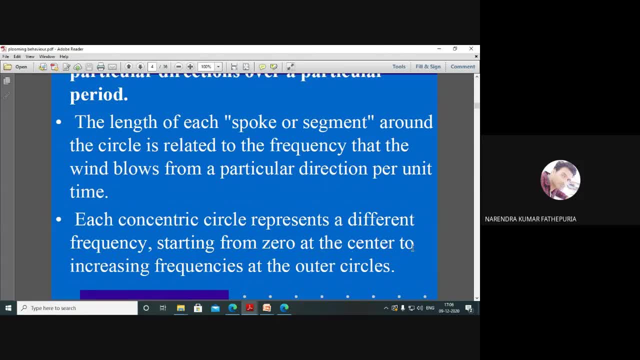 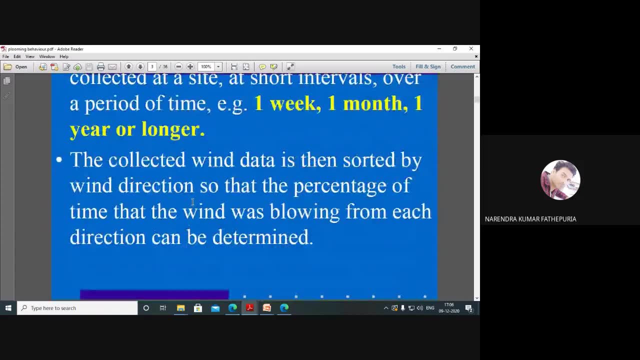 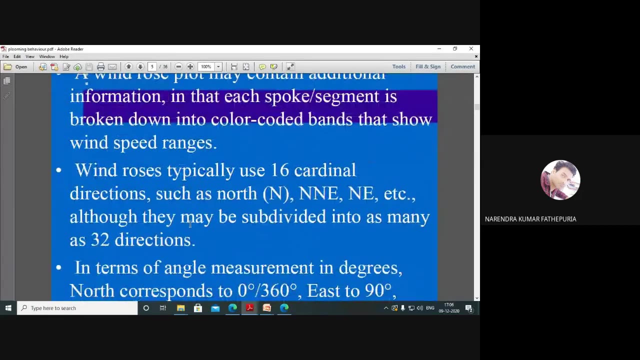 concentric circle represents a different frequency, starting from zero at the center to the increasing frequency at the outer circle. there's a mechanism, there's a systematic procedure for drawing this diagram using those diagrams. so we've been talking about north, north, northeast, northeast, etc. like the sixteen. 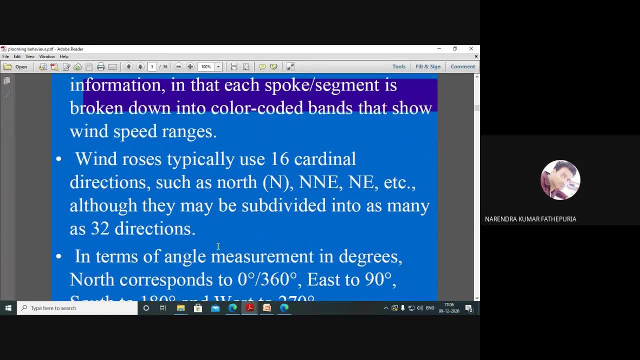 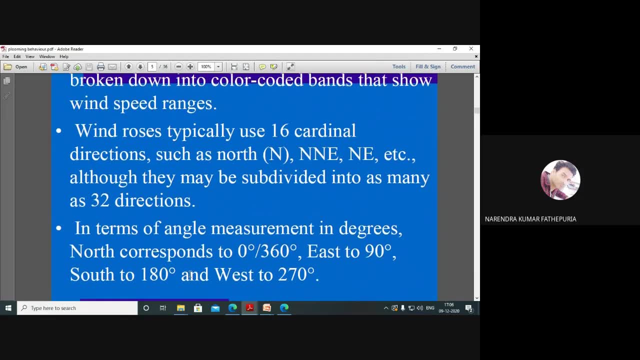 combinations, although they may be subdivided into as many. thirty two directions in terms of angle measurement in degrees: north correspond to zero by thirty three sixty degree, east to ninety degree, south to one eighty degree and west two to seventy degree. so we have to, based on this, 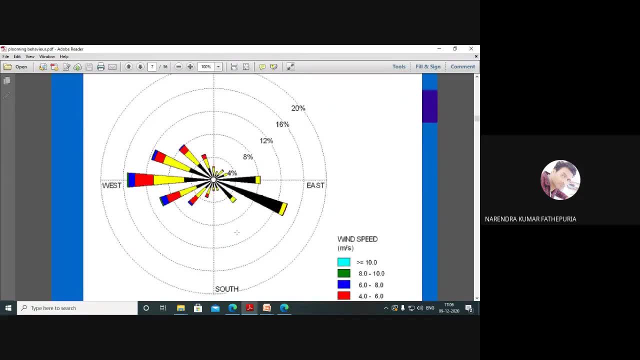 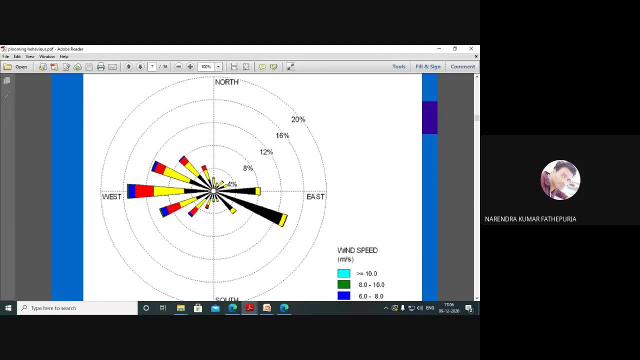 there's a scale and then we have to plot it. in gate exam they will not ask for plotting and sketching this and all that thing, the simple concept they will be asking. so this is wind roll diagram here. percentage is given in this box a four percent. 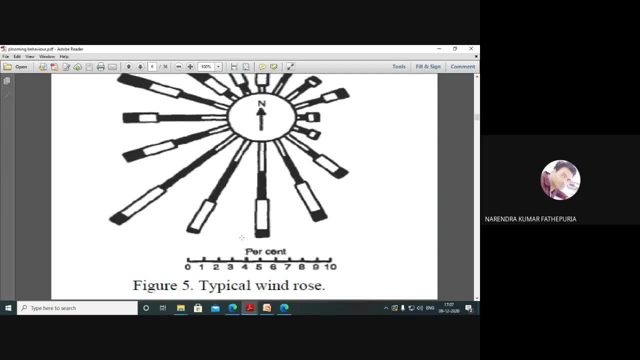 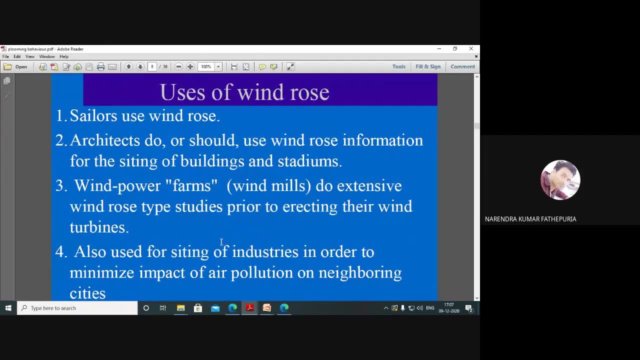 eight percent, twelve percent, sixteen percent, twenty percent. right, so typical wind diagram. uses of wind rolls are very effective. sailors use wind rolls from Portugal and England is, by another, much desperate idea to throw into the switch in. Goodnight be merry and anxious, are you with me, good? 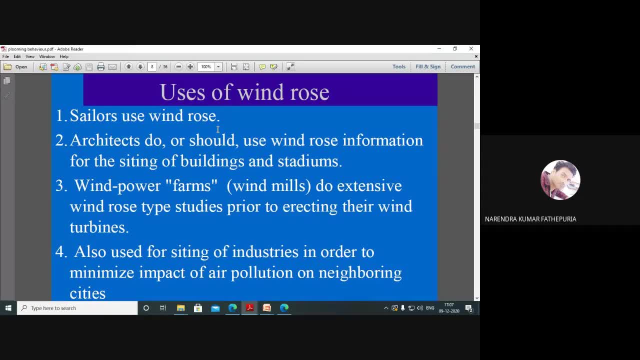 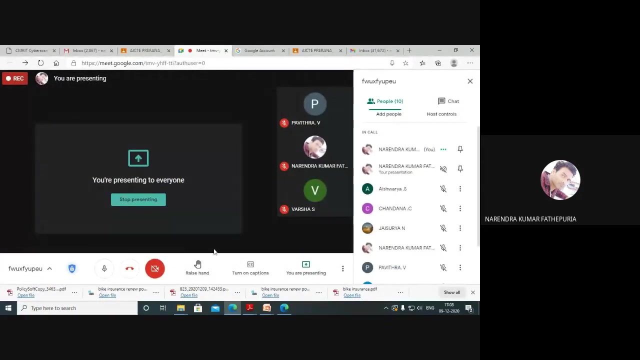 I thought that we have made up you. is this audible now? Can you hear me, Pavitra? can you hear me? Is this audible now? Can you hear me? Yes, sir, Now can you hear me? Yes, sir. Okay, So this is the wind rose diagram. 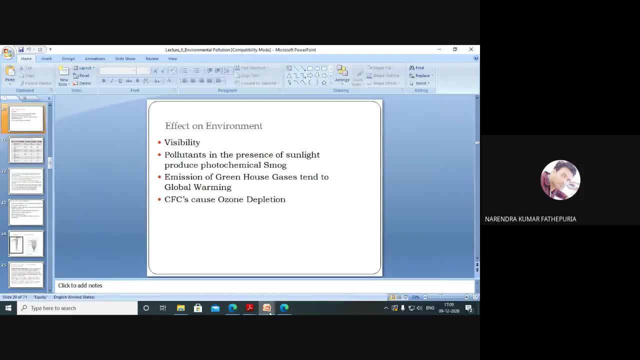 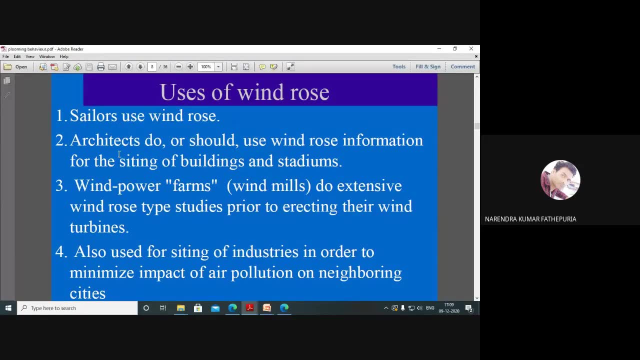 we are talking, So same as using this architect, which was also used in this project, giving the near graphic version which we have drafted now, where the pirates are using their function to make this case and the production is coming up, and this is what we are trying to do. 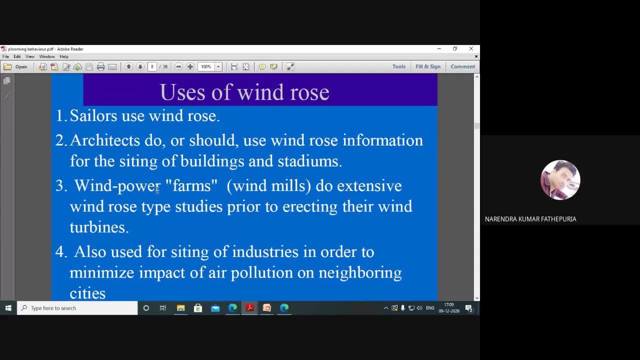 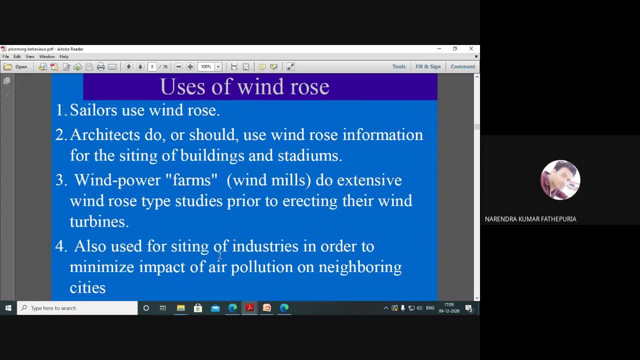 So that will come to you, So we will cover forms with these, with these tips and tools that we have used in this project, and we will talk about this. So, first thing, we will first add in the most important thing, which is not only the. 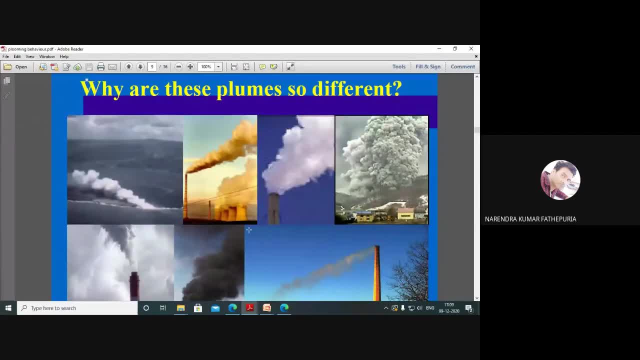 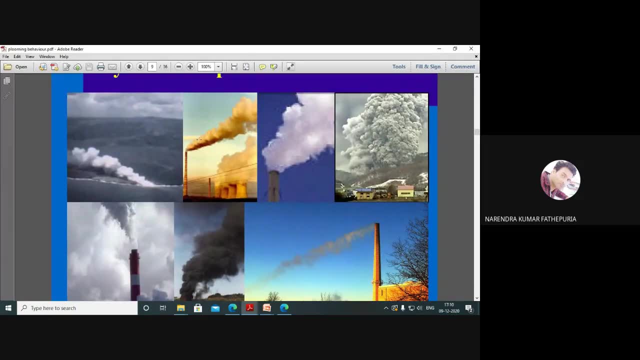 print, but also the process. Now I will talk about the prints. These prints are very important. Prints is nothing but a piece of paper. On the strip of the print, this position is this person. there They are. this snow is making its own path there. This path is called as: 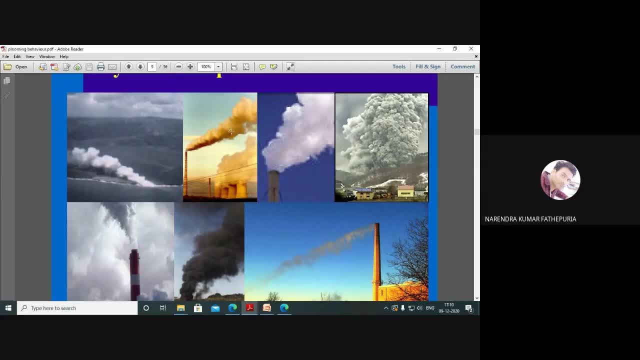 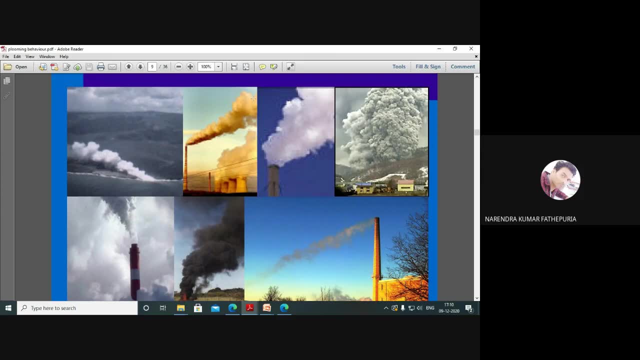 the print position. So in what direction? which print path will be going for the position of this person? So suppose he has in that there is a print which is giving a which is in this, this direction. Sometimes this print is going on the upper direction, right? 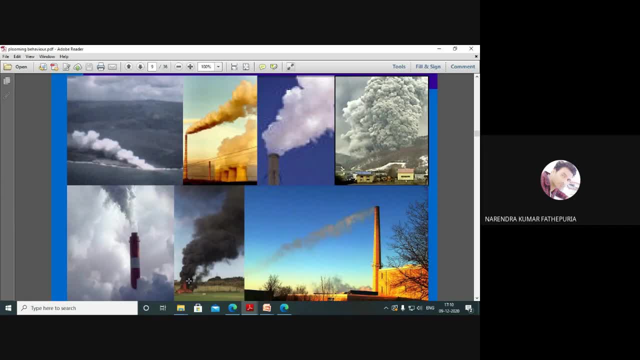 Sometimes the print is directly coming towards the lower direction. So it depends what type of sleeve that smoke is pouring while it is dispersing, while it is releasing from the shape of the print. That is very important while you are, while you are trying to understand, 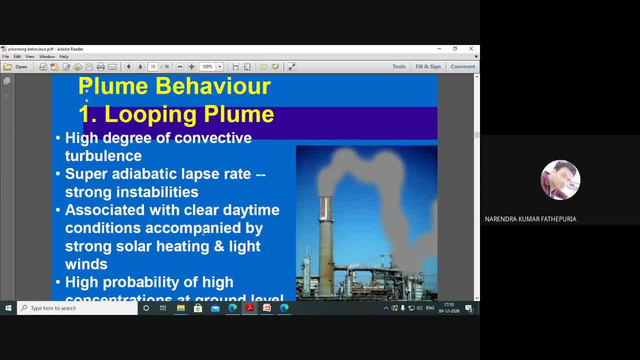 the dispersion of the point. Okay, That is very important. That is what is chrome-chrome behavior. So there are six states that are involved. So there are six states that are involved. So, for example, let us speak about this one. So let us look at this group here. 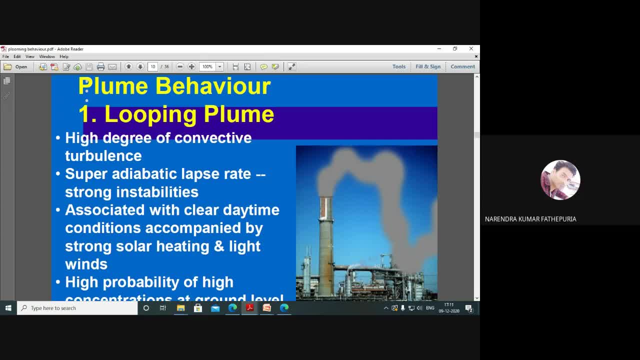 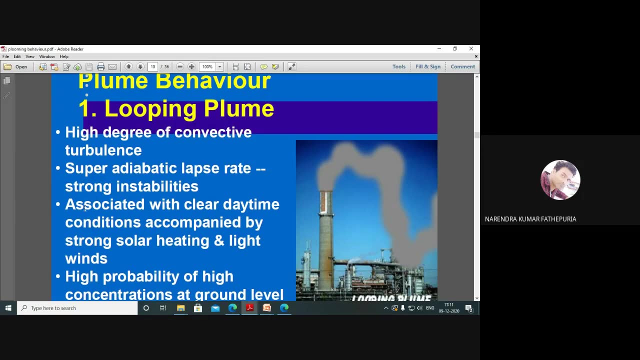 One is the grouping group. This is the grouping group which is made by the. once this is released, on the strip of this, The slope is released that in this case there is a different grouping group: The aggregated, super-aggregated здесь. this is strong study of this. This. 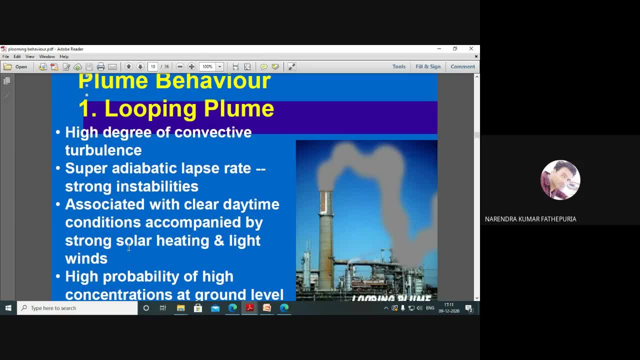 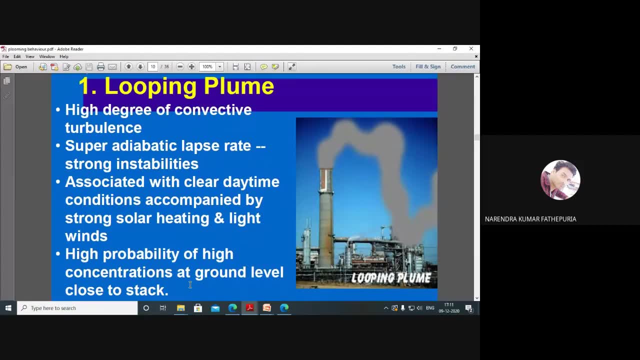 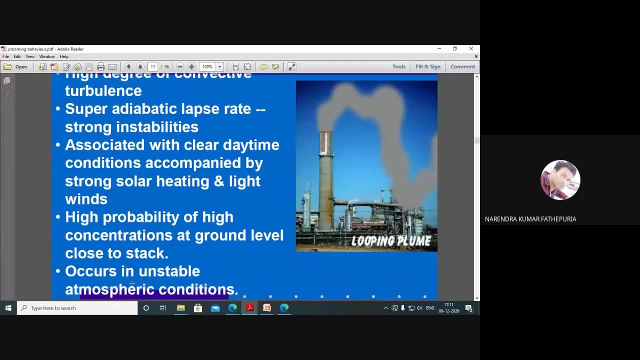 here is clear data analysis accompanied with a strong solve here, Making this all in the High probability of high concentration at ground level close to state. So high probability of high concentration at ground level close to state. So a person has a stable rate of atmospheric emissions. 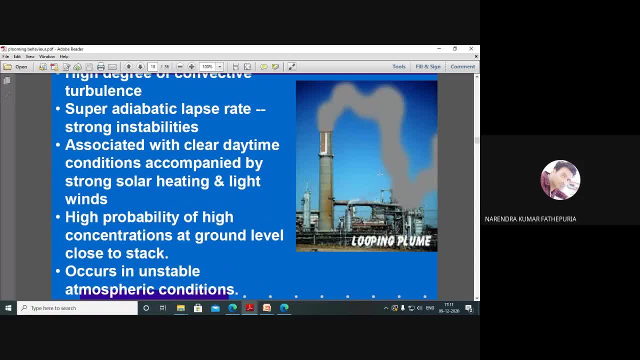 This is called a saluted state And that you have to relate with the adiabatic landscape as well as the ELR system For the stable level, a stable energy flow, as well as the adverse conditions. are there Salutes to behaviour when you think through behaviour? 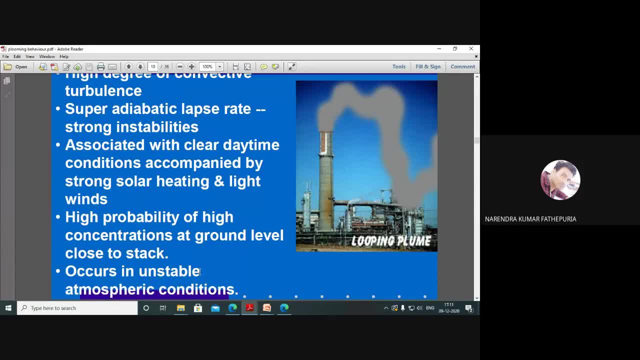 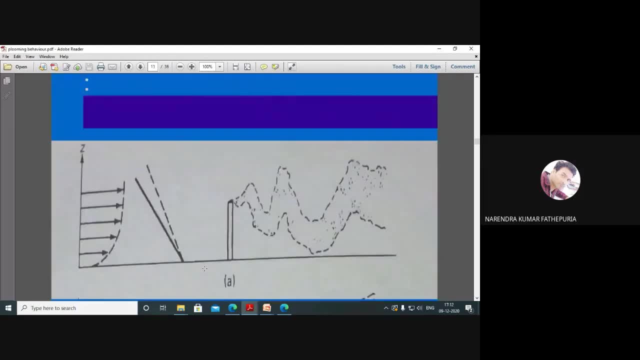 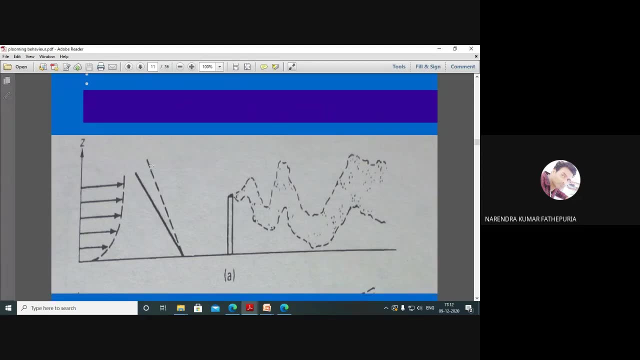 Close to the unstable conditions And that is called an adiabatic state. ELR is related to ESR. ELR is related to ESR. When you say adiabatic period, go back to ESR. This is your ELR current in the left side. 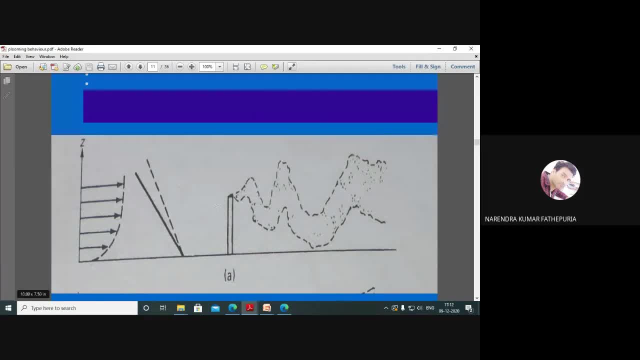 This is the radioactivity in the right side. This is the radiation mass Here, the Here the radiation mass ELR is greater than your ELR in the left side. ELR is related to the adiabatic landscape. ELR is related to the unstable condition. 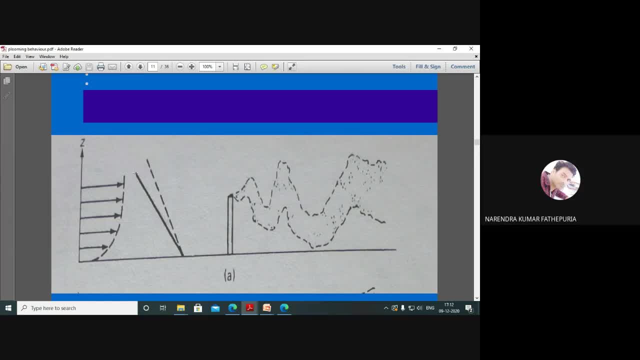 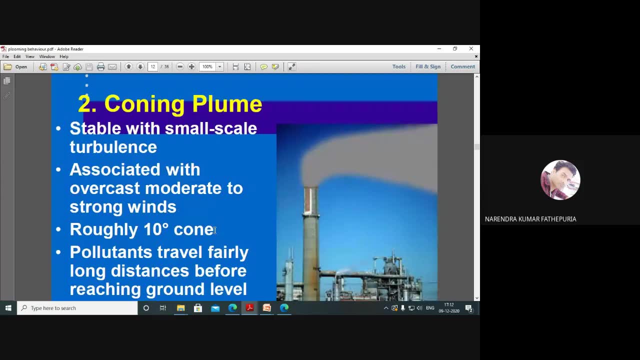 So ELR is different in this. So this is the unstable condition, That is the behaviour in that case. This is what we call an adiabatic state. This is the idea as well. Second is the conning phase. 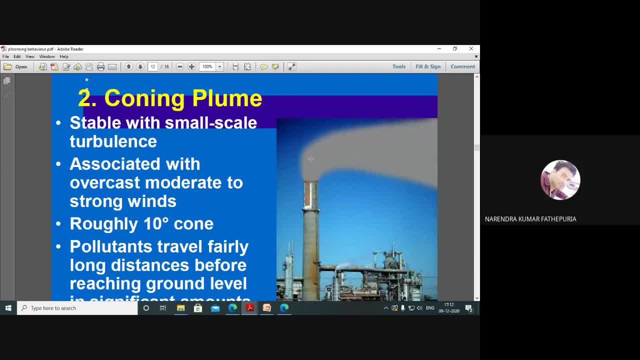 This is the con. The con say: once the collision is discovered, it is released from the state of the city. It will go into a clear behaviour, A coning behaviour. It will form a coning section, A coning section. 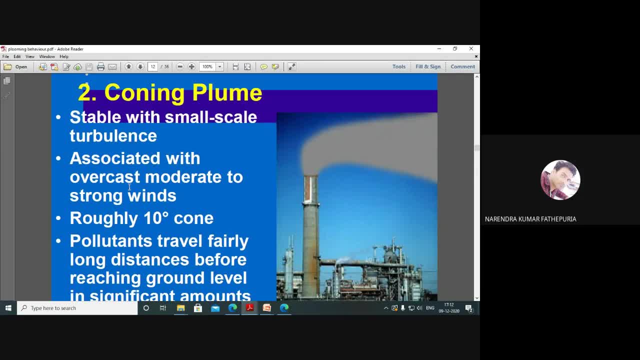 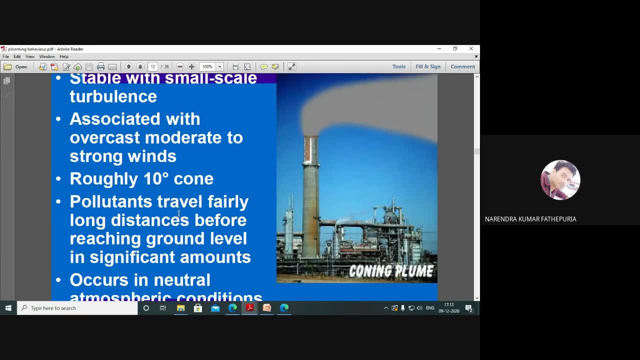 This is the condition. This is the steady condition for small scale of winds associated with overcast water, Strong winds, Happy 10 degree coning, Coning, con Or. it can travel fairly long distances before reaching down level. Insignificant amount of. 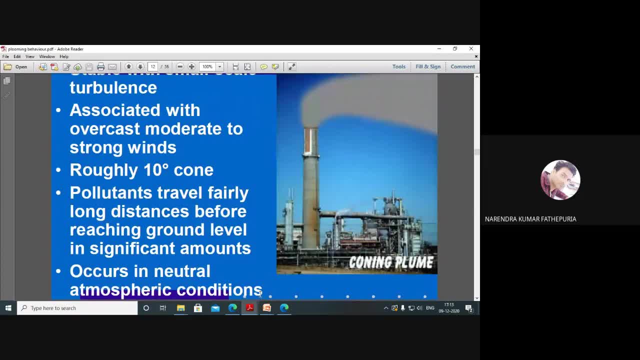 It occurs in a little atmosphere conditions. This is the coning condition. It occurs in a little atmosphere conditions. ESR is required to ELR. Go to ELR, It will be directed. It is the policy direction Polis is directed. 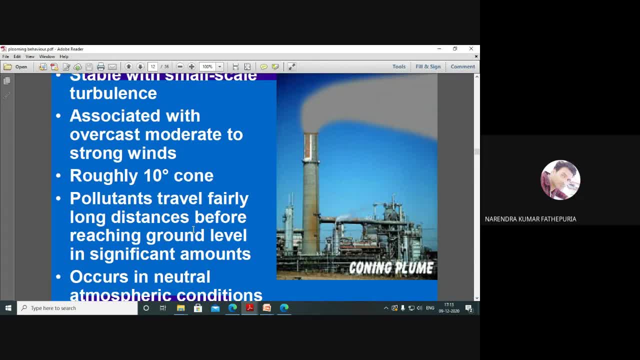 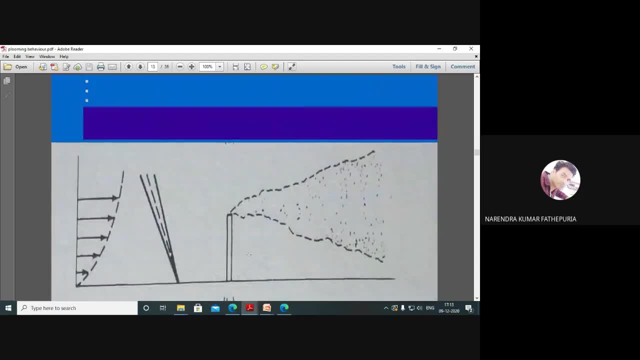 So 10 degree con in thewald status is the condition we will see. This is the coning condition. This is the coning condition. We have the adiabatic left slip Embar относically to right Gaia adiabatic section. 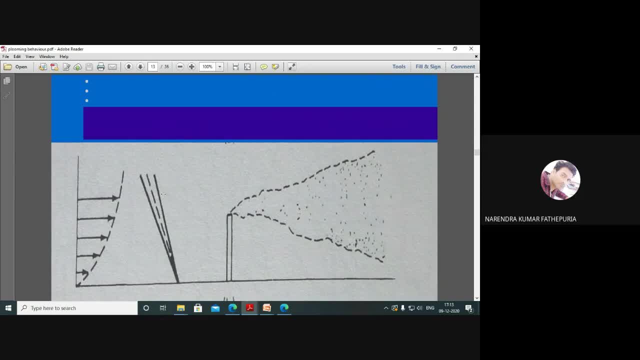 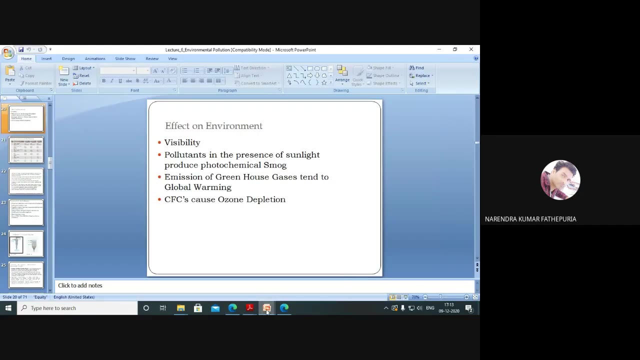 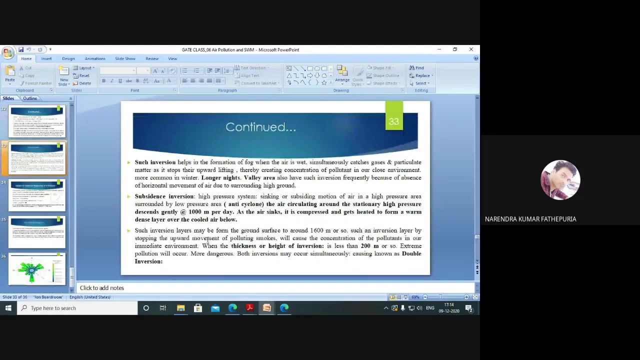 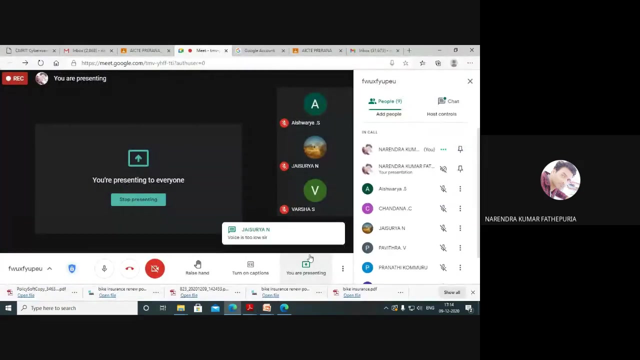 Both these four things Unassembled So that the ELR will not. quantity constitutes, as gone, A neutral condition. What was the condition that we created for the environment? Neutral conditions, Strict, Strict conditions, Strict conditions. What is the state of the environment? 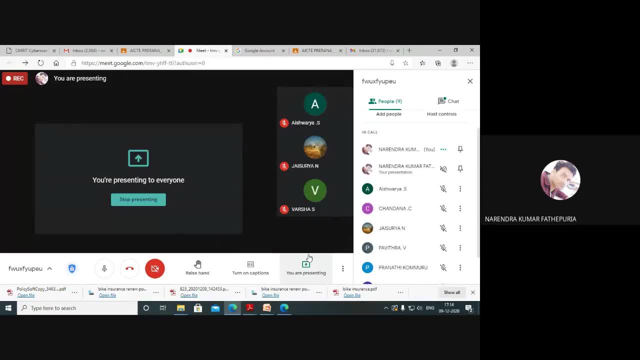 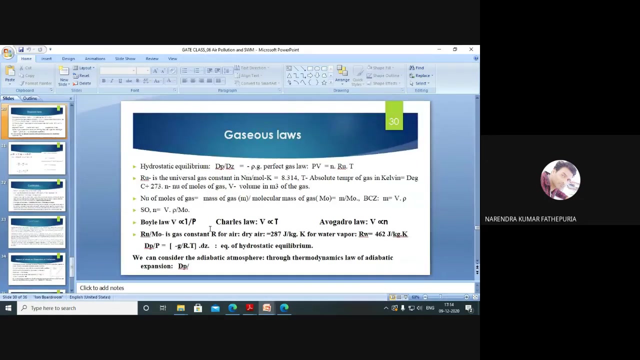 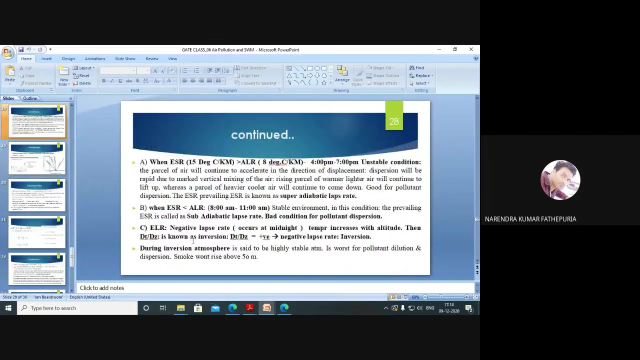 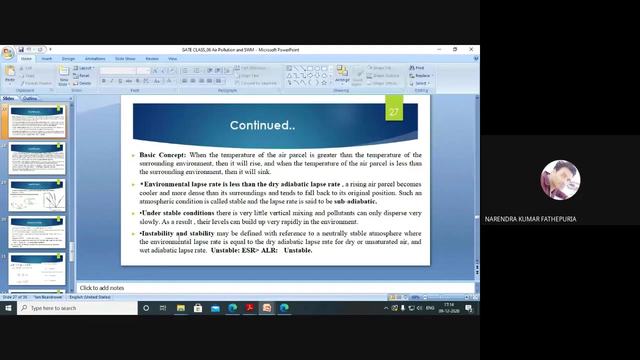 Now it is file, now it is scale. it is just going to write the message. so here we have, under header 1, which is moving around, it is digging out the game. so it is, it is still running. It is still running. 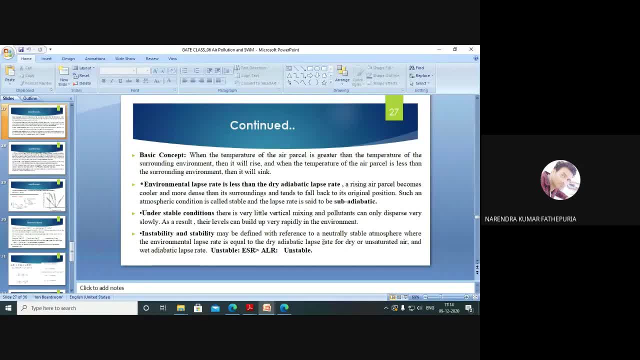 So yeah, so it is, it is still running. So yeah, If we have under header 1, it is moving around, It is digging out the game. Yeah, So it is still running. Yeah, So, yeah, So yeah. 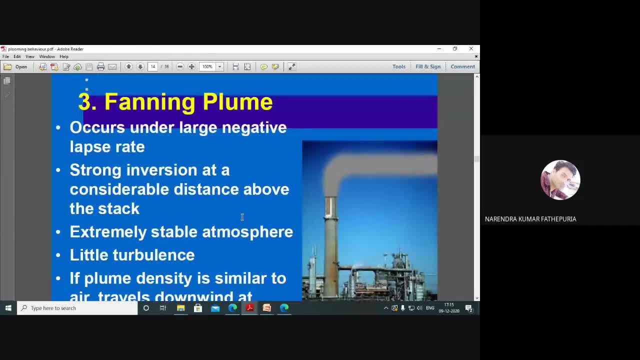 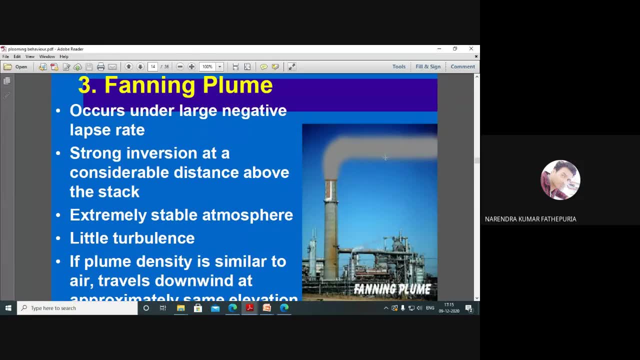 This is the spawning condition in advance of tanning period. this is the plan tanning period, which will be the tanning period. So it will go down this way: T volume, C height: It will go for the certain height of spin. after this it will disperse in a straight causal view. 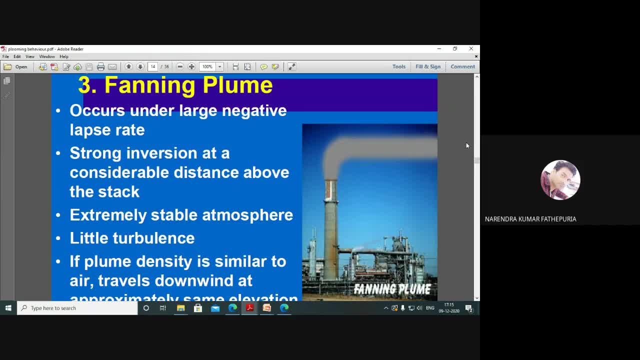 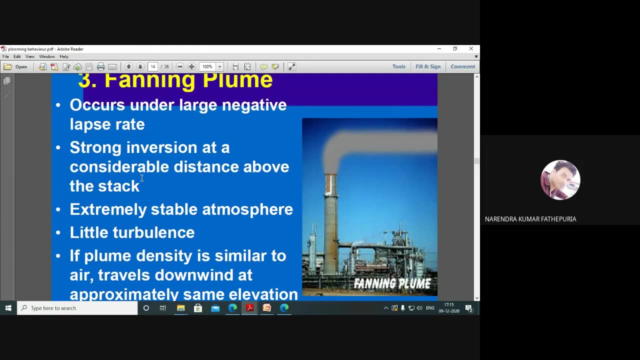 So then, after passing through certain distance, it will go down on the surface, on the ground. So it occurs under the large negative net state conditions: strong inverting at a sensitive distance. That is the state reverse condition for the atmosphere: Spanning period: reverse condition, sensitive distance at the state: extremely stable atmosphere. 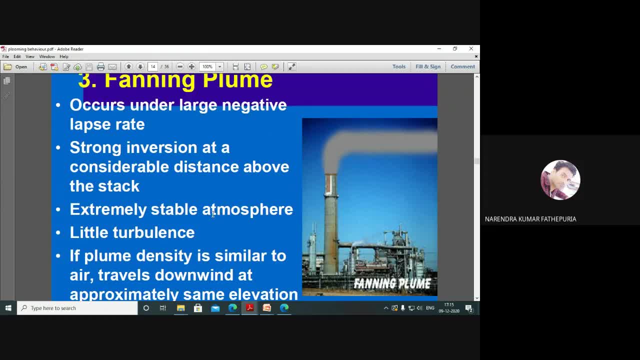 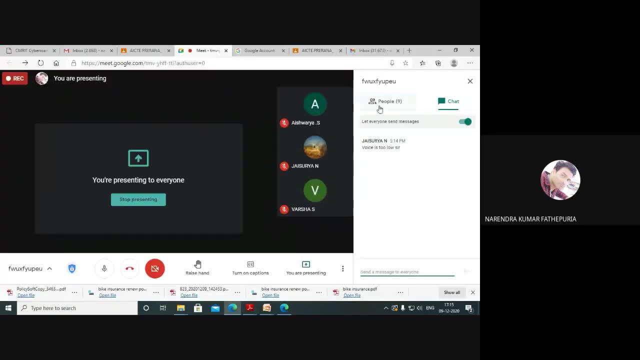 Extremely stable atmosphere. as I told you the position, the stable atmosphere is not good for the environment. The voice is audible now clearly. Yes or yes? Is it clear by voice? This is a tanning session only. goodbye, Thank you. 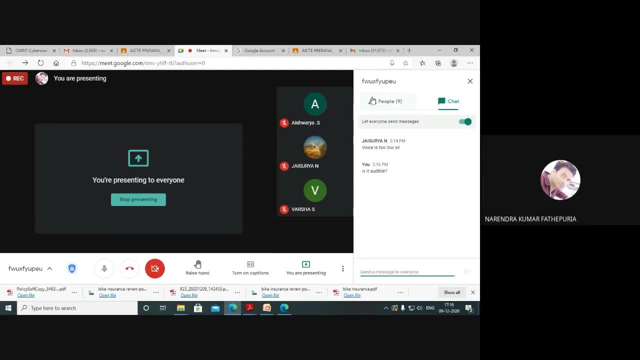 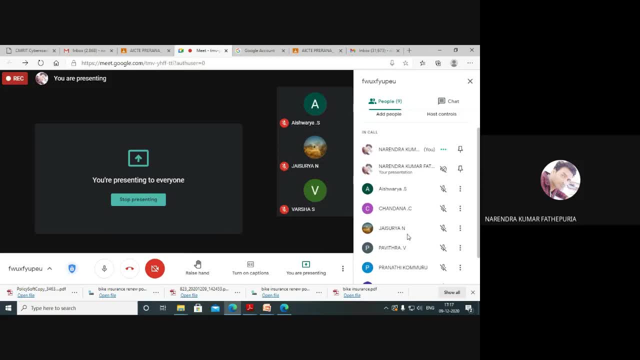 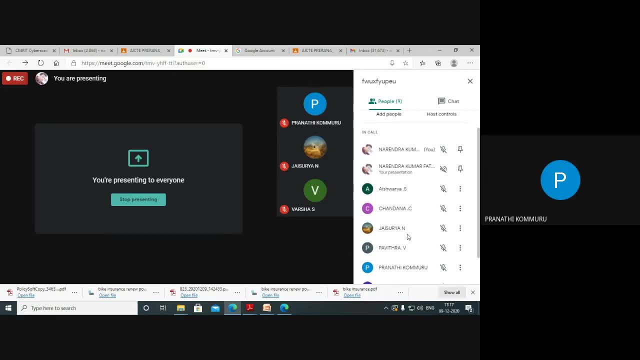 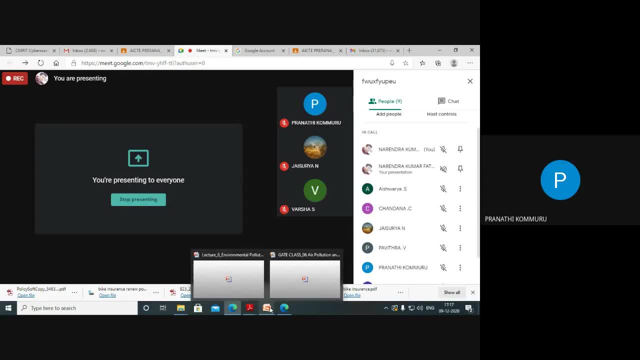 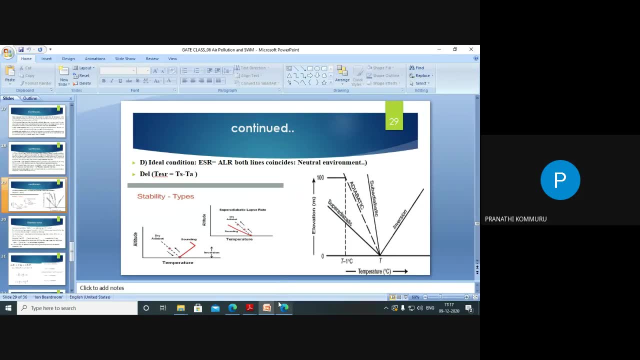 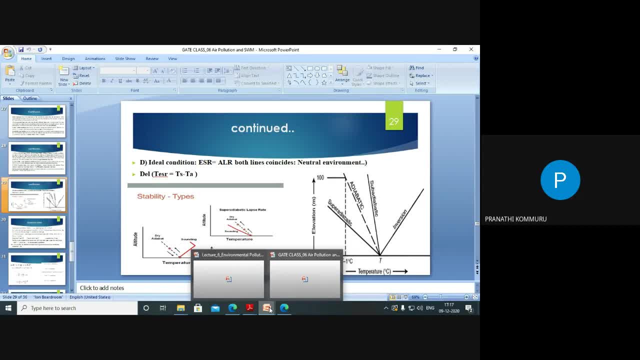 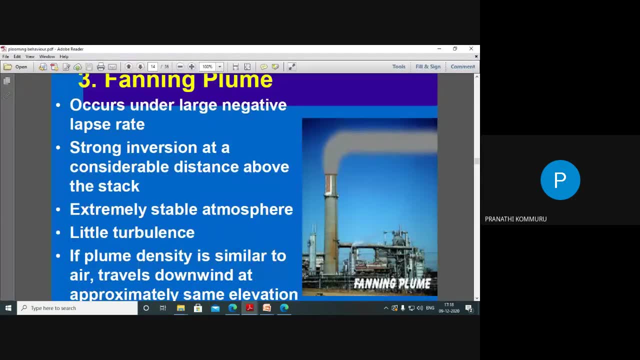 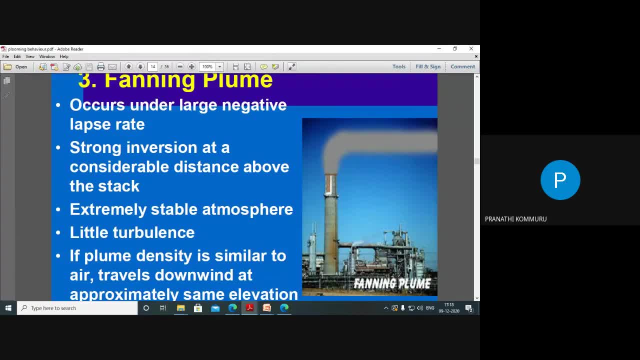 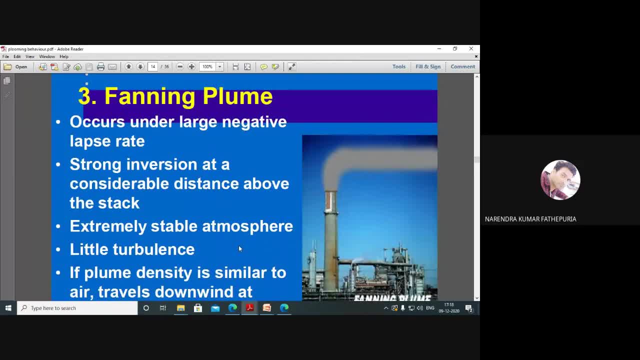 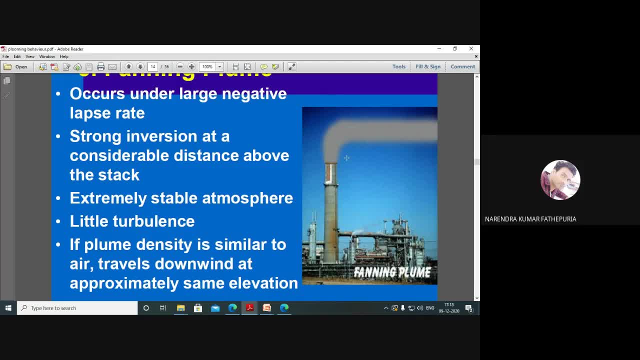 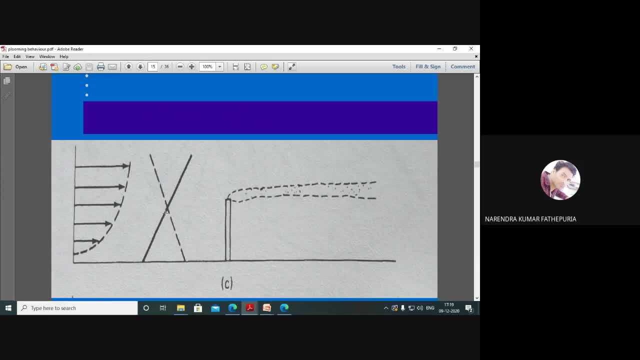 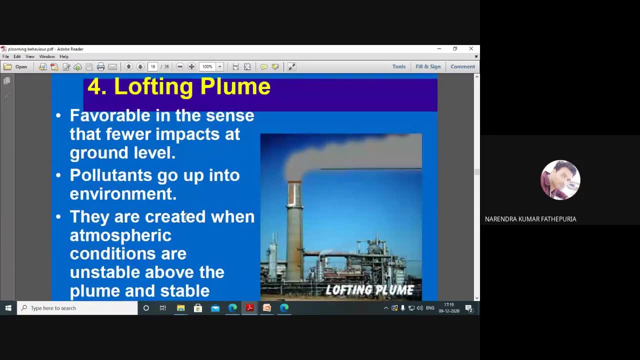 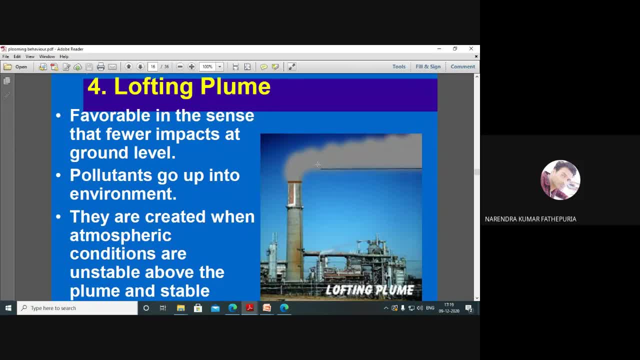 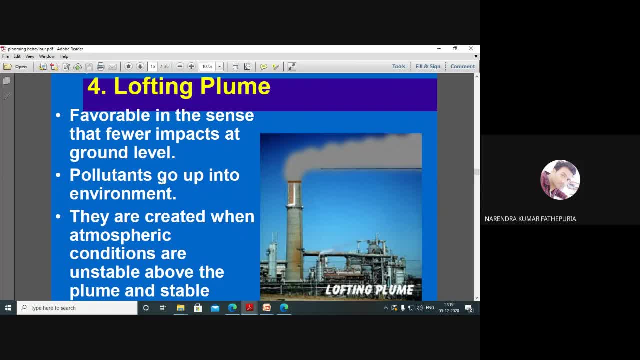 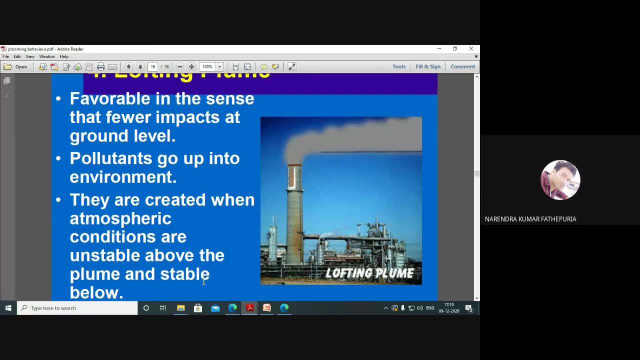 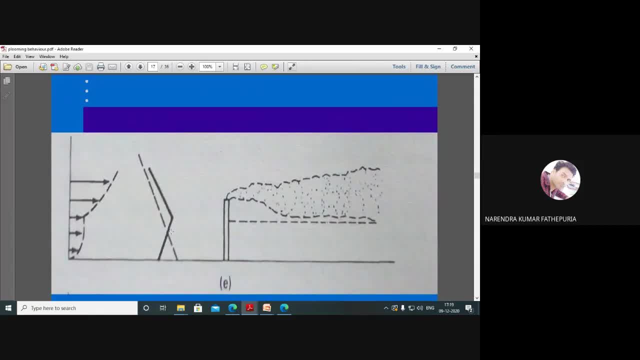 Thank you, Thank you. adiabatic left state in environmental depth it will. it will go like this: and and then finally it will be become up a approximate parallel to the adiabatic. it will be like this: from that part, this height, you escape it and you make a straight line over there. it will be a straight. 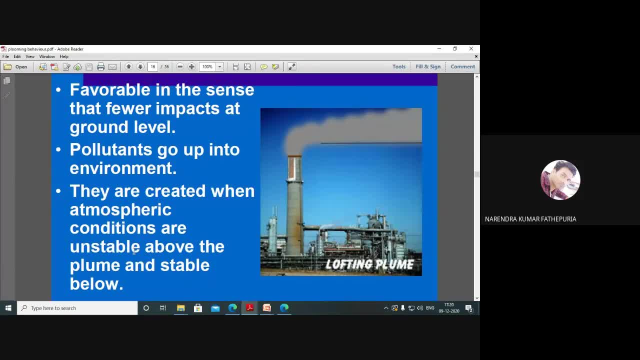 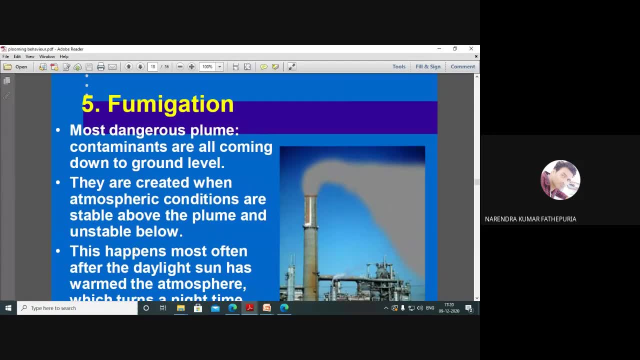 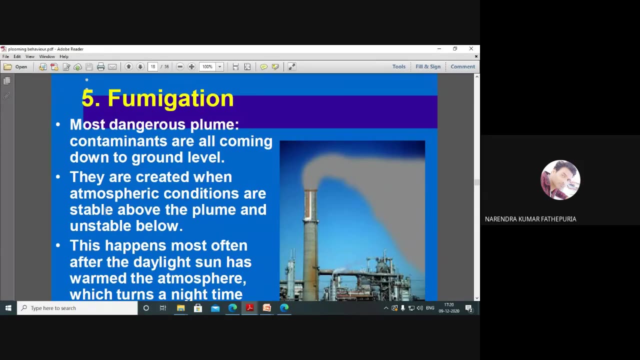 complete. this is an unstable condition. unstable conditions are good for the pollution dispersal, so that's good. this is generally the comparison. anything they can ask in the gated exam about all concepts, any, any concept, they are so which that you have to say seven, eight types. are there that? 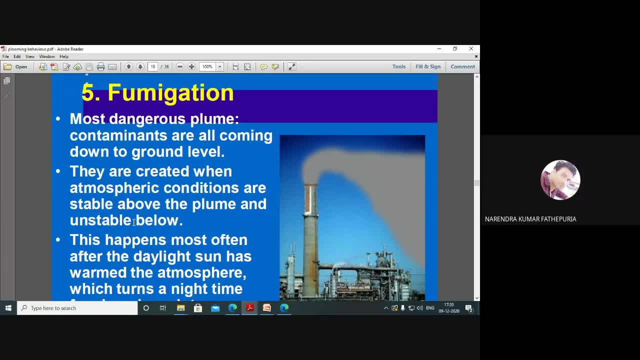 you have to understand which one is good, which method is stable, so they can ask the multiple select solutions, right, uh? highly unstable fumigation, highly unstable, good for the atmosphere, good for the environment, here also, yeah, now the combination of your the plume behavior as well as plume behavior with respect. 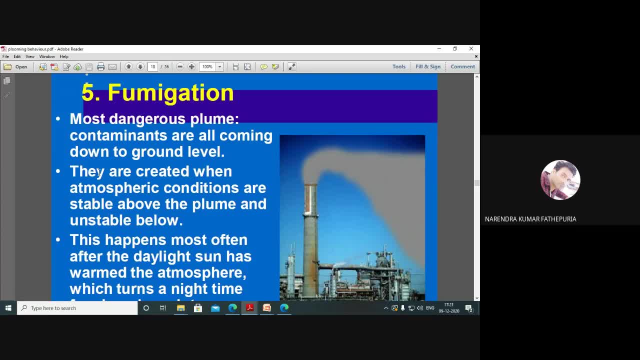 to esr, alr, as well as the alr that you have to compare. i i have one, uh, one slide where i have accumulated everything that is good for you, but i will come later. i will go later to understand everything. fumigation is most dangerous: plume, uh, contaminants are all coming down to the towards. 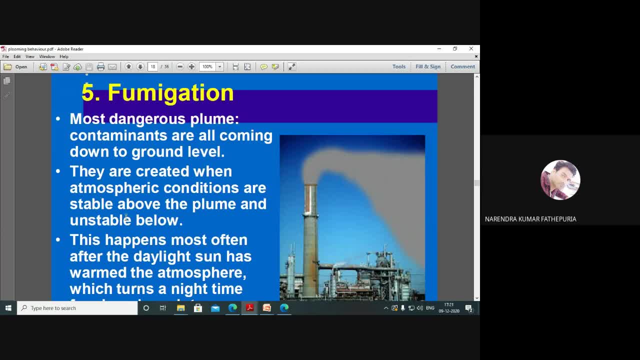 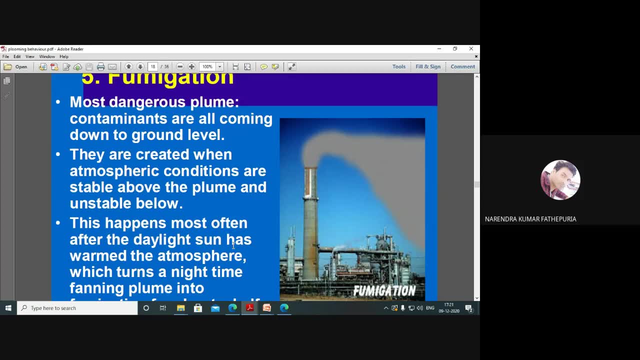 the ground. see, there they are created when atmospheric conditions are stable above the plume and unstable blow. this will happen most often after the daylight sun is. they are created when the atmospheric conditions are stable above the plume and unstable blow. above there is a stable condition, below there's an unstable condition. this happens most often of. 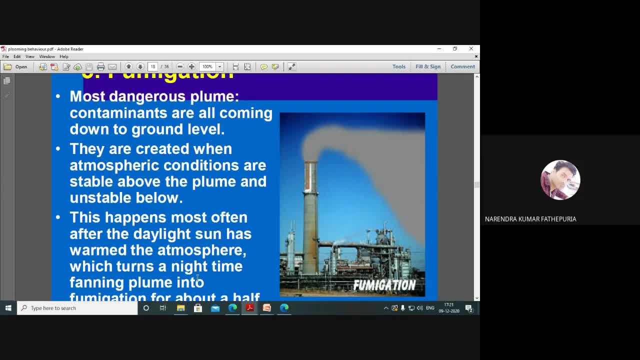 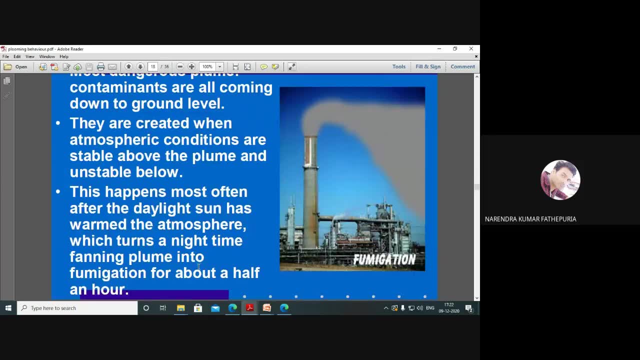 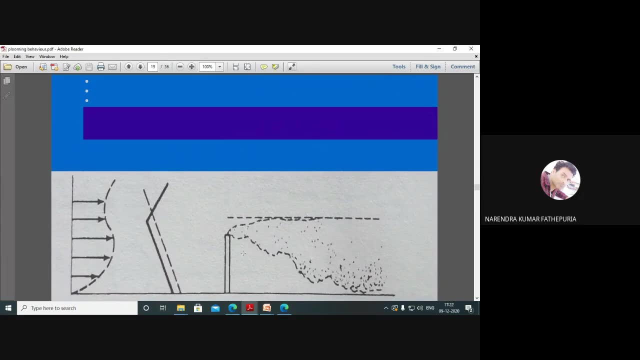 after the daylight, sun has warmed the atmosphere which turns a night time of fanning plume into the fumigation for about half an hour. So this is the condition for the, this is the condition for the, for this pollution dispersion. So the surrounding area, the, 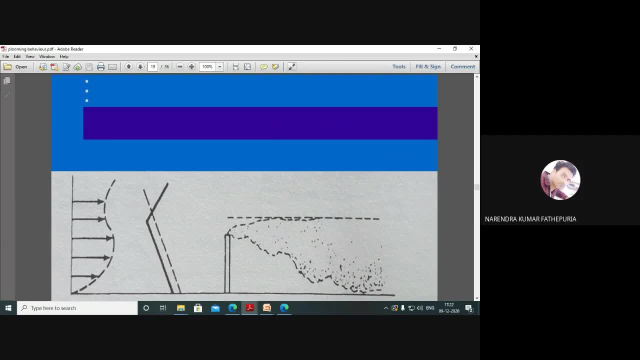 whole area. the pollution will be travelling towards the ground now, So it is not dispersing into the atmosphere, It is not going towards the stratosphere, It is going towards the ground only And it is not travelling at too much of distance. also, So the surrounding 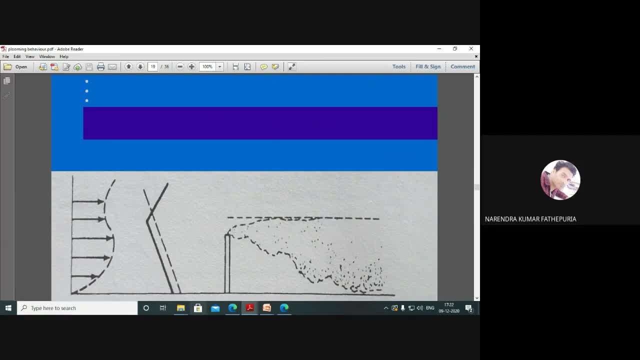 area surrounding. whatever the area is there, the whole kind of pollution will be dispersed into the atmosphere, into the, probably on the ground only. This is the condition here, Here: adiabatic lapse rate and environmental lapse rate. So dotted, we have considered: 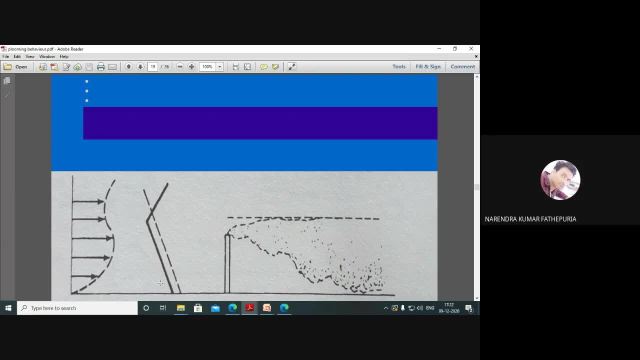 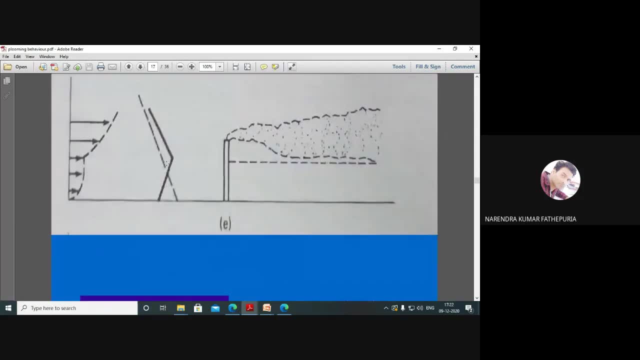 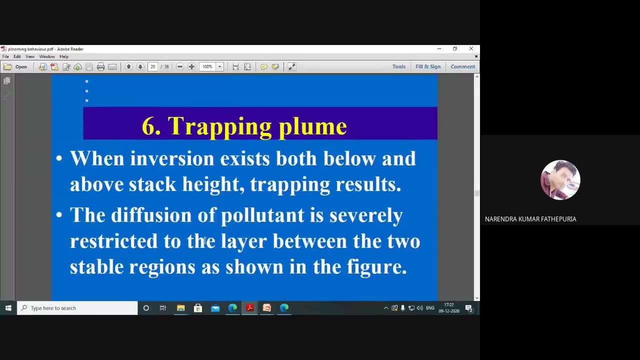 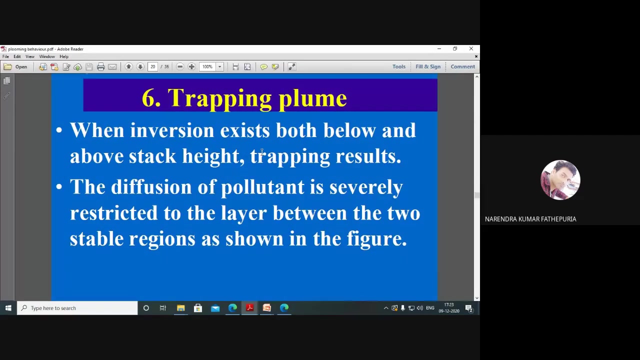 as the adiabatic lapse rate and this is the ESR. So this will be the relation for it. This graph will So do not get confused here Like this: What are the comparisons of that? Trapping plumes when inversion, both below and above the stake height: Trapping results. 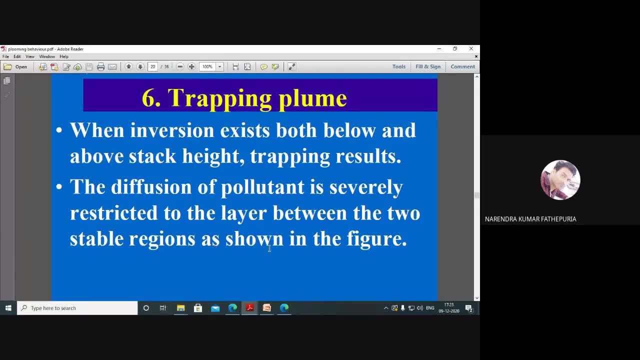 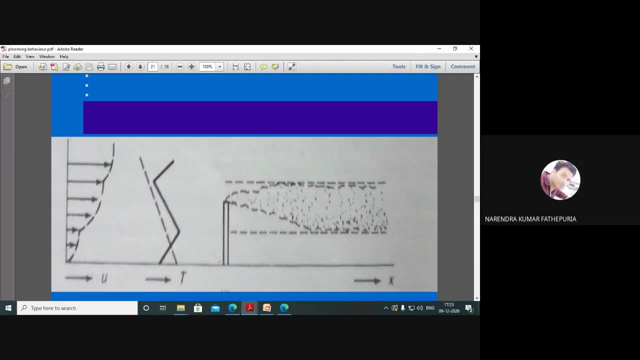 the diffusion of pollutant is severely restricted to the layer between the two stable regions, as shown in the figure See here. This is the one dotted line on the above of the pollutant, Below of the pollutant. This is the chimney from the air effluent is discharged. So 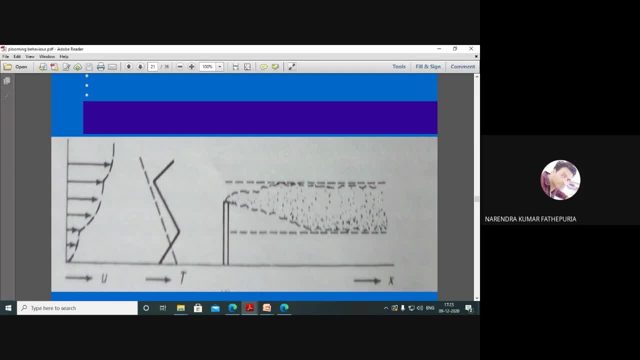 pollution is dispersed and it creates an inversion condition. It is kind of blocked here, It is kind of anti-cyclone inside. So it is very dangerous And the behaviour of ESR and ALR will be like this, Like this Environmental lapse rate with respect to time distance. 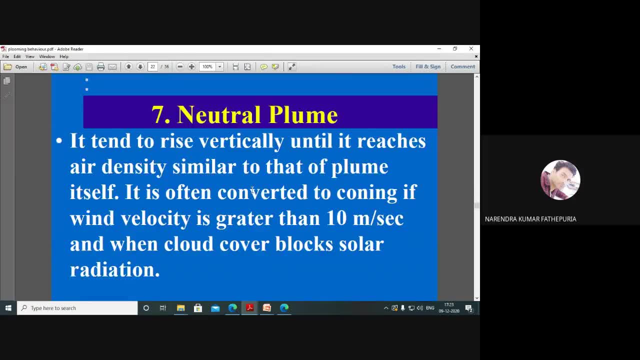 So this is the sixth condition for this. Then seventh is the neutral plumes. It tends to rise vertically until it reaches the air density similar to that of the plume itself. It is often converted to coming to conning if wind velocity is greater than 10 meter per second and when cloud overblocks solar. 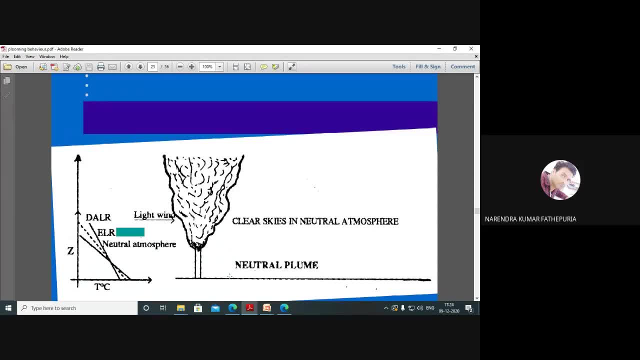 radiation. This is the condition for neutral plume, So altitude. with respect to temperature, This is neutral atmosphere, So environmental lapse rate and dry adiabatic lapse rate. So adiabatic lapse rate, The plume will be going towards the smoke will be going on the top. 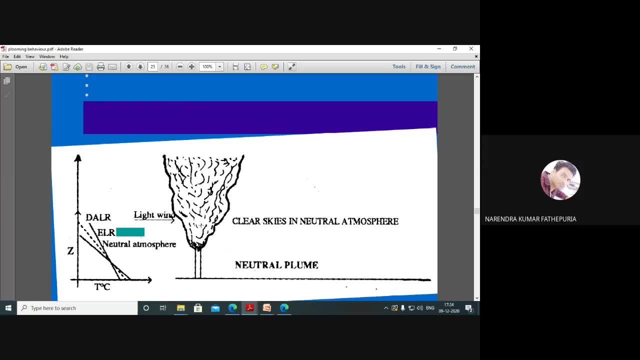 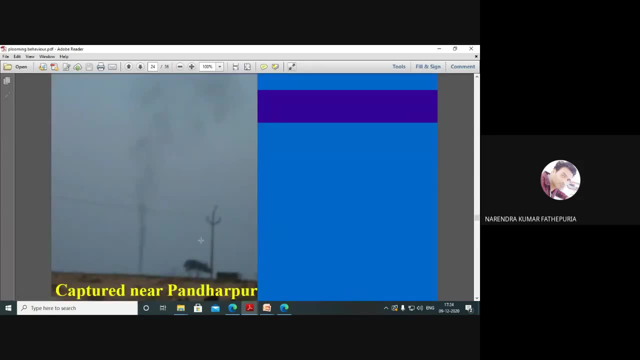 of the top. there only Light wind. Wind speed is low here, Clear skies and neutral atmosphere. So finally it will travel for this 13 height and it will disperse into the atmosphere. This is stable condition, Neutral condition. You see here, Captured near from the chimney. 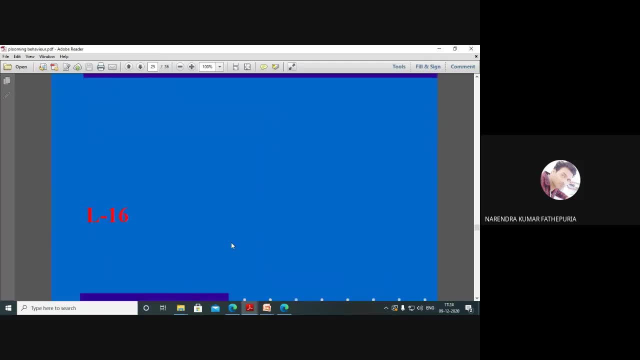 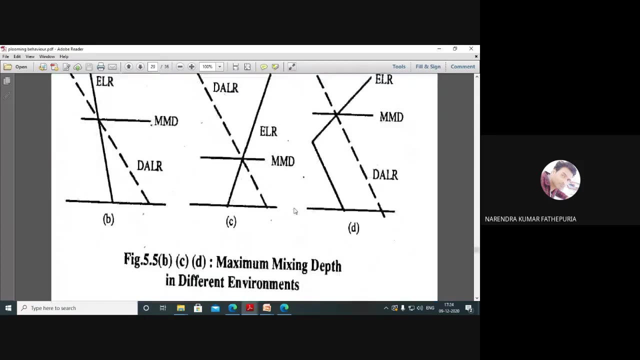 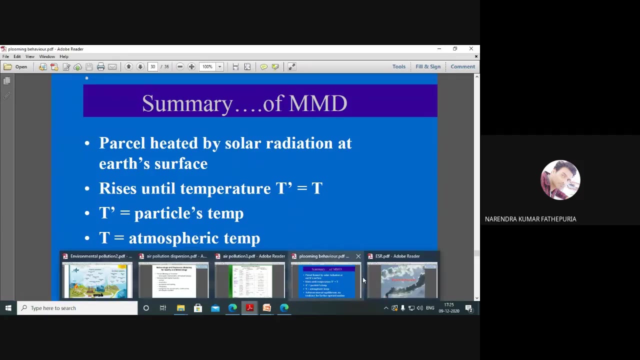 it is going up. only There is a maximum mixing depth and we don't have a time for this. You just find I will just send you this property. You just go through that, You will get an idea about it. So plume behavior: I have explained here also Various plumes, slopings and all that. 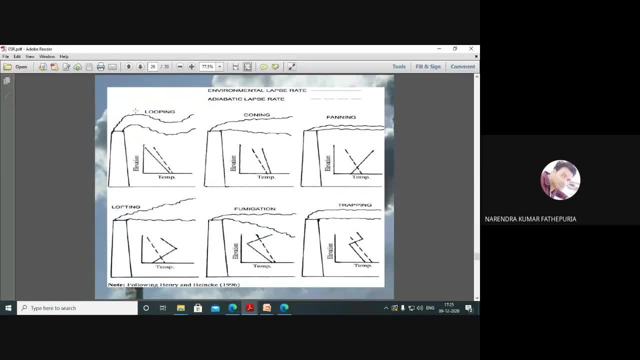 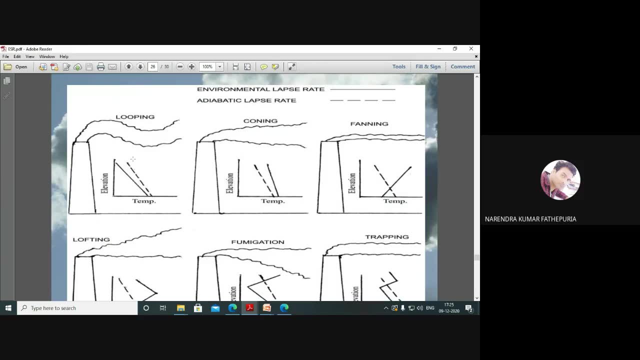 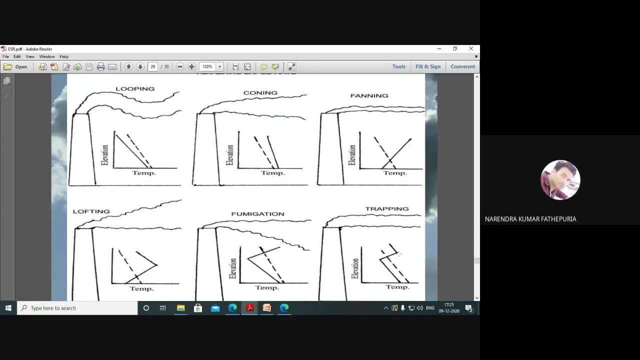 You see, here there is the comparison we have in the one slide. we have explained here everything. This is the elevation and temperature, This is the looping condition, This is the conning condition, This is the fanning condition, This is the lofting condition And this is the fumigation condition. This is the trapping condition. 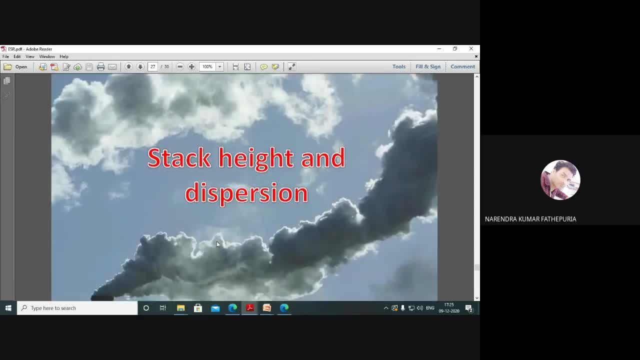 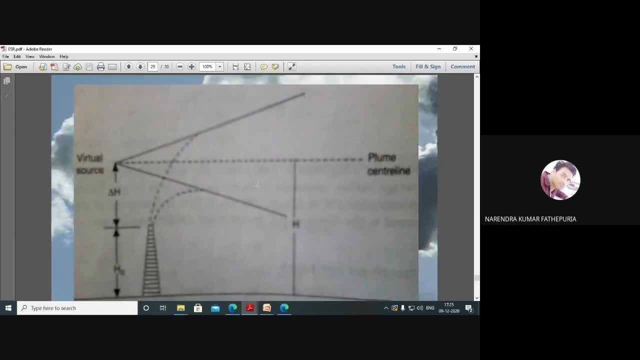 These conditions should be in your tips only Stake, height and dispersion. So that is the highly technical. You have to go for the various derivations and numericals. You have to do it. The plume concentration, plume center lines and all that. 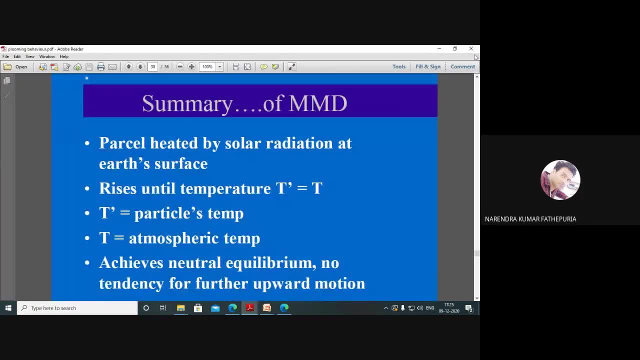 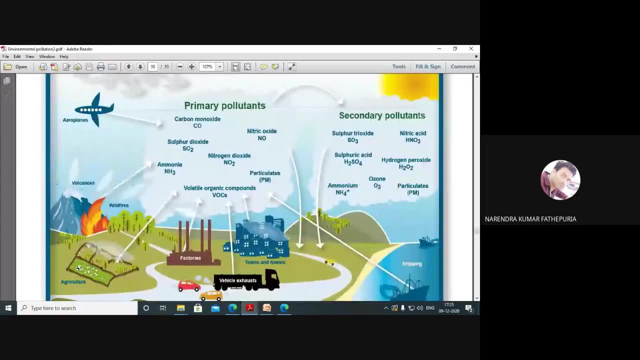 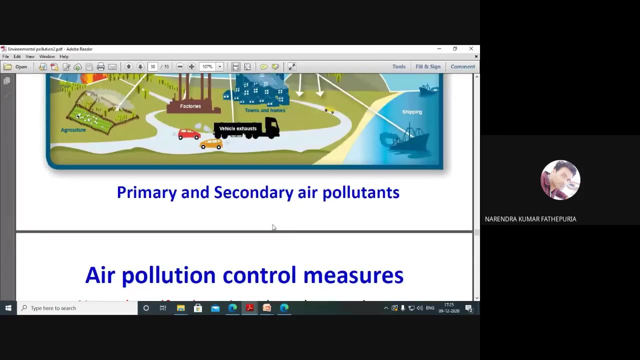 Okay, So that's all today. uh, we'll wind up the session, okay. um control and measurement part, i will take another five minute. that is also important. control in ways of employment, of pollution- we have studied everything that is also important. so, control and measurement part: there is a hierarchy for the environmental 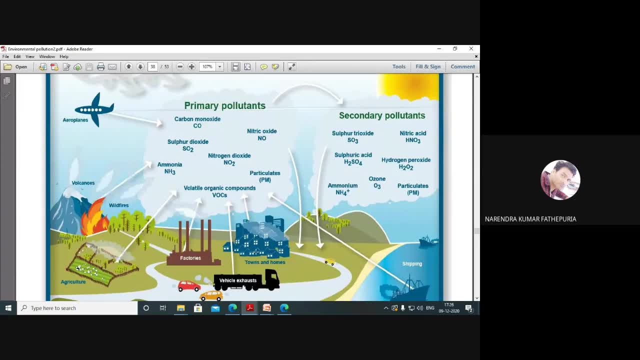 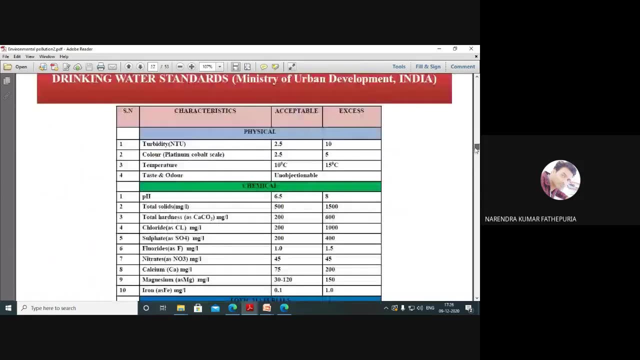 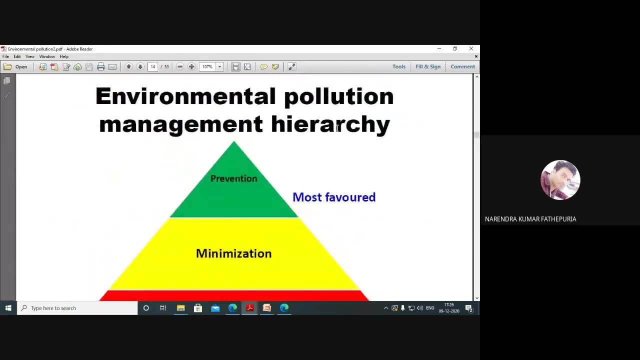 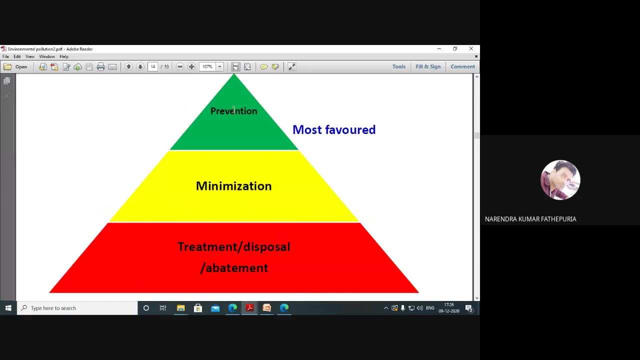 pollution control. environmental pollution control. um, the, the like the pyramid. no best payment. we have considered for the solid waste also the same way. we will be having a pyramid diagrams. this is like this: uh, yep, so this is the environmental pollution management hierarchy: prevention, minimization, treatment, disposal. and about abatement, we have always prepared. so first of all, 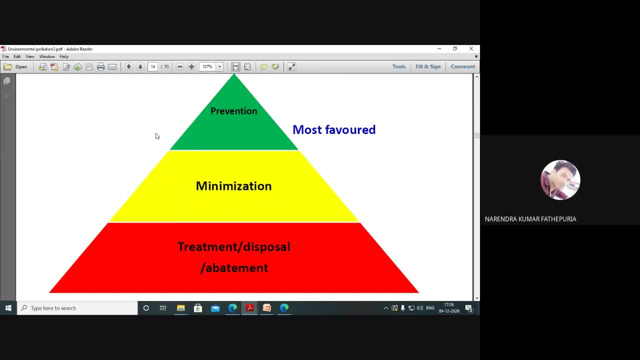 that we have to reduce the pollution at the source itself. we have to prevent the pollution at the source itself. suppose the pollution is releasing from the thermal power plant, uh, then you have to stop the pollution there itself by using the partial uh, partially or fully you are, if you use the more sustainable and biodegradable fuel. 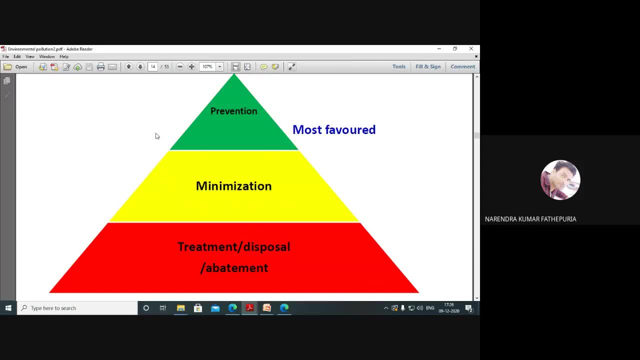 rather than using a coal. so if you replace coal, or or you just stop that coal plant and you go for the renewable energy sources, like solar, wind, wind power, wind power plant, hydro, hydro power plants- right, um, and you can go for the geothermal power plants- right, these are the more sustainable way. 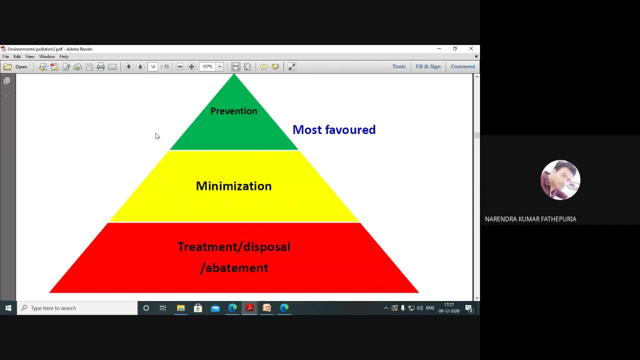 of energy generation rather than depend, being dependent on on thermal power plant and uh conventional sources of energy. you have to sift it into the renewable energy sources so that that we have prevented the pollution itself, because there is no coal burning and pollution will not be there for the emissions. 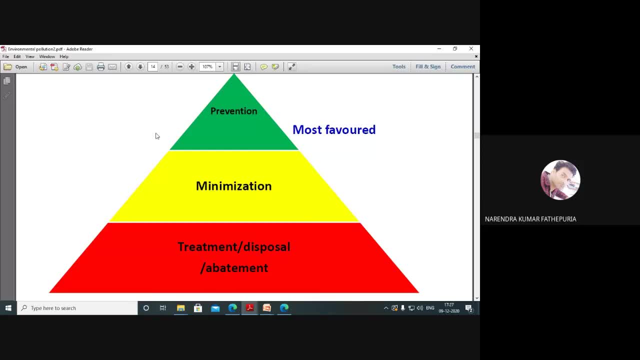 automobile vehicles what you will do, rather than being dependent completely on the automobile vehicle, the fossil fuel based emissions. we replace the fossil fuel by using electric cars, by using biofuels, by using biodiesels, by using bio cng cars- right so if you replace the fuel itself, so 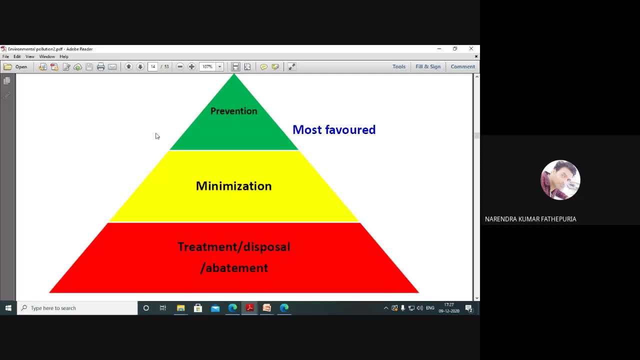 combustion will be not happening in the internal combustion engine, so of course the really then will not be. they told you then the the pollution will not come out from at all, from the source itself. so these are: the prevention is very effective, technique highly preferable, and then if the particular industry 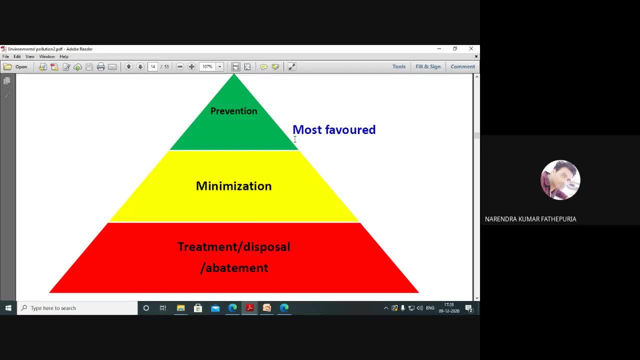 releasing a pollutant like the, like the um. There is automobile industries, manufacturing production sectors, steel manufacturing industries. You have to partially, or at least 50%, you have to replace by the SDF and RDF fuel. So SDF and RDF fuel are more renewable, more sustainable. 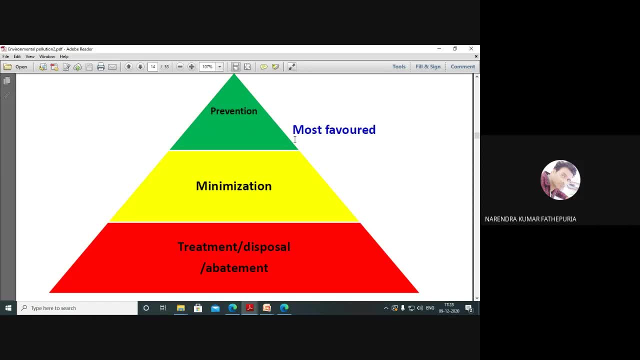 Then we can prevent the pollution And construction also and building in urbanization and building transport, whatever the things you are doing, it And construction things also, you can use a more sustainable material. So more sustainable material, if you are using it, then it is good for the environment. 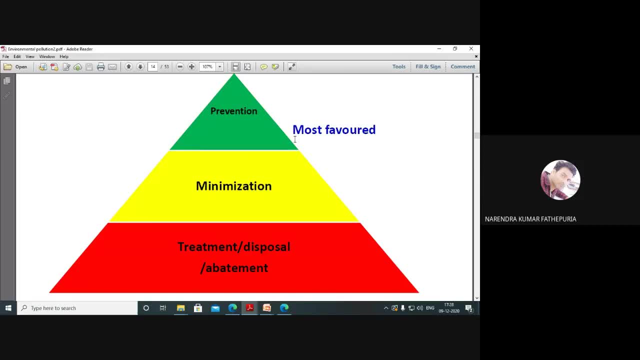 And the third thing is reusable. not reusable the transport, like road transport, rail transport and gear transport, Everywhere you are using fossil fuel, that you have to stop it and that you have to use more renewable energy source. Yeah, fossil fuel should not be used. 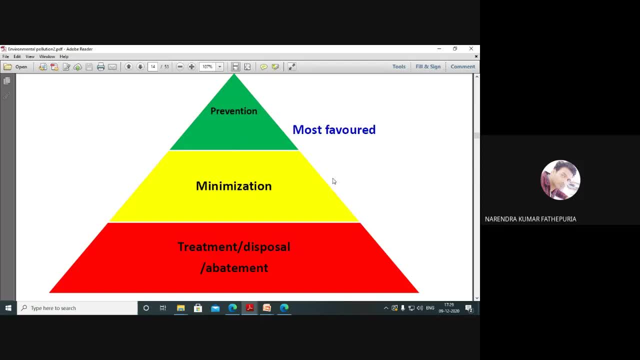 So another thing: prevention, after that minimization. If you can't prevent completely, then you have to minimize it. Minimize it means partial replacement of the fuel by using more sustainable fuel and all that right, Biofuel, biodiesel. Other thing: using the public transport rather than using the private transport, always right. 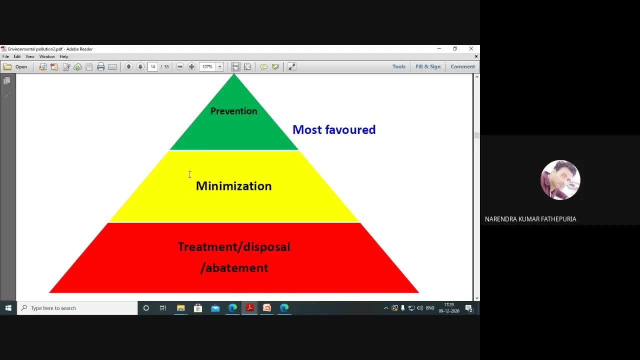 That personal vehicle should not use that much. And then public transport- we have to use it right. And Five minutes, Okay, okay, okay. So minimization is a very good practice technique If you minimize the air pollution by doing various preventions. And agriculture also. So if you are using the pesticides and insecticides, if you use it less, then also environmental pollution can be reduced. Open burning should be stopped in open dumping side of municipal solid waste as well as in the open burning should be stopped in the residue left in the agriculture farm. 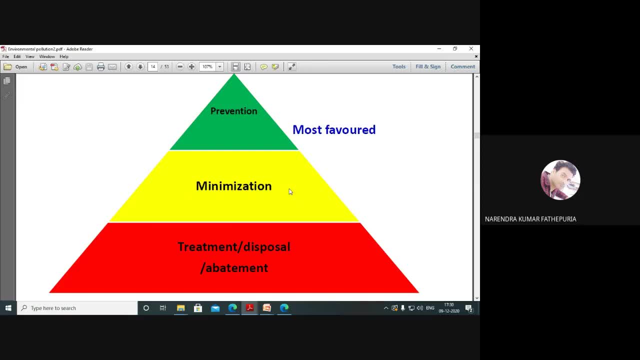 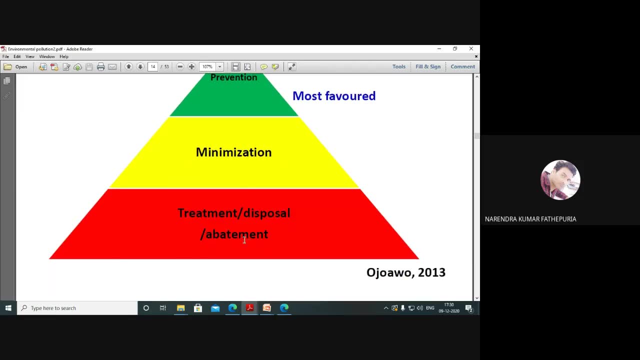 That also can stop the pollution at any cost. right? These are the various techniques that we can do it Now. if you can't do anything, then the treatment. that is the main effective technique that if pollution is coming that you cannot stop it. 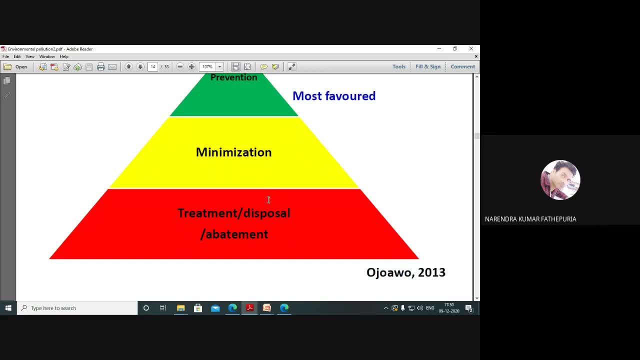 Then you have to treat it. For treatment part, you have to use various. as I told you, there's indoor air pollution, outdoor air pollution. For controlling the indoor air pollution you have to go for air purifiers and all that right. 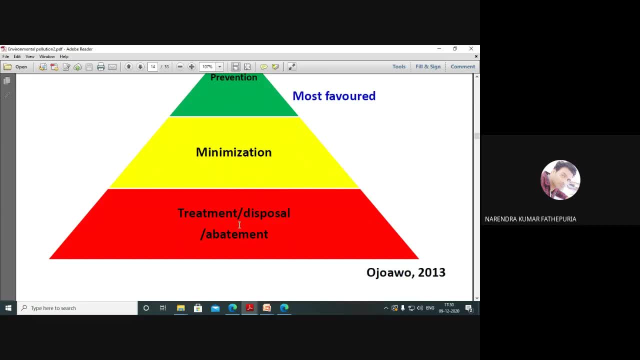 For outdoor pollution also. nowadays you can put a big, big air purifier tower so that way we can minimize the air pollution right. Once you identify the air pollution is coming because of this, only then you can control it. And then treatment and abatement part, various engineering devices you can use it. 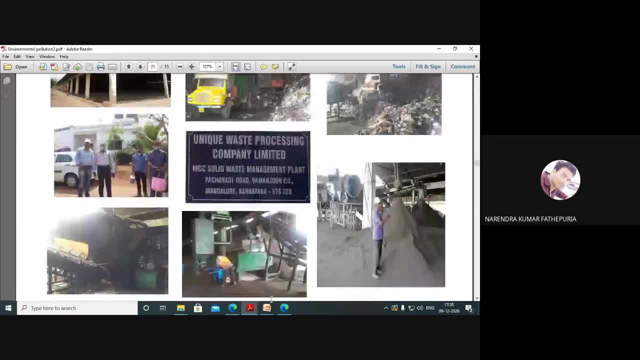 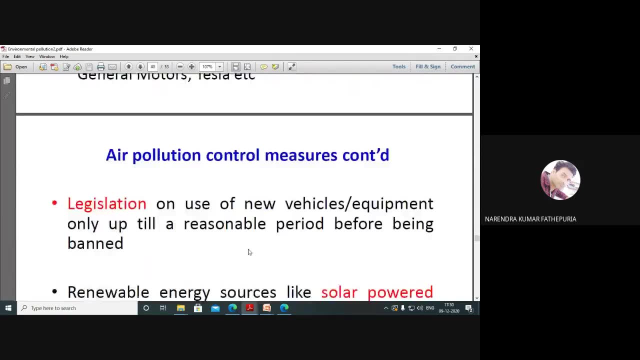 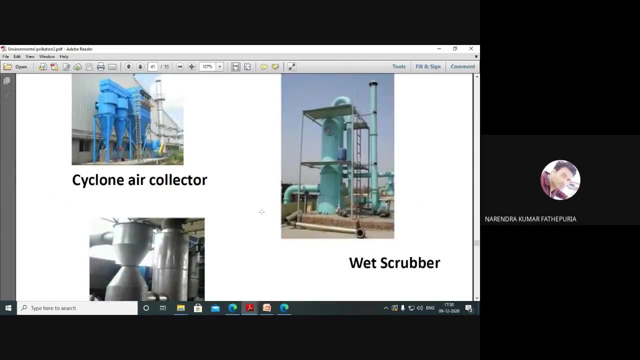 For controlling the air pollution, like electrostatic precipitator. type: electrostatic precipitator, wet scrubber, mechanical scrubber. right, These are the engineering devices that you can use for controlling the pollution. Here it is: There's a cyclone air separator, cyclone air collector- wet scrubber- wet scrubber and cyclone dust collector. type: electrostatic precipitator. 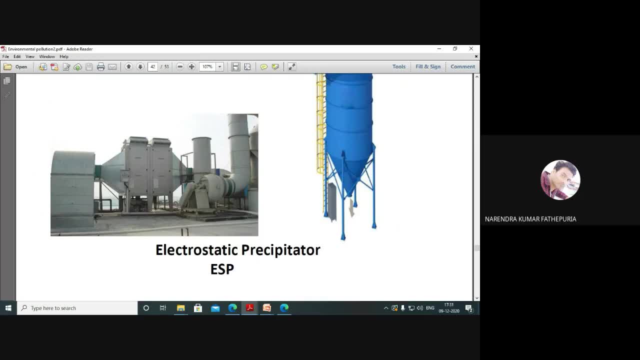 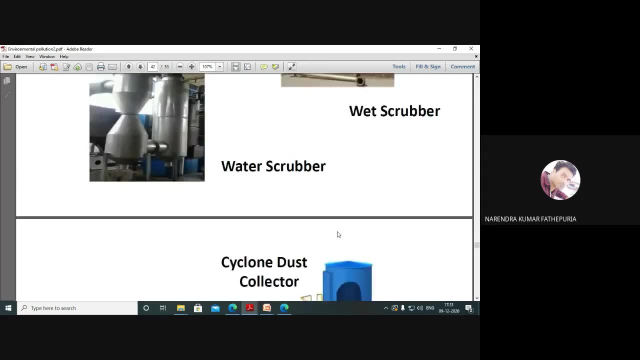 These are the air control pollution residue devices which has to be incorporated in the industries Which are responsible for relieving the pollutions right. So these are the. the pollution can be can be controlled from the industry, from the industry part. 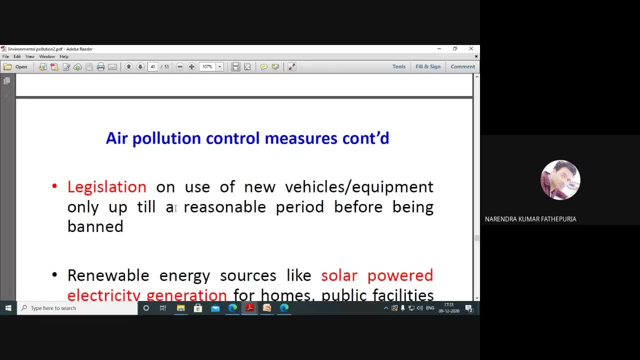 Legislations. the rules and regulations should be very strict and the government has to make the guidelines clearly. They should put the penalties. pollution control board has to do the audit regularly, regular basis for the various industries. while giving the environmental clearances Public, we can say the contribution is very important. 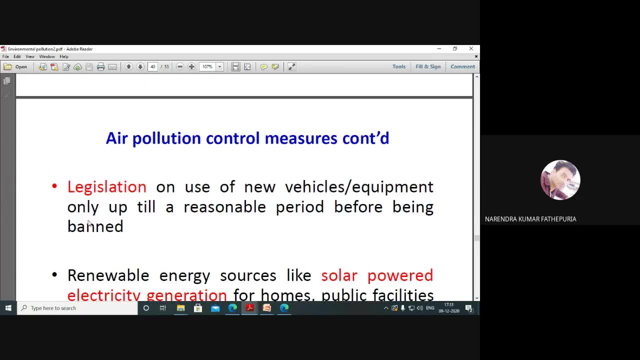 So you can do the audit regularly, regular basis for the various industries. while giving the environmental clearances Public, we can say the contribution is very important. The public is to be very aware of the pollution part and to always protect our, our, our atmosphere. 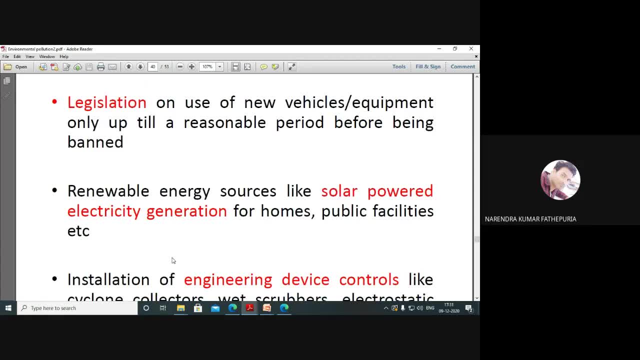 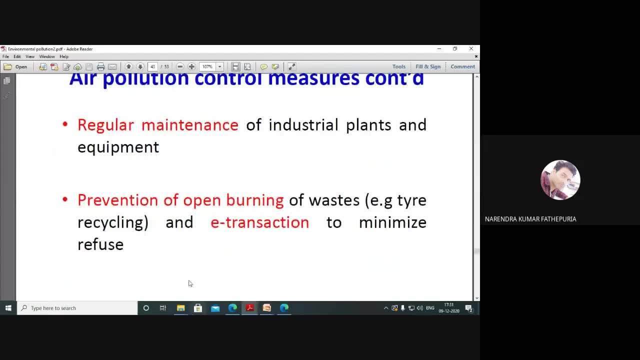 More plantation is required, right, Renewable energy sources are uses, as I told you. right, These are the some things that we can do with for controlling the pollution and before that, as I told you, the waste management is always important regulations, and this is always important. 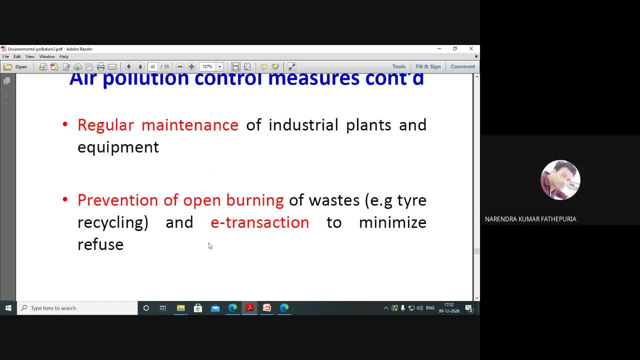 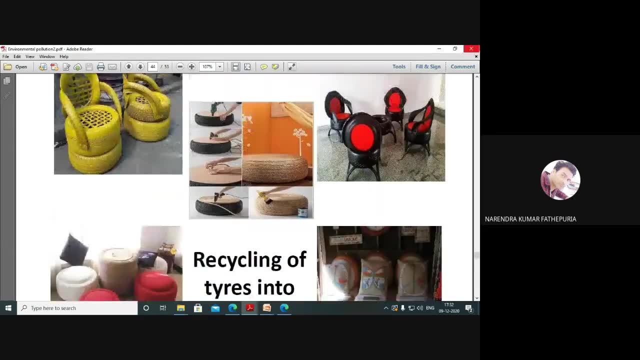 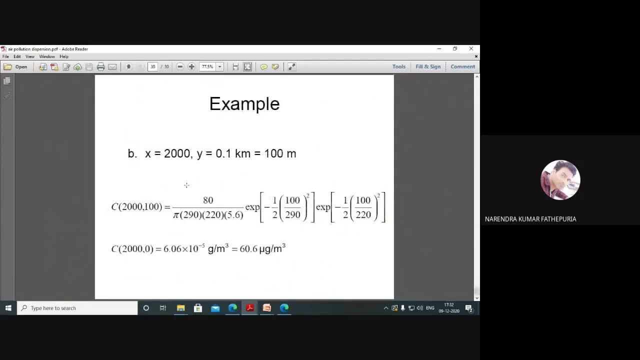 Regular maintenance of industrial setups and plants can also be done. Prevention of open burning, based any e-transaction to minimize the refuse right is the various things that we can do for controlling the air pollution part. okay, so these material I will circulate in their Google classroom. I just download that and study quickly. 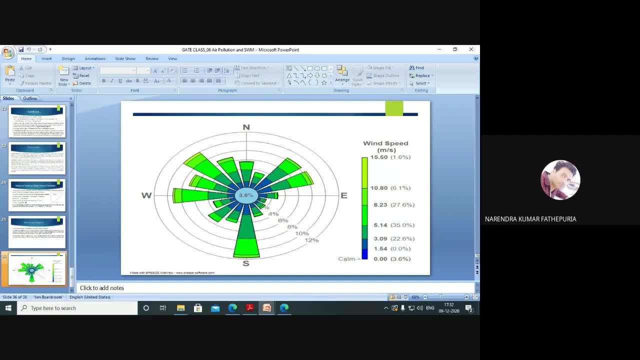 and then write your exam in the West for the great exam. so by this note I will just bind up the session for today. thanks for the CMR, IT management, as well as Nick Mercer and those every given our portion, this classes and we have. we are here in the king. okay, for this year it is fine. for the next day: okay. 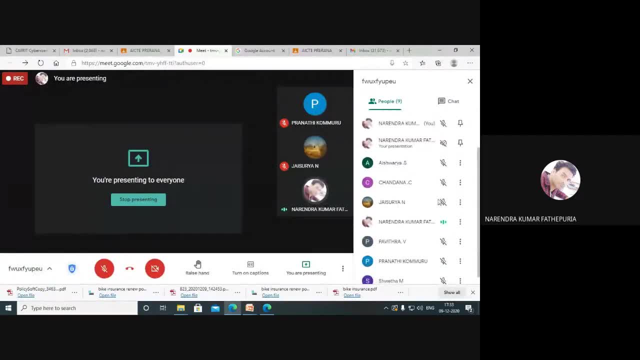 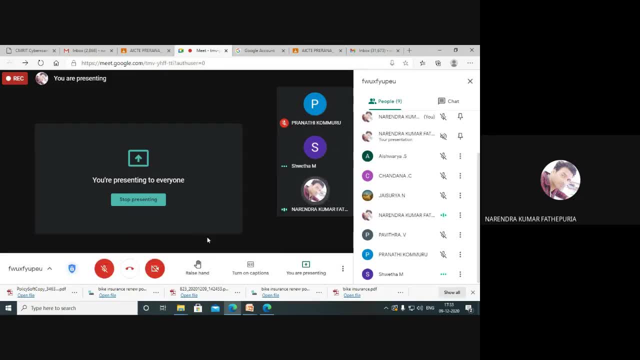 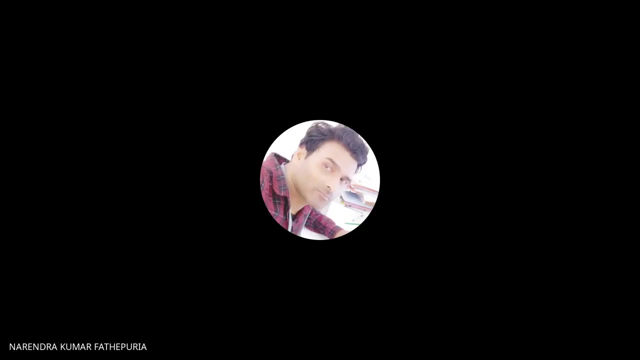